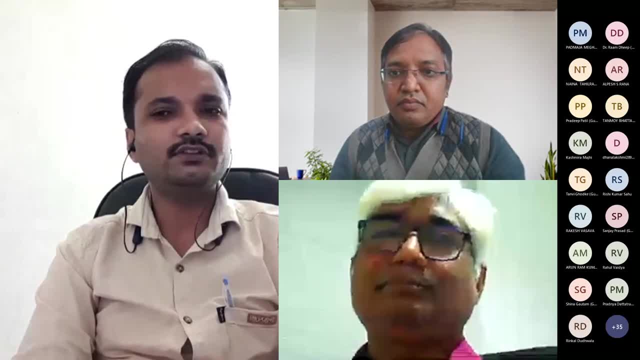 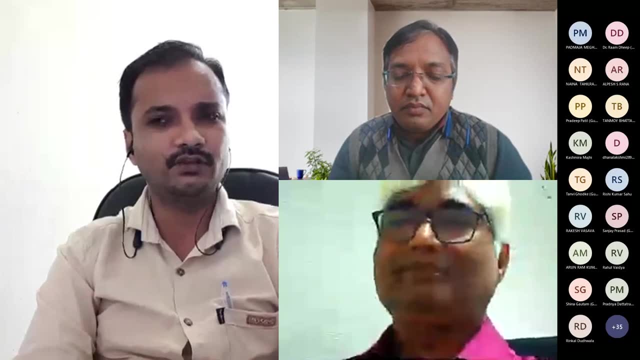 Indian Society for Technical Education, the Indian Science Congress Association, Material Research Society of India and the Indian Society for Technical Education. He is a representative of the Indian Association for Technology, the Indian Association for Technology, Indian Dissemination Association, Electron Microscopy Society of India and Indian Institute of Chemical. 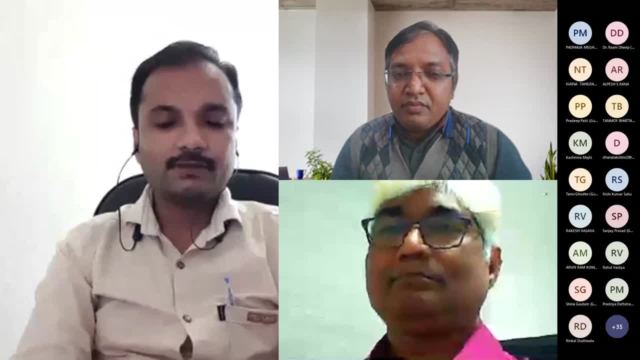 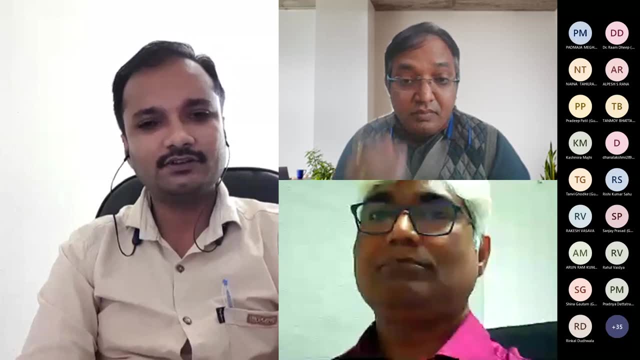 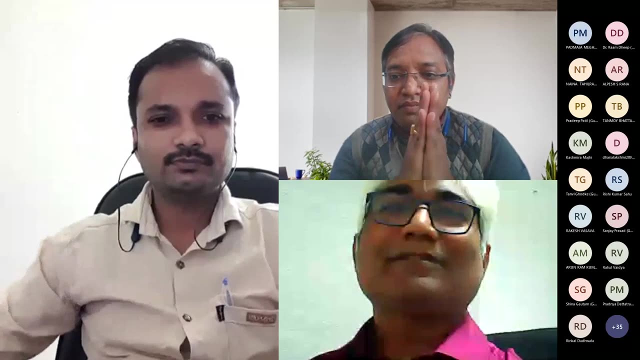 Engineers The Chemical Engineering Department, Government Engineering College Baruch welcomes you, sir. Now I request Dr V N Lad sir to take the charge of the session. sir, please Thank you very much, Professor Rohit Mr Rajiv, for nice introduction. 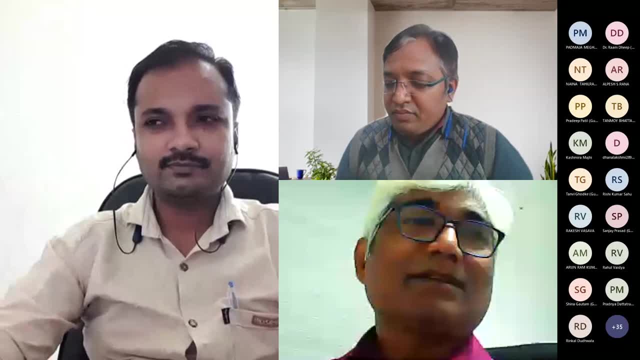 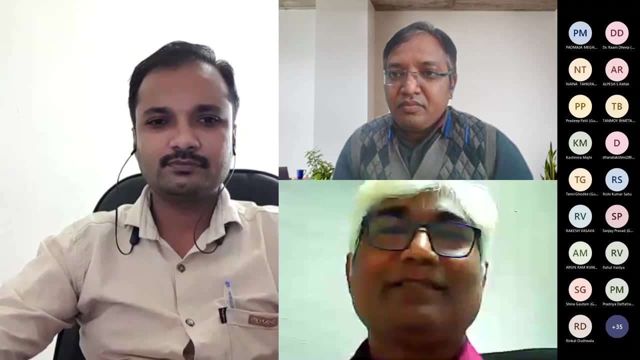 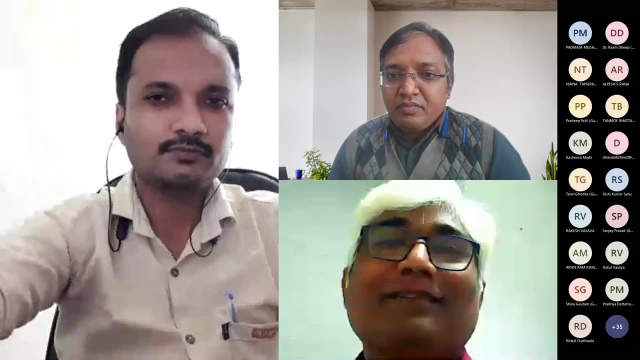 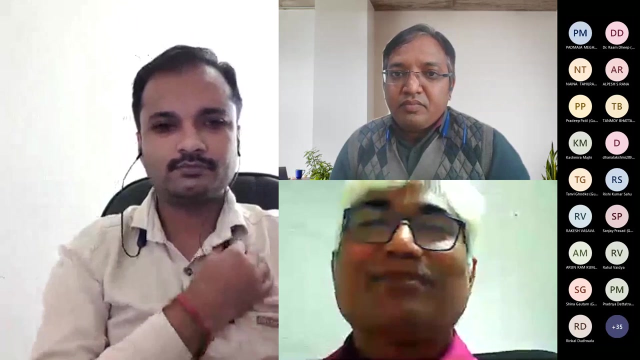 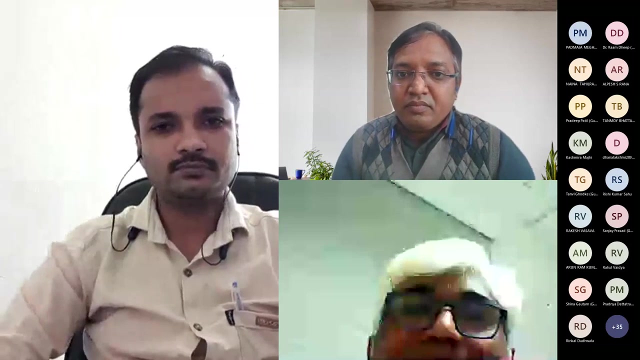 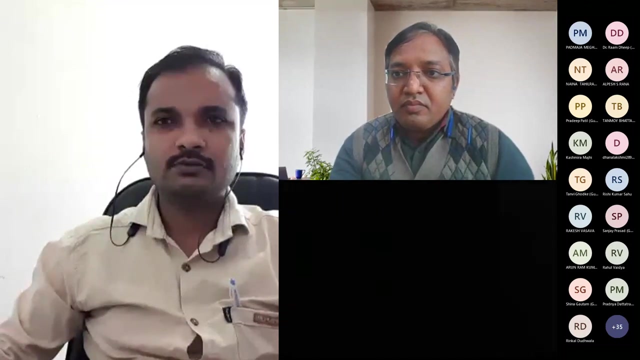 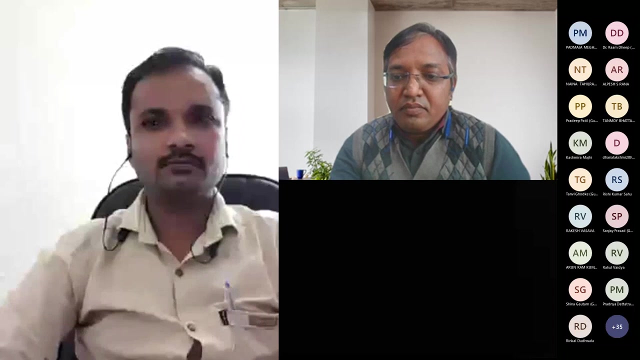 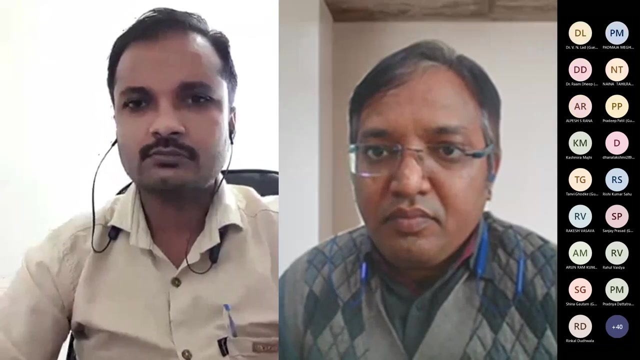 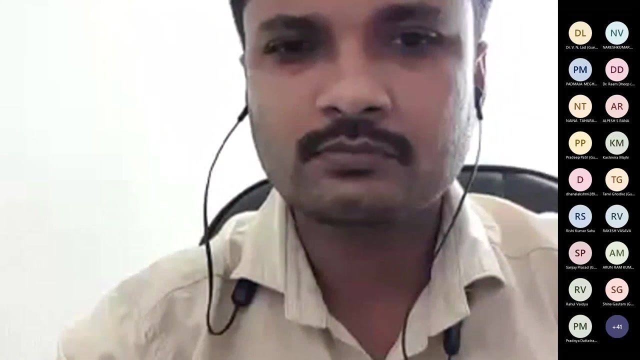 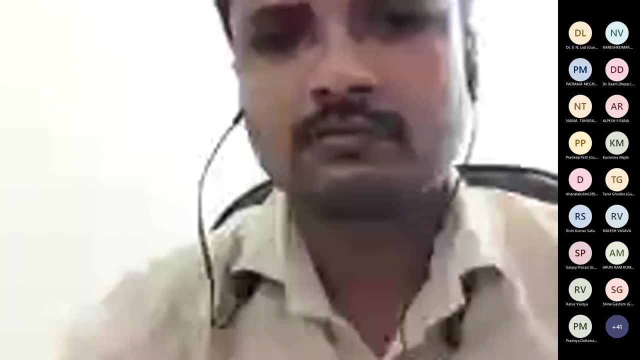 Thank you again to Professor V N Lad for inviting me to deliver this lecture. Thank you so much for giving me this opportunity to share my views on this particular topic in your FTP, So I'm sharing my screen now. Thank you, So my screen is visible to you. 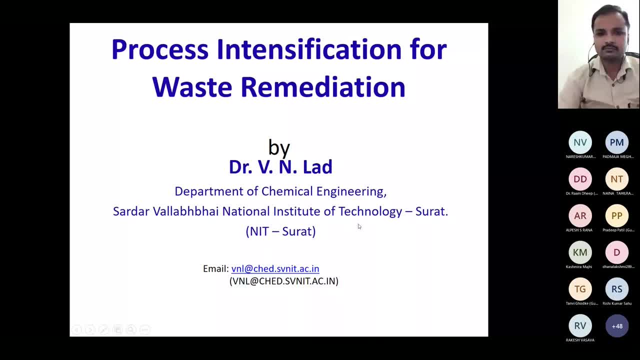 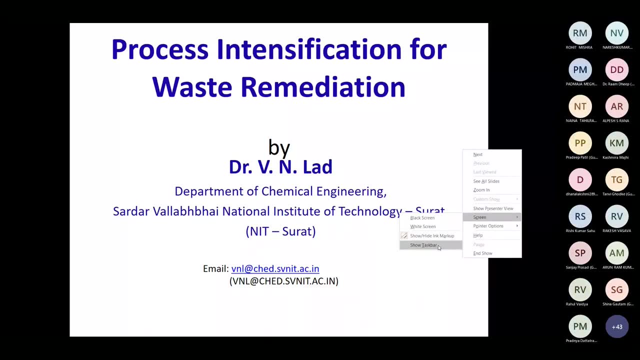 Yes, sir, Screen is visible, So thank you once again. Again, my name is Dr V N Lad and I'm here to deliver this lecture. Thank you very much, Professor V N Lad, for giving me this opportunity to share my views on this particular topic in your FTP. 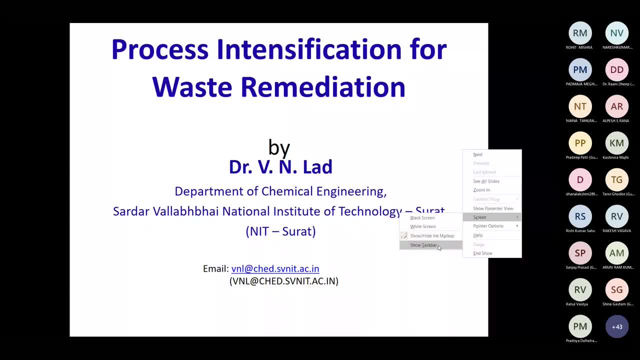 Thank you very much, Professor V N Lad, for giving me this opportunity to share my views on this particular topic in your FTP. Thank you very much, Professor V N Lad, for giving me this opportunity to share my views on this particular topic in your FTP. 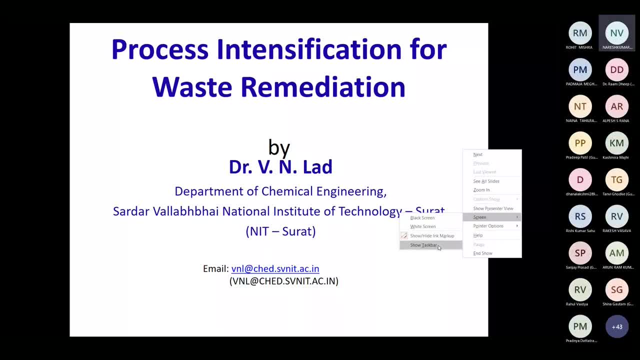 Thank you. Thank you very much. So I am going to speak something about one just for preliminary mention: Res verification. So it's a Come up And so mine. Look at the document. This isaso Someone's Name. Looking Cuz Yeah. 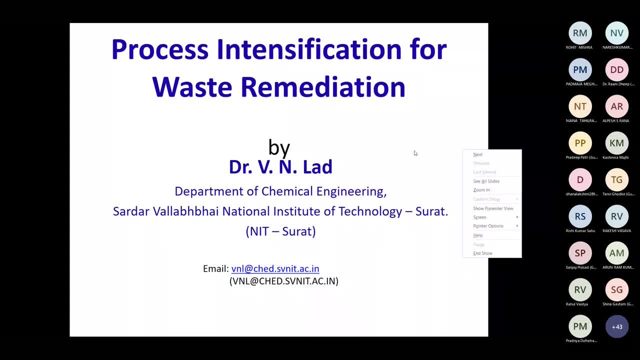 I'm not sure about this thing. Come up Shouldn't Background the difference between the base management based remediation and the zero discharge. so not going into that particular thing directly, we will focus mainly on the process intensification in the initial uh during all the times, and later on we will shift. how can we implement this? 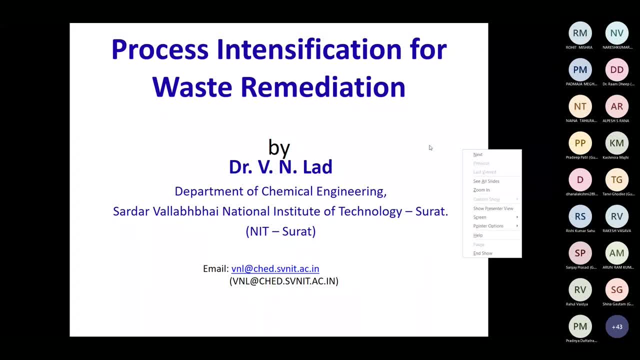 fundamental concept of the process intensification for waste remediation. so, uh, the main logic behind this, the process intensification, is that interesting. like always, we want to produce more amount of product, quantity wise, very good quality of the final product. so we want to have all this good quantity, more quantity with good quality, extra pure. 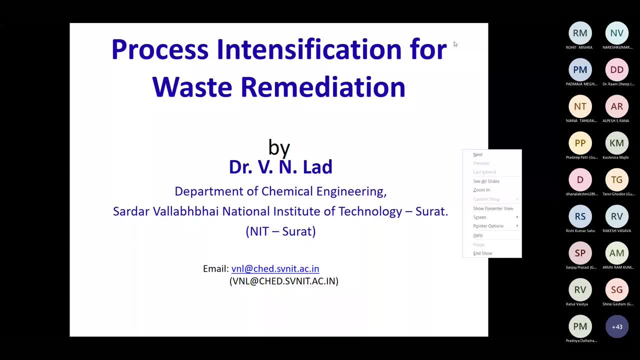 quality of the final product and also in with the limited energy consumptions, or at the low cost, or at the low uh resources, uh or so the in order to produce that quality product in a very good, with enough quantity, in a timely position to market, is the main focus of the process. 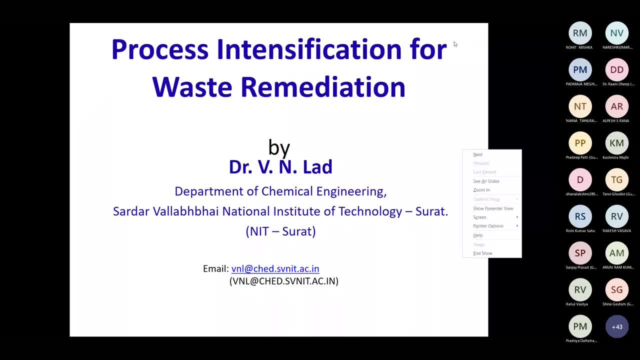 intensification. so basically this uh, intensification means if you want to produce an imperial, any product, or if you want to have pom-poms providing the service, then what kind of intensity can we need to carry out in our conventional plants or conventional process or at the? what are the necessary steps in order to achieve that? 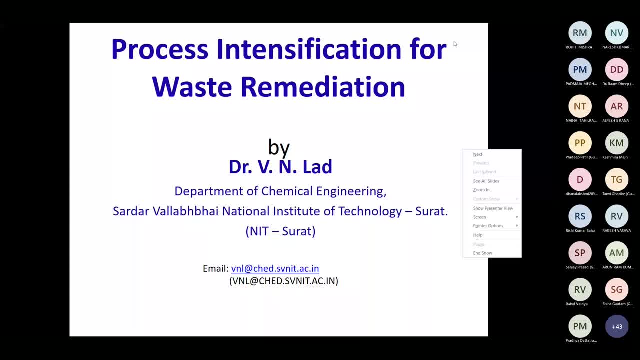 particular goal for is all included in this intensification of the process. now, how to implement all these fundamental things, uh, in order to have the waste remediation. so the basic things related to this intensification are the basic things related to the waste remediation. so the basic things related to this. 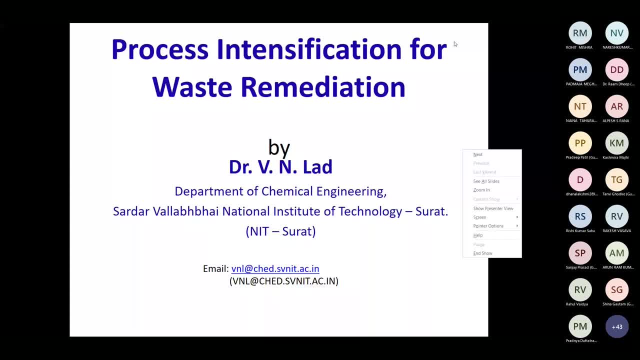 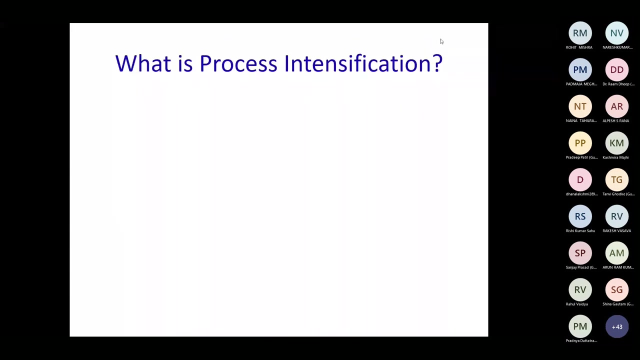 intensification is the how to minimize the waste, how to minimize the hazardous effects of the fish, or, and in order to achieve this thing, what are the main changes we need to carry out in order to have some set of the conventional process? so, uh, so, so This will be the next slide. 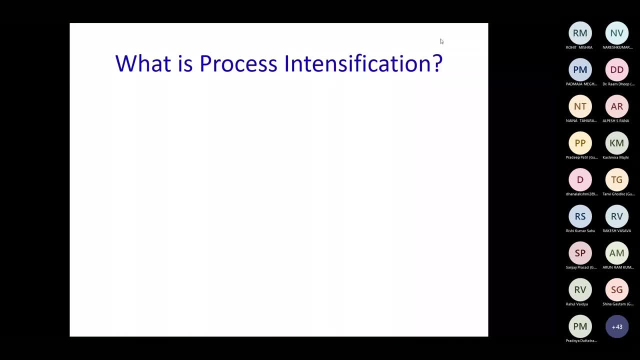 so this is the process of the process intensification. so this is the process of the process intensification. the process intensification is so that is what is known as the process intensification. so ultimately, the result of the process intensification is good quality product, much more quantity, which can be available in a limited time. 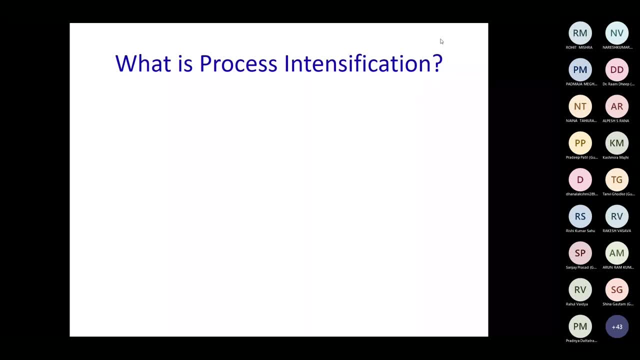 that is also one of the aspects of this process: intensification. and so what are the basic things? see, if you want to produce any, any product like, if you are having some reaction like A plus B gives C plus B, then there are some constraints, like the rate, constant kinetics. 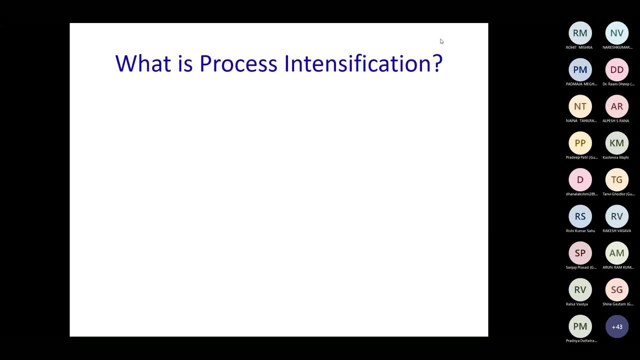 of that particular chemical reaction, which will limit our effort in certain ways. so what are there in the hand of the designer of that process or the processing plant, what are the flexibility or the resources available with the designer and accordingly, we need to work on that with the teams in order to achieve the desired results. 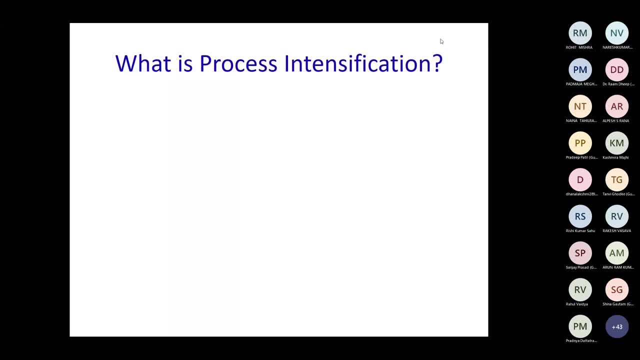 So in this case, it is the design goals of the intensified process flow. So using MINPS, ultimately, this intensification will ultimately result in a drastic change in the process, which will ultimately result in a significant advantage in terms of energy. 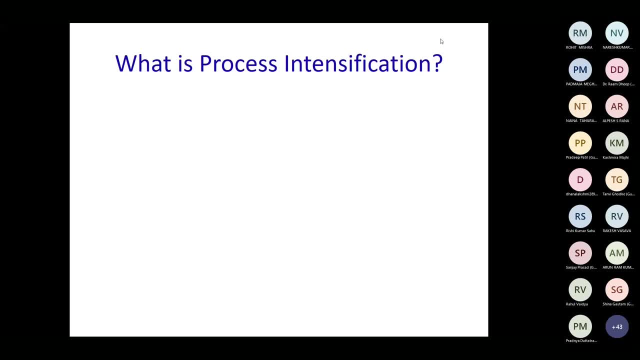 in terms of cost, in terms of product quality, in terms of the quantity, but when we talk that, in case of waste remediation, it will ultimately lead to the minimization of the quantity of the waste or the minimization of the toxicity, hazardous properties or the 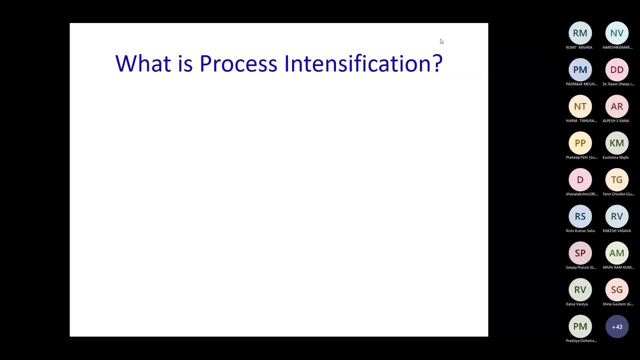 hazardous characteristics of that waste product which is coming out from that affluent treatment plant or the industry. So initially, if you want to intensify an existing process, you can start in the existing traditional process, conventional process, which is available at our plant site, And before reaching that, any gas liquid or that multiple stream. 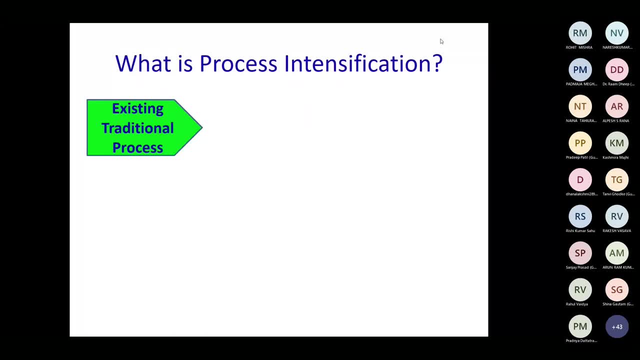 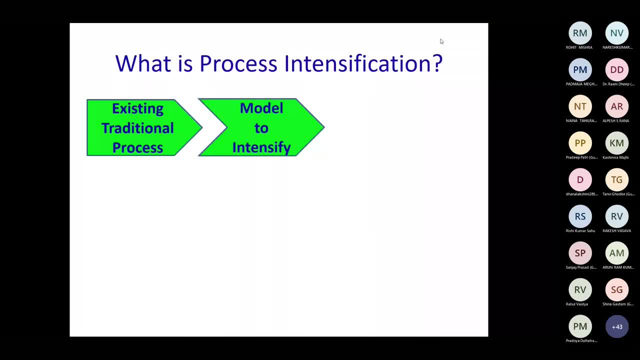 steps with that conventional process. So initially we need to model how to intensify that existing process. Now this model may be of several types, like including some physical models, some pilot plant studies, laboratory scale studies, as well as some mathematical. 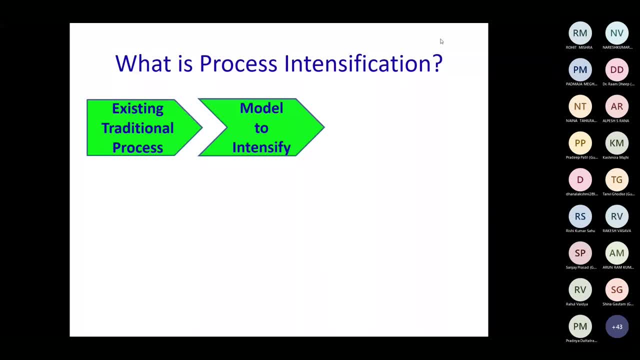 modeling nowadays also provide a very efficient tool in order to have that proper identification of the process. so uh, later on it comes to that. how to implement that model in order to have that physical process, so uh, how to implement that model is again require some input from the existing environment, like if 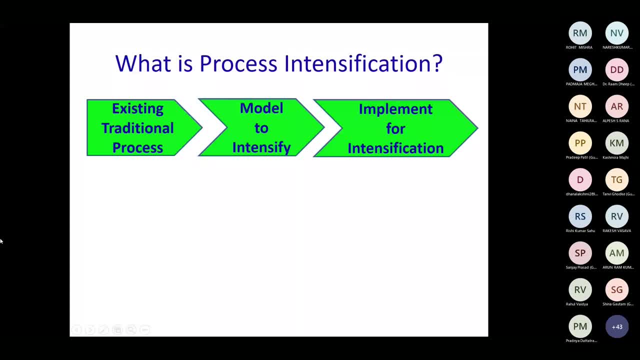 you want to treat that, your acidity based in your neutralization stream, what are the resources available or what are the other alkaline streams available from your own plant and according to that, we need to work out on those kind of resources. another example, uh, like if you want to. 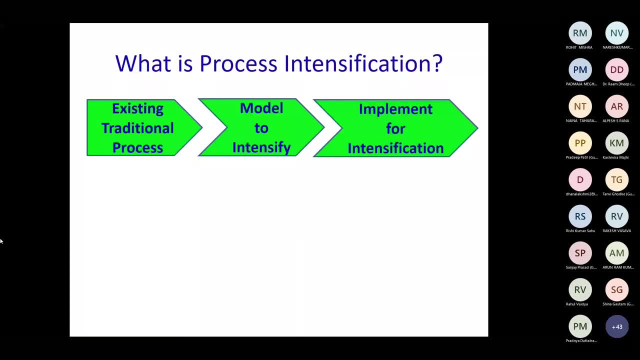 locate your effluent treatment plant in certain area of your entire plant site, what is that connectivity of with other processing plants or processing equipment which are delivering that stream, which are going directly to that effluent treatment? so the overall fighting system, as well as some intermediate holder tanks and even the sequence. 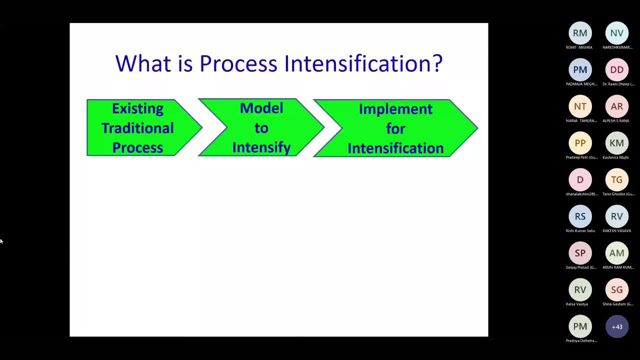 of all the main reactors, as well as other separating treatments, need to be reconsidered in this particular stage, while implementing, uh, that model which we devised by some sort of critical thinking or some simulation. so, ultimately, uh, in short, that intensification for waste remediation starts from the laboratory. 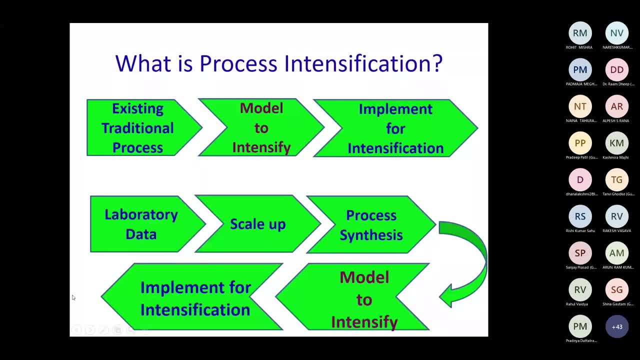 data which will give some hazardous property of the waste as well as treated waste, and quantity of that treated waste as well as quantity of the uh incoming influence in the effluent treatment. so that's what we're going to talk about in the next part of the presentation. 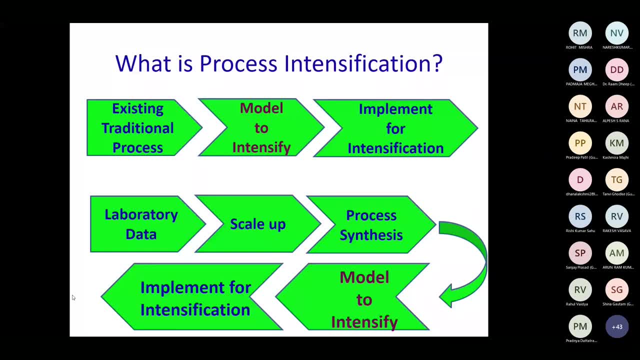 so thank you very much. the next part is my project, which is a report on the possibility of use of some large scale data, um, in the aging treatment plant of the industry. and using this laboratory scale data, how to carry, how to facilitate some change in the main processing steps requires some rigorous research and development studies in at the 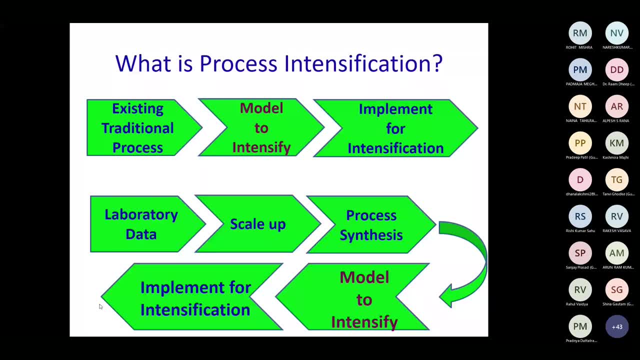 laboratory scale and these laboratory scale data need to be scaled up in order because ultimately we want to attended goal for our commercial product or commercial process. so in order to convert that laboratory or pilot plant studies data to that commercial food scale plant, we need to do that scaling up of 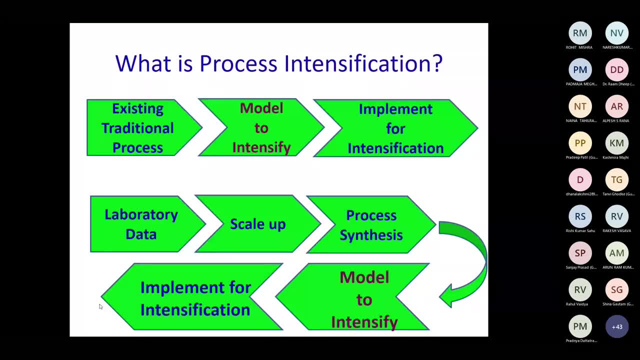 that and that is very related to that process synthesis. so, ultimately, beginning with that modeling when they, by implementation of that particular model, they will reach to that final destination. so that is the main concern. like maybe, if you want to see what is, what was the initial step? the initial step was simply this existing traditional process. 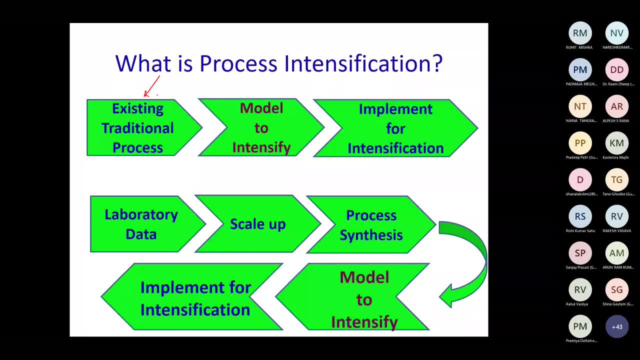 if we are having at our hand or at our plant site and using some models. this model may be physical model, maybe mathematical model or some simulation tool which will give us some appropriate model and how to implement that particular model in order to divide the physical processing steps or sequences of various operations and chemical reactions. so again, if i 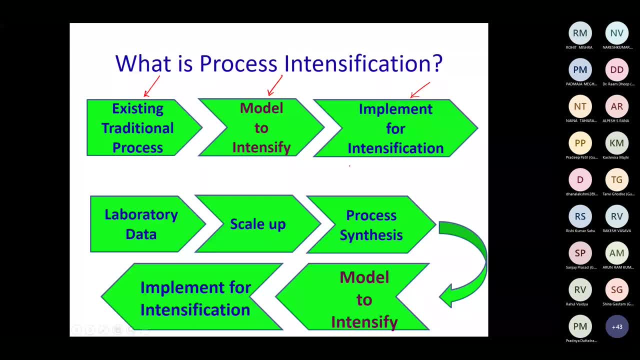 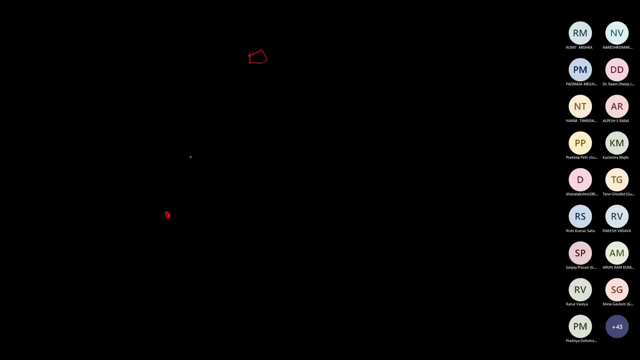 want to elaborate the same thing, like if i want to reach from one destination to the other destination, what are the routes available? like one, maybe this one, maybe i can go at this station and move this place. another is directly, i can go from this road, but this, there may be lots of. 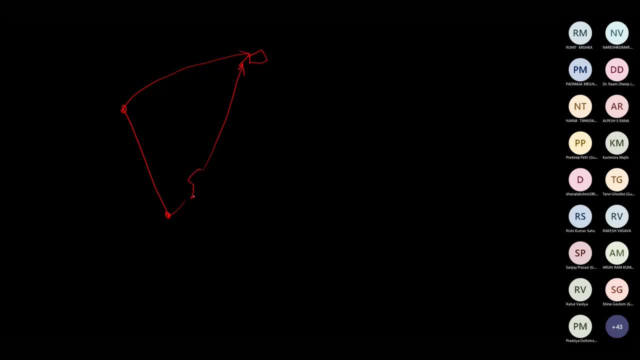 disturbances may be present in this in this region, so i some situation may not allow to cross this barrier in my travel now. so in order to avoid this kind of divergent, i need to go, i need to avoid this shortest route, and this is similar to some process constraints. 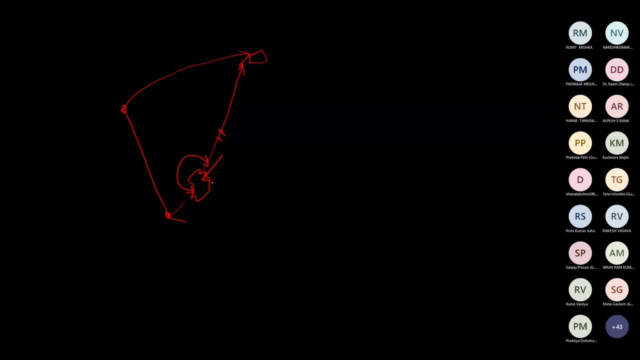 or sometimes the chemical kinetics of particular chemical reaction, will not allow us to alter size or the type of that particular reactor or the some utility requirement or some catalytic requirement, and enhance. in order to avoid that thing, we need to, uh, find some other ways which will directly and 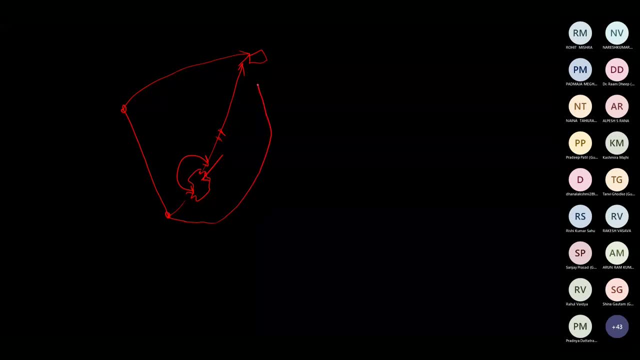 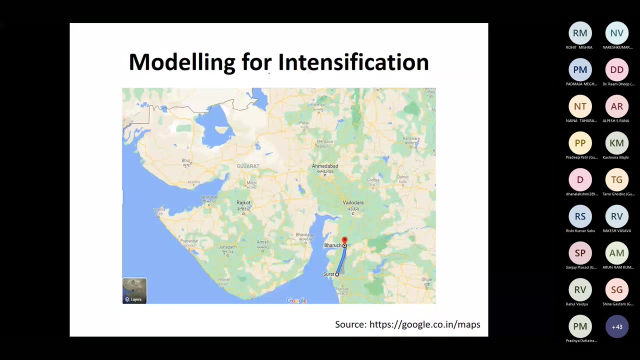 safely and timely allow us to reach to that particular destination. so that is the main thing in this process in transportation again. but just for example, if i want, so you know, if i want some, let's say some solidéta want to uh, travel from my institute to this organizers institute? uh, this google is giving. 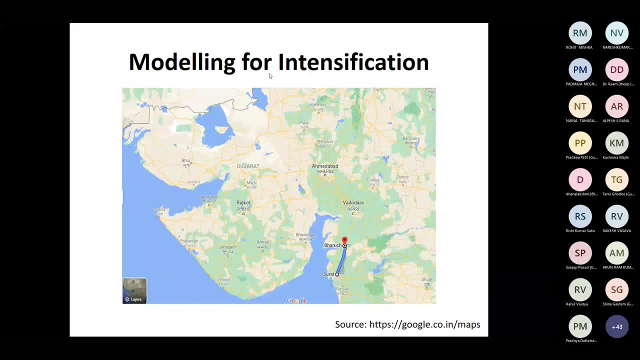 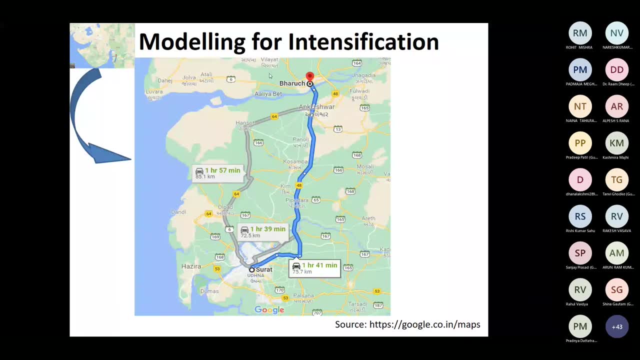 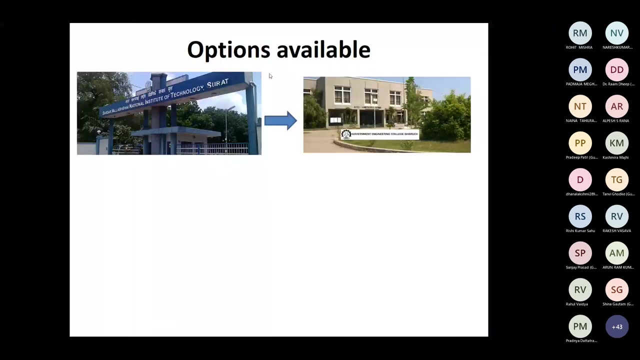 me this kind of map and when i zoom it it will show different options for traveling to train, traveling to uh by roadways, and even in the roadways there are also few options available. so i i am having a few options. like, i can travel through train, i can travel through. 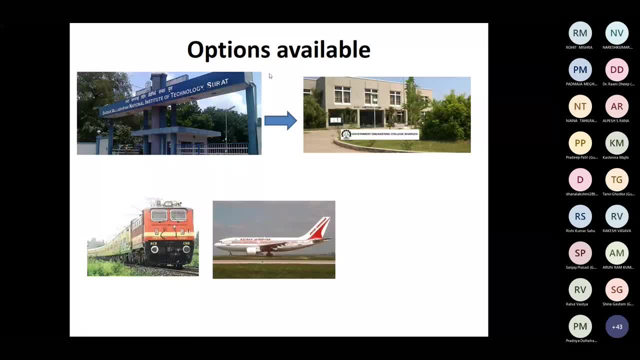 this vehicle or ultimately, this thing. so all options are held out. unique features, but will which option will give me the more flexibility for traveling and reaching timely destination? that is the main concern here. so so this is: what about that intensification? now, how to implement this thing in our based radiation. so, as we have just now discussed the 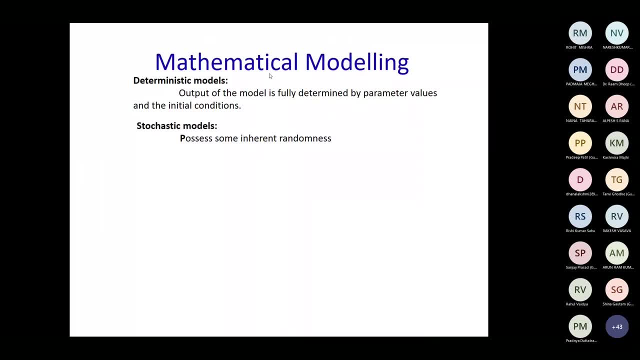 basic things is. the very first step is the mathematical modeling. and again, in this mathematical model, there are two types of models. uh, one is known as the deterministic model, the other is stochastic models. so ultimately these two types of models depends on that randomness. so basically, this stochastic models incorporate some inherent randomness, whereas in 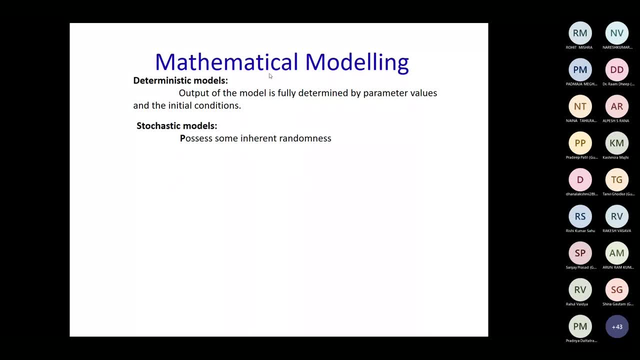 the deterministic models, uh, associated with some sort of output of models, is fully determined by the parameter values and the initial conditions and using that condition we need to frame some mathematical expression and we're following that mental equation or that model equation. we can, as when we have that required parameter, and that required parameter need to be optimized again for 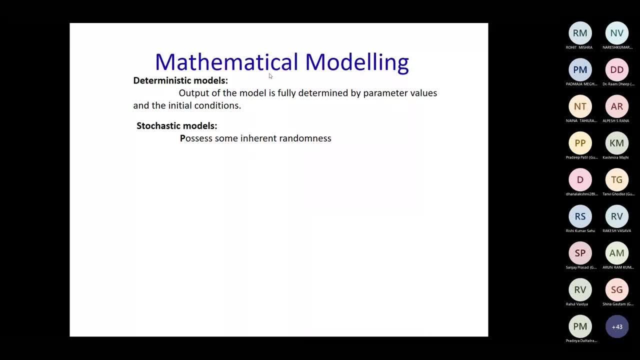 optimization we need to. we can adopt any trial and error method practically, or you can also go for some sort of similar optimization. techniques or design of experiments will also help us in that case, in order to eliminate some data and to have the optimized value of our required parameters. 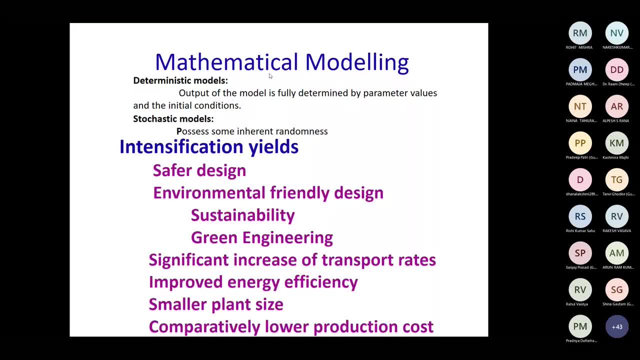 now further that ultimately, when we implement that model, so what will be the final achievement? so maybe the process equipment may be the same, or sometimes the flow sequence may get changed, sometimes the entire equipment get replenished or replaced by some other significant change in the geometry as well as the type of the reactor, type of the separators. 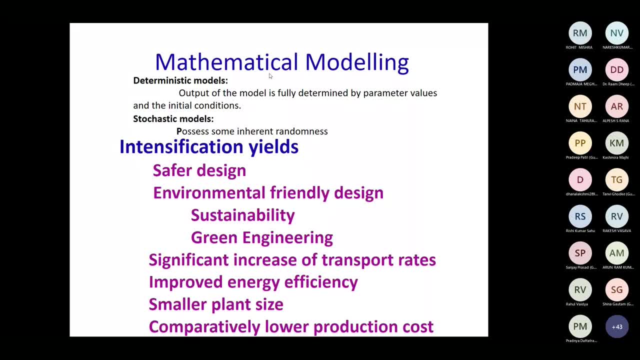 but ultimately the final intensified process will give more safety, more safer design with the same product or same initial and final stations. second is the environmental friendly design, because while in self-intensification then we are talking about that with the mediation, we need to think about that sustainability. 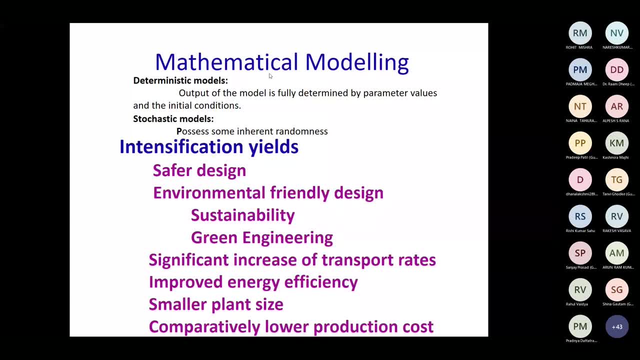 uh watch the sustainability of this particular process and if we are going to change from uh processing equipment by some most sophisticated equipment, what, how flexibly it can cope up with some new instrumentations and how that man power will be trained in order to handle that particular assessment more safely. 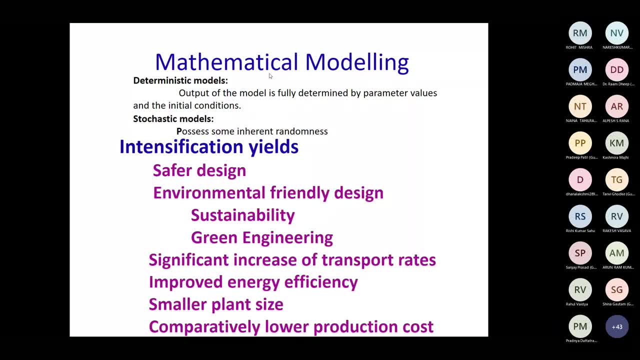 結果 And besides this, we need to also think about that environmental sustainability and also the market sustainability as well in the same case. So some fundamental concepts of the green engineering, sustainable environmental processing we need to consider in order to design or implement that process: intensification when. 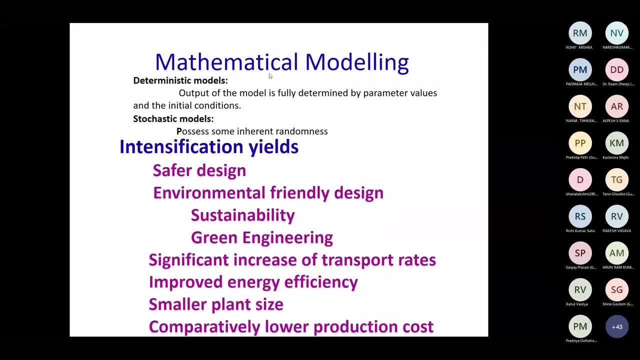 we try directly from the mathematical modeling. So another advantage is a significant increase of the transport rate, mass transfer rate, heat transfer rate will greatly increase and hence we can have that rate of production of final products may be very significantly increased. So, but what to in the case of the waste remediation? so in that case, how can we reduce? 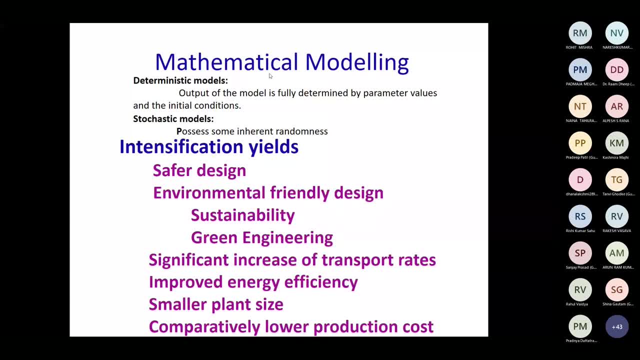 the overall quantity of the hazardous waste significantly in that quantity. So that is the main concern: while doing the process intensification for the waste remediation And from ultimately this, when we implement the process intensification, we can reduce the overall quantity of the hazardous waste. 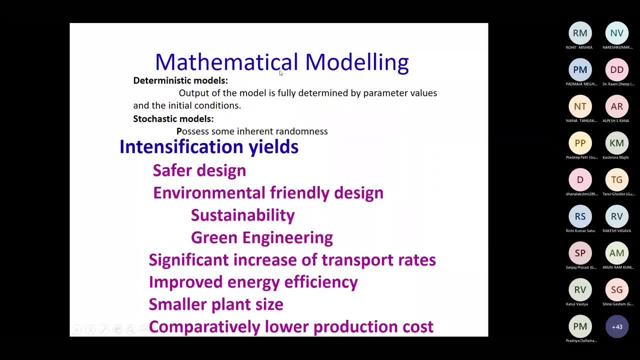 So that is the main concern. while doing the process intensification. So that is the main concern. while doing the process intensification, So that is the main concern. while doing the process intensification. As now we understand the process intensification from this mathematical model, we can also: 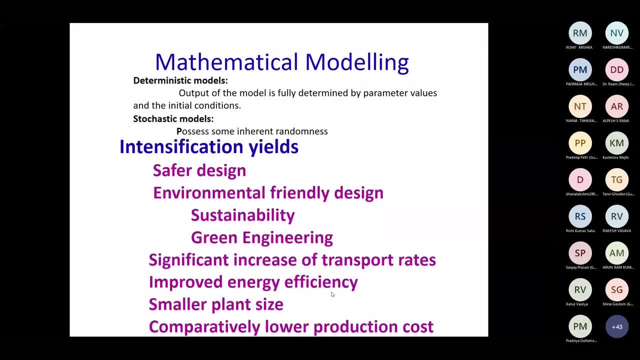 come out with some smaller Corinth scale of plants or even from smaller size plant to be. we can have the same or the better quality of the product, but clamorably that this throughput may be drastically minimized, As now we understand the process: intensification, which requires high speed and cutting out. 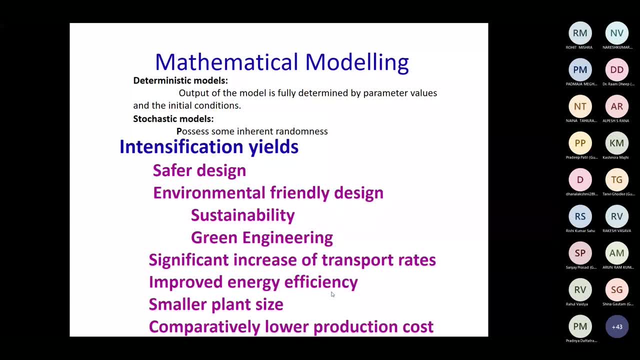 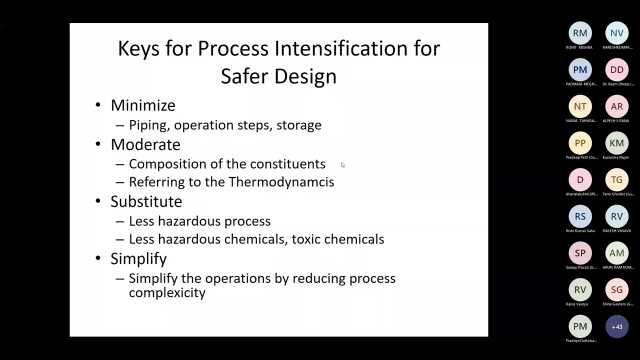 So ultimately, all these things will result in more safer design and also cost effective as well as energy efficient processing. So these are the main advantages of process intensification And what we need to do, especially for safer design, in order to implement that intensification. 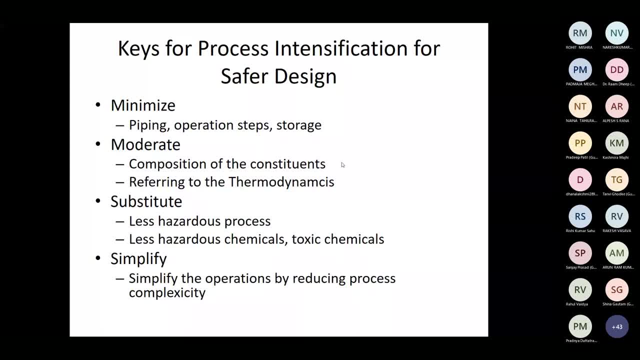 So we need to minimize that. overall piping length means the overall transportation length of the fluids need to be reduced. operation steps need to be reduced. overall storage strength size. So these are the main advantages of process intensification- Or that overall intermediate storage tanks need to be reduced, or the size of them all. 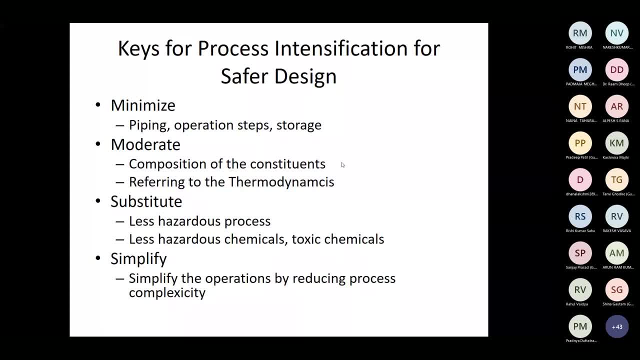 these equipments need to be reduced. So means when we talk about the decrease of the size or the decrease in that overall length of transportation of the fluid, in that case we need to consider like ourselves, as in the design stage only. So lots of things in the process: intensification starts at the design stage only and some moderate. 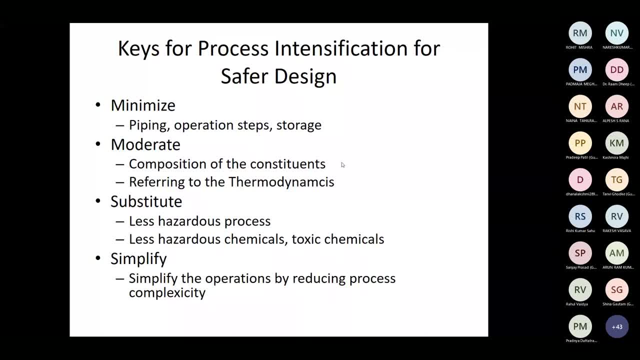 change in the composition of the constituents may ultimately lead to lots of poor savings in the material of construction of various vessels, as well as processing steps may be easier. So if we make some moderate change in some material, this is the special thing we need. 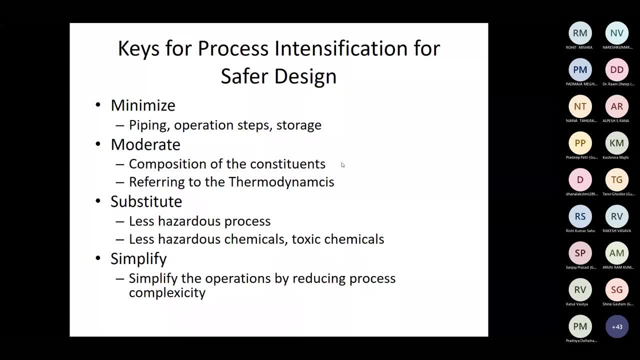 to consider because ultimately, our final product is fixed. Sometimes the raw material is also fixed, but what are the other intermediates or intermediate processing steps involved in the overall conventional process? we are having in our hands to work on that, So we need to consider that. 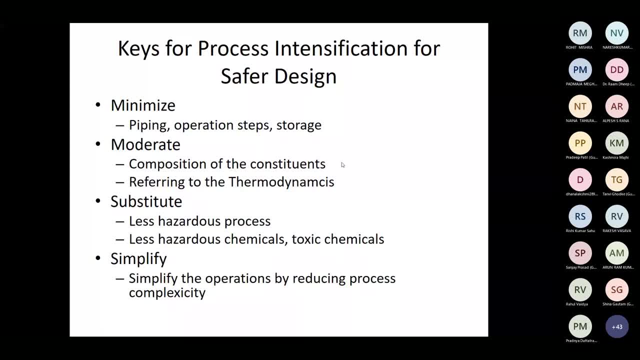 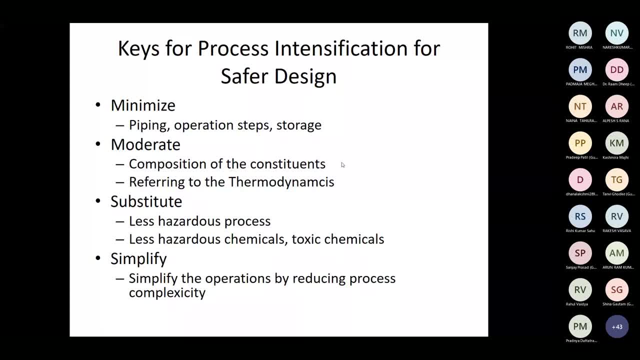 in place. So if we want to get the fat that we have made the foundation of the final decision and we have to play with some started parameters accordingly, we need to change that available parameter not rightly, and this will only lead to the final design. we could be more. 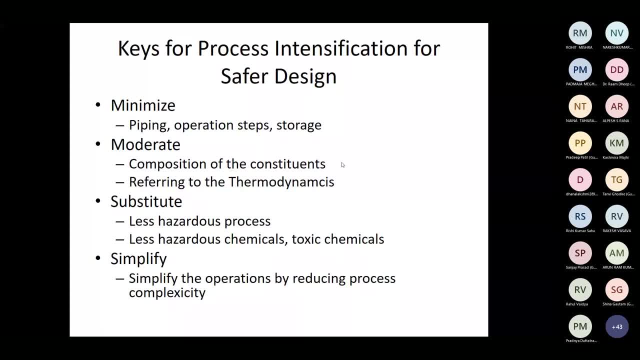 safer than the initial one. So, in order to do these, two things are of lots of import: the composition of the constituents and thermodynamics, Because the thermodynamics are often kort. Yeah, we ultimately deal with that. uh, conductivity is the heat, or the heat capacity and quality. 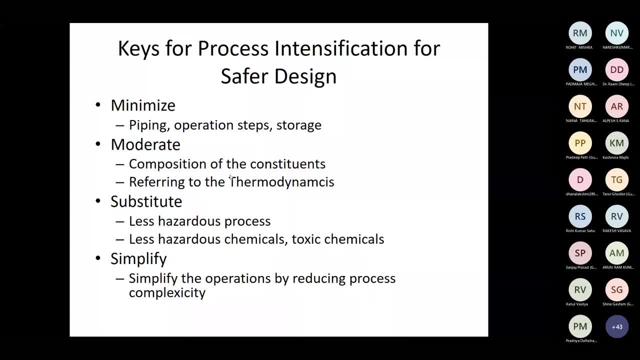 of the substance and hence, for some, um, even even simple mixing may be associated with lots of heat of mixing or heat of solution, and that's why we need to consider this, uh, energy transfer as well, uh, and even the moderate change in that temperature condition sometimes, uh, ultimately, 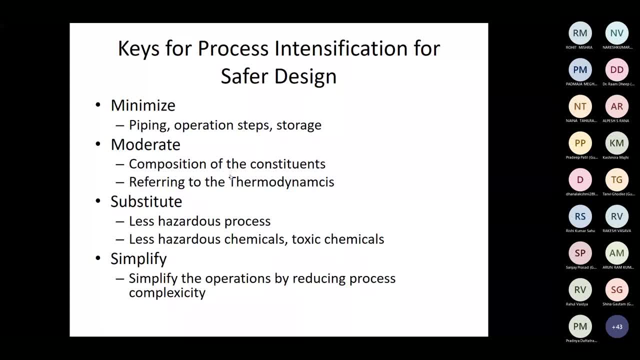 resulting a lot of drastic change in that overall heat transfer or mass transfer. then the third component is to substitute another component in order to avoid certain hazardous materials. so, if possible, if, if it is in the hand of the designer, then the third option is to choose the least hazardous process route or the least hazardous chemical we can substitute. 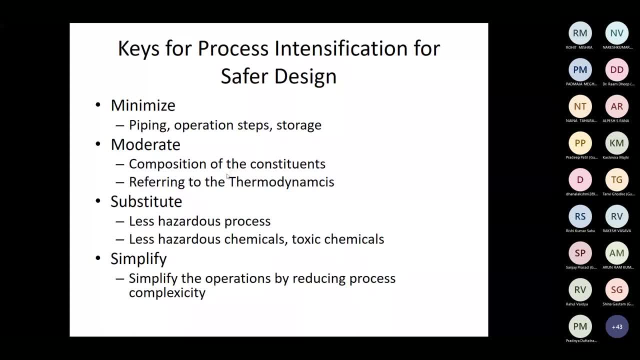 the most hazardous chemicals which is going to be utilized in our final product. so means, ultimately we need to think about the toxicity or hazardous characters of the chemicals used in the processing step and the simplification of the operation. we ultimately solve lots of complexity of operation and the manpower can easily handle uh simplified operations. 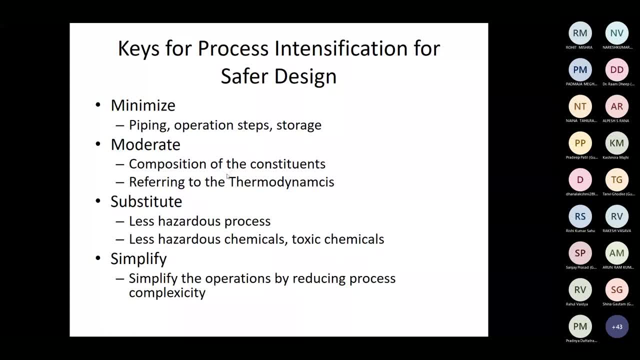 even though some complicated instrumentations will also facilitate easy control by the workers who are working in that plant and the plant area, and hence, uh, the proper alarm systems, proper control or the flow control will be necessary in order to simplify the process, which will ultimately result in the smaller size and safer 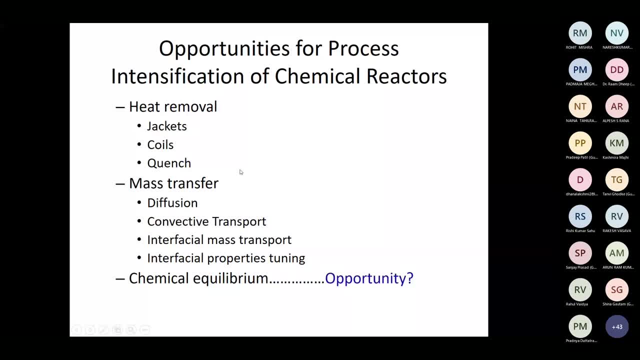 design. so like, just for example, like, if you want to remove the heat, we can have the options of quenching with some other material, implementation of the coils in the reactor, or provide in the jacket outside the wall of the vessel. now, which out of these three will facilitate your purple? 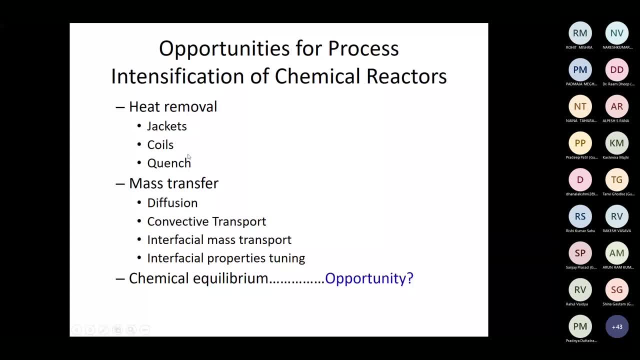 for for heat removal, if the contamination is the core stolen, what should be the better thing? if the heat transfer coefficient is the ultimate driving factor, then what need to be chosen from the checkers or coils? what are the corrosive environment if your coil is going to be immersed? 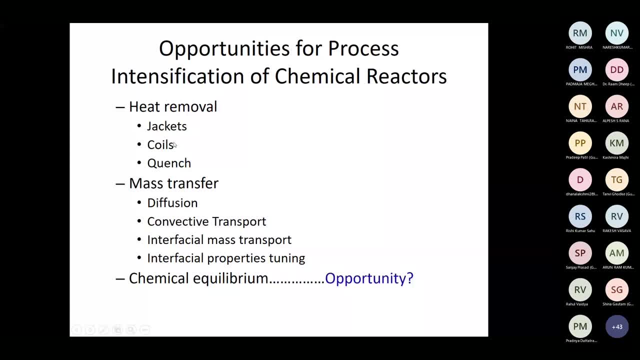 in your processing fluid, like suppose you are having this reactor and if you want to utilize this coil and if you are using this coil in such a way, so, so suppose this is your cooling coil. now this entire equipment will get filled with the processing fluid and hence 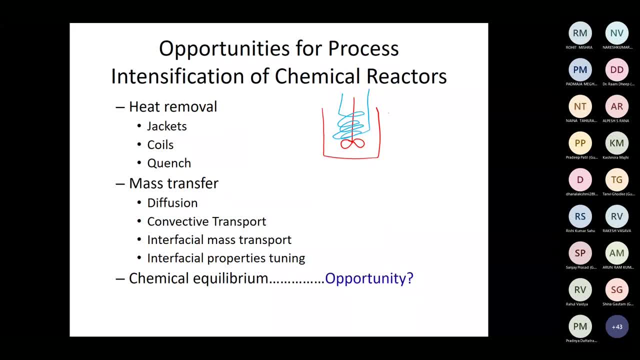 this coil is going to be submerged in that, inside that processing fluid, and if your so, what i mean to convey is, in this case, uh, even though your, if you have chosen your material of construction of the coil, which will ultimately result in a higher thermal conductivity. higher thermal conductivity, you know, less heat transfer resistance and, at the same time, 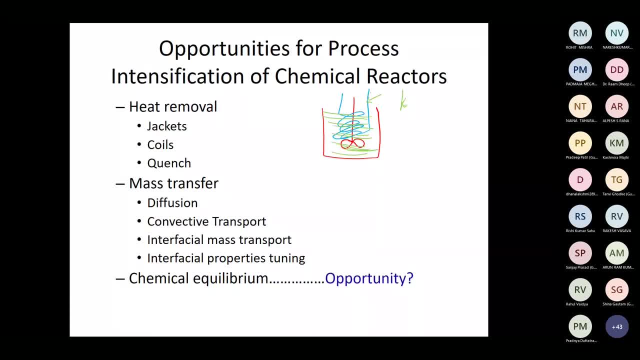 what is that thermal media which is going to flow inside this coil and accordingly, the material will be compatible to that thermal fluid which is flowing inside this coil now. so so that uh nature of that thermal fluid will ultimately affect the material of construction, but at the same time, the constraint is the thermal conductivity. 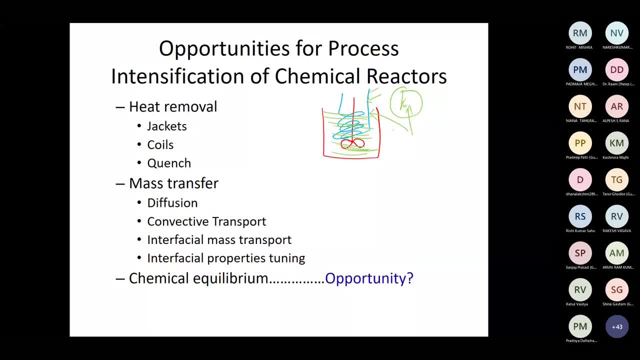 now, now here, when we are using the coil. at that time, its external surface of the coil will be also exposed to this environment, because it is in direct contact with the processing fluid and hence, if your processing fluid is corrosive, it will also corrode the outer surface of this coil and, in that case, the utilization of the coil. 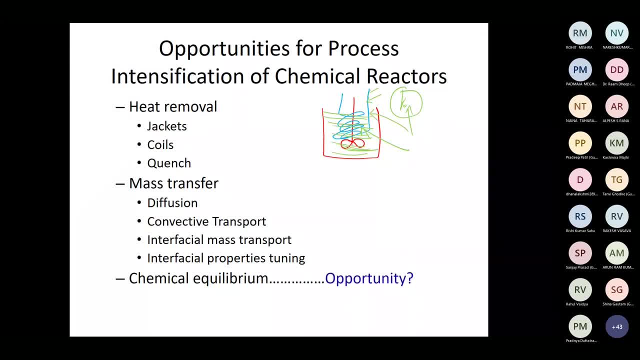 is not advisable. So what to do in that case? So in that case, jacket will be the better option, Jacketed reactor will be the better option and hence only this reaction vessel valve we need to consider, we need to bother about the material which will. 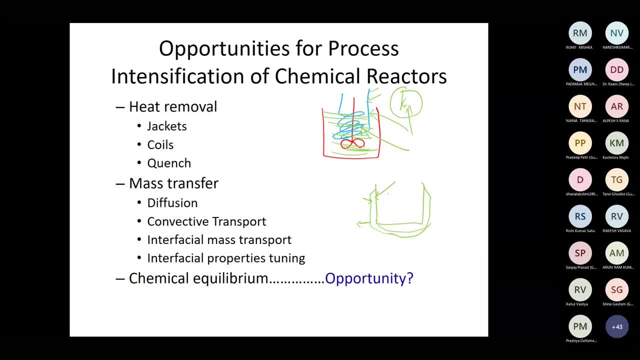 provide us with less heat transfer resistance, more high thermal conductivity and, accordingly, that the corrosion environment will be only at the inside surface of this valve, and outside surface is normally that for heating or cooling fluid. Now, in the case of mass transfer, if we want to, 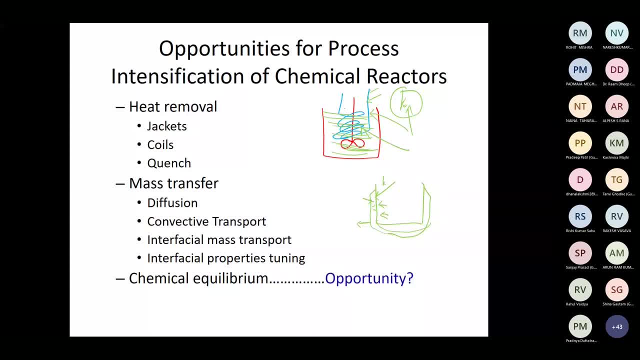 change any subject which are considered by mass transfer, then is it in our hand to change the diffusion of some substance, How to alter the mass transfer coefficient For particular cross mass transfer separation operation. Then if it is mass transfer diffusion, then connective transport, or is it what kind of? 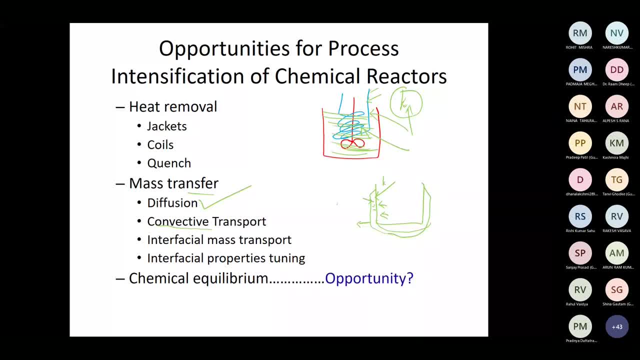 diffusion is taking place. What is the degree of turbulence in the fluid or what is ultimately leading to that large chance or varies to which the mass transfer coefficient is taking place In your reaction media? And, uh, interfacial mass transport. Uh, this is very important thing over here. 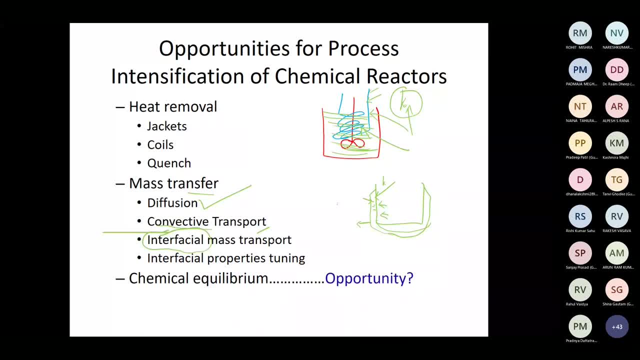 interfacial mass transfer. There are lots of chemical reactions as well, lots of uh mass transfer processes in chemical industries which require spatial attention when we want to uh transfer one species from one phase to the other. For example, if I 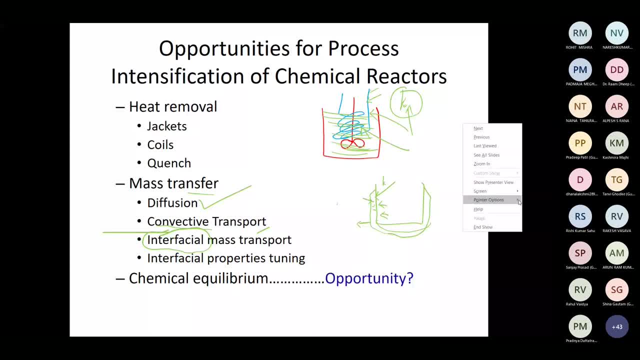 I was both. here There is a membrane and on this side I'm trying to transfer. I'm trying to transfer, Let's say, a one order membrane. this side we are having one liquid, or you can consider, suppose this is a large droplet and this 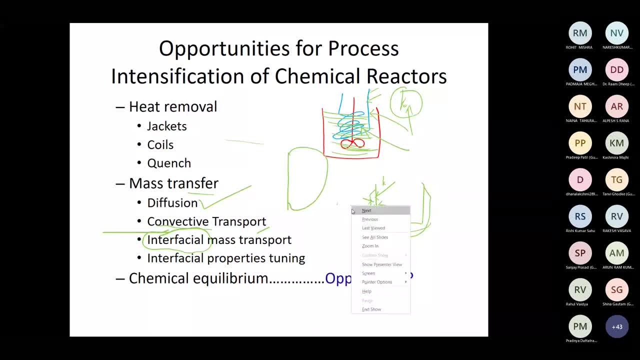 is continuous, this is your continuous liquid. and here, in this continuous blue liquid, one drop of this, another liquid color with the green color and, as you suppose, one of the constituents, like this a, is going to transfer from the bulk of this blue fluid and it is going to enter in this drop here. so what are the resistances offered by this system? 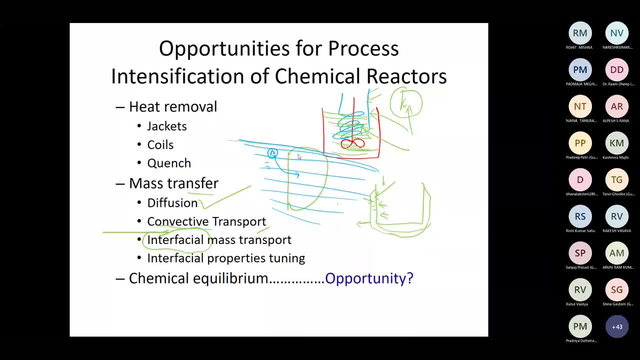 in order to travel components. this is a from this place to this place. this is your station number one, this is your station number two and while traveling, it has to cross this barrier. see here, this now, how much resistance is offered by this fluid itself. any idea, you can interrupt me anytime if you have any doubts or any query. 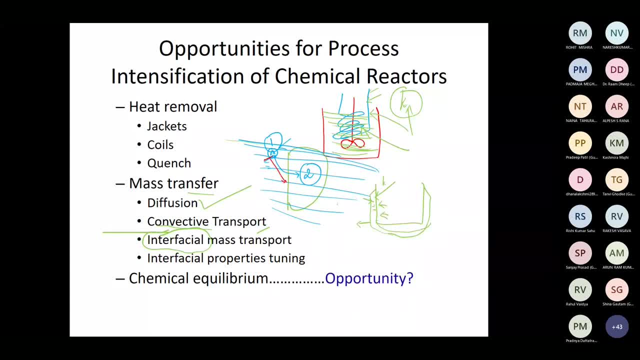 so i have asked you what are the resistances of this fluid and what are the resistances offered by this? all the water parameters which are ultimately resulting that a different kind of resistance experienced by this. this is a while traveling from the bulk of the fluid to this boundary. 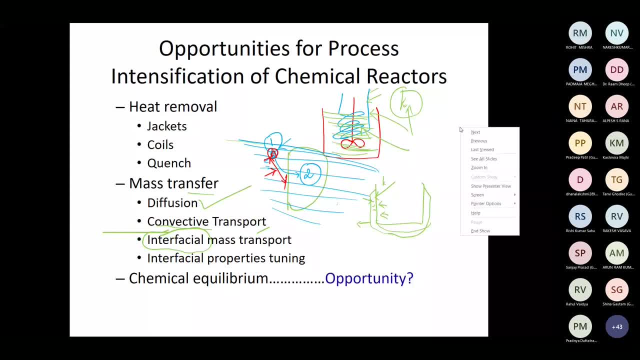 so we have this flow like this in terms of when the weight gets'll in the width of it. as you'll see in the video, what this flow is is a flow like this: in terms of how much resistance will that give you one or two years? in terms of how much resistance that we would have. 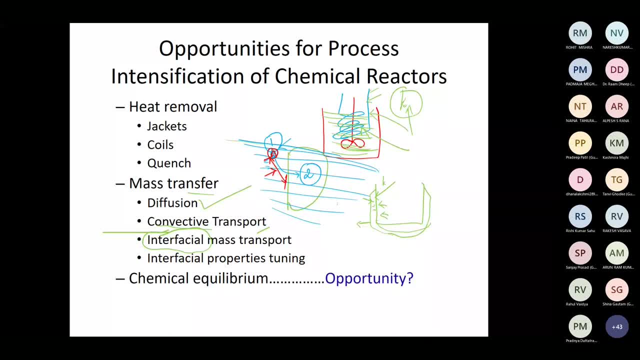 in the future. so when you consider that or you consider that as a number of things, it has a different type of resistance. we can see that the change of present freedom in terms of the flow of the fluid from the center to the center is much less than the flow of the fluid itself. 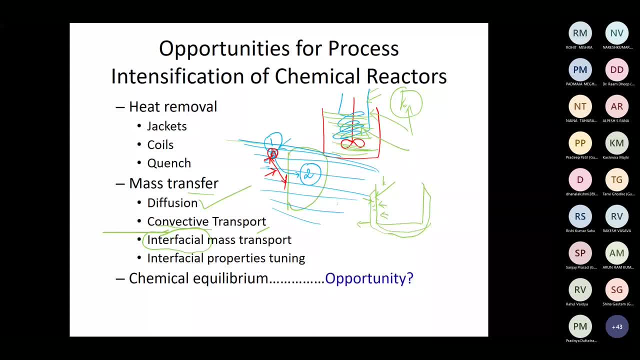 huh, anybody continue, sir, pardon, no, continue the session. yeah, yeah, yeah, yeah i. i have asked something like what will be the overall resistance offered by this disease, a while traveling from the bulk liquid to the boundary of that droplet. so so see, uh, depending, do you think in this case, if you? 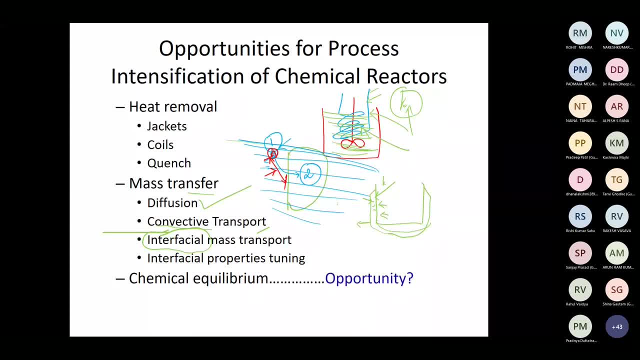 are overall. this distance also matters instead of your a, a species, at this point. rather, if it is available at this point, then this large distance it has to travel from this point to this point. so extra resistance because of the extra length it has to cover. so now, 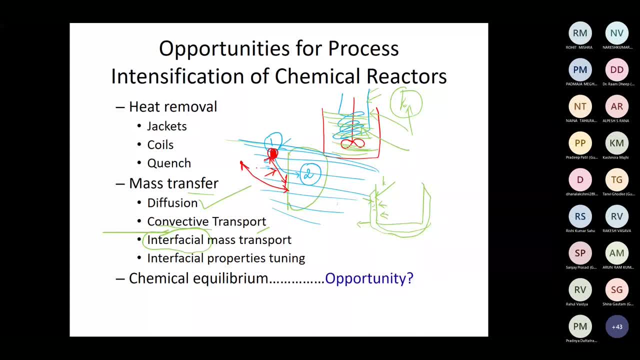 second thing. first is the distance overall. second is that viscosity of this liquid through which it is traveling from bulk phase to this interface, so the viscosity of this blue color liquid. next, if we are having agitator, suppose this entire thing is placed in a vessel. and if we are, 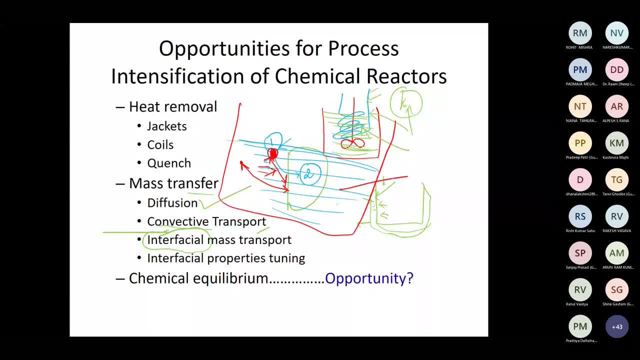 having some agitator or impeller over here. that will also cause lots of convective current and that's why that will facilitate easy transfer of this species a from this place to this interface. okay, so these are things we in our hand. if you implement this kind of agitation, then this resistance can be easily eliminated. 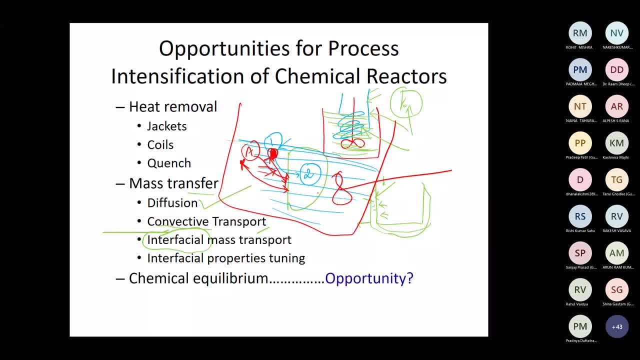 or it's, it can be, not even in some case we can eliminate, but we can reduce up to certain extent. now the second: once it, uh, once it's entered, how, any how, suppose it has entered across this barrier and once it enter over here it will completely intermingle with this liquid or it can go directly. 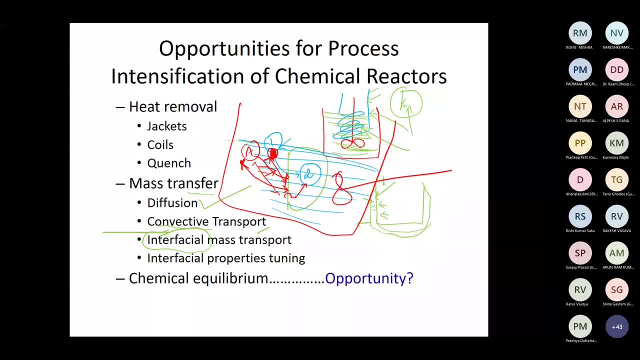 to the bulk of the liquid number two, green liquid, because it may be compatible with that it is, it may have the good affinity with that particular chemical. so you can consider like this maybe, the example of some uh solvent which is used in some effluent treatment plant in order to uh extract. 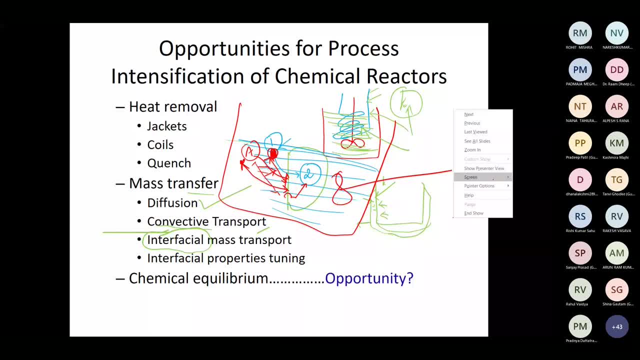 hazardous component from the effluent stream. so if your liquid, if your liquid, if your, this liquid- number two is having high affinity of the component. egg is very hazardous in your influence, coming out from your plant. so you can use the solvent in such a way which is having more affinity and that's why it will. 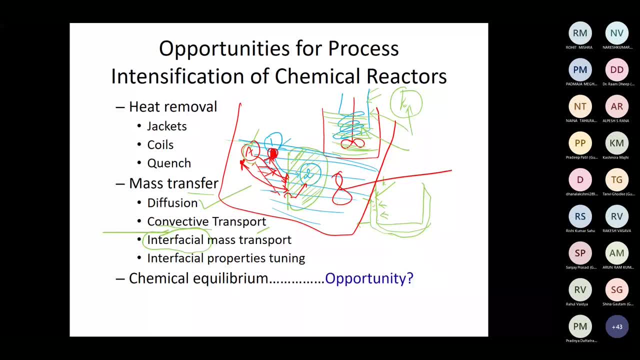 preferentially dissolve only a in it and only a so so. so the resistance of for experienced by this species a after crossing this boundary will be very negligible in that case. so where does what will control this entire mechanism? what will control this entire mechanism? so, that is, how proficiently it can cross this barrier, how proficiently, how efficiently and how. 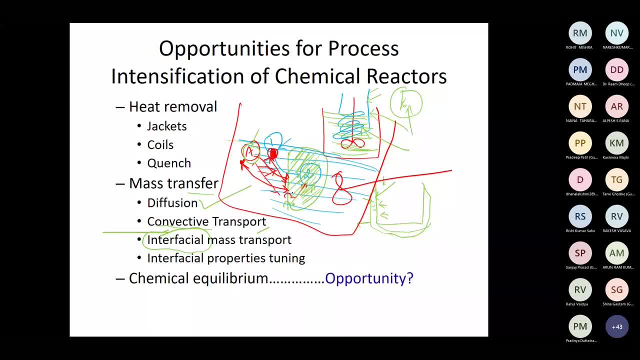 efficiently and how faster it can cross this boundary, interfacial boundary. that is very important because, if this is see the mechanical adjustment or providing lots of turbulence can. important because, if this is see, the mechanical adjustment or providing lots of turbulence can facilitate reduction or the decrease of this resistance and, due to this, compatibility or 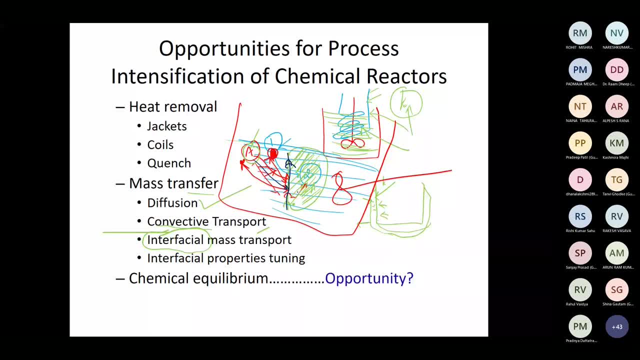 high affinity is of a with this liquid two, liquid number two. it can easily dissolve over here, but the extra effort need to be provided. how, what is the extent of the resistance which is experienced by the species, say, by crossing this boundary and entering from this phase to this phase? that is, 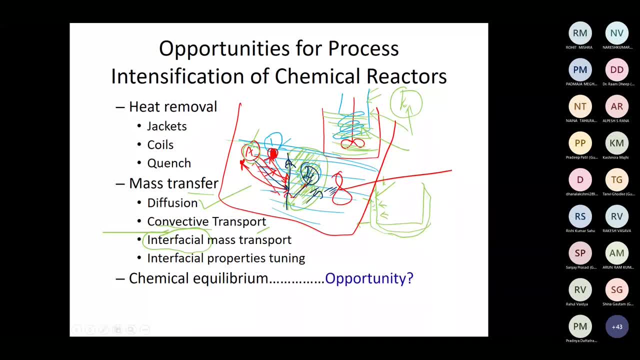 most important. so what are, what are the things need to be done at the interfaces? how to make that interface permeable for transfer of species, a in this case. so we need to look out that thing of interfacial mass transport as well, and that's why, in order to facilitate this thing, we need to 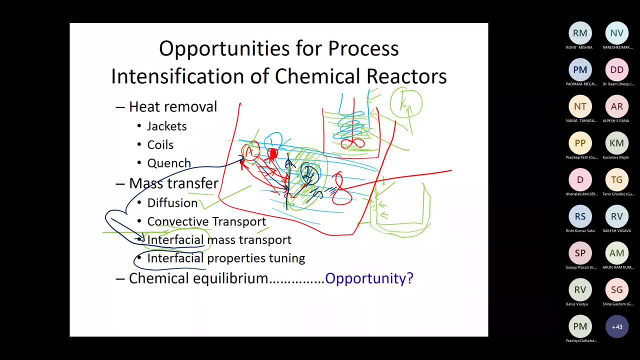 bother about this interfacial property tuning. so what are those interfacial properties? for example, very simple, it is like interfacial tension play a major role in this particular thing and if the temperature tension is decreased, a can be easily penetrate in that liquid, b. 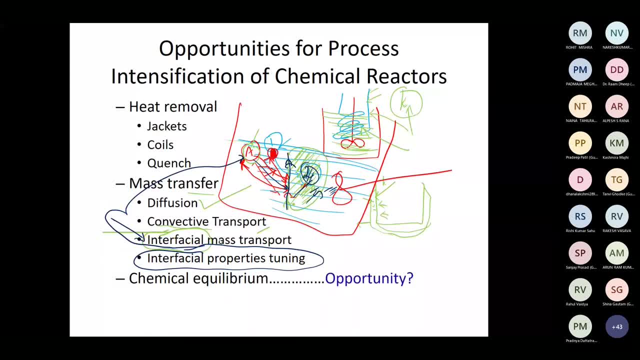 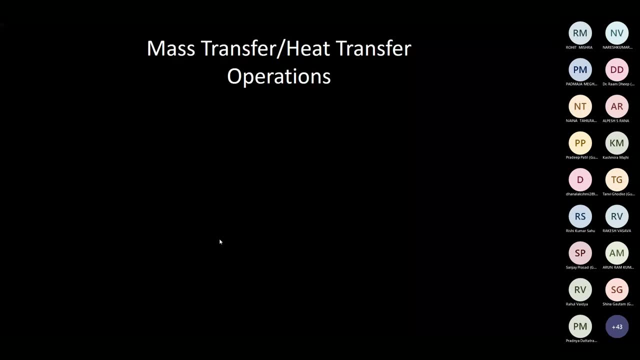 and hence it can control this entire process. so, according to this mass transform, the heat transfer operation will also give some insights of how can we treat our effluent before sending them to neutralization tank or for clarify circulator. do we need to homogenize the overall temperature of the stream? 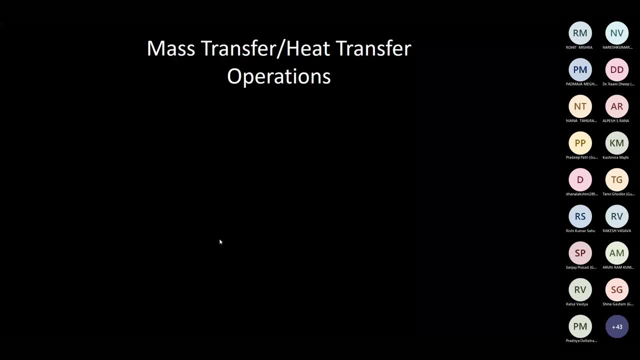 if theicity in this machine varies, particularly in the social temperatures, for instance, if the heat intentionally is kept high in the reservoir or at the home temperature in the land stay large temperature periods during the residents training on the energy generation parameters during tillage stages. they need to cope. 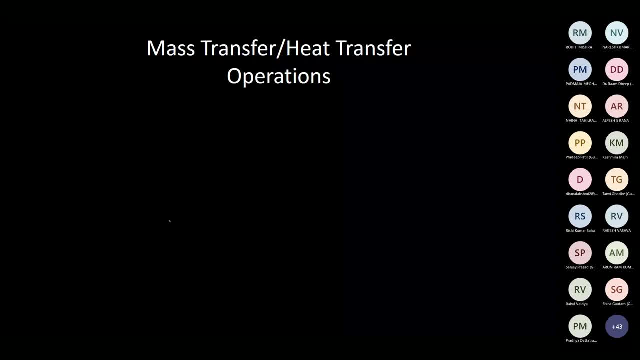 Those embedded caustic gases will bring around好啦ät. не, that's like. if you take example of like, so like, if i so like, it's considered like here i can drive like. these are the mass transfer government processes and these are the heat transfer driving processes. 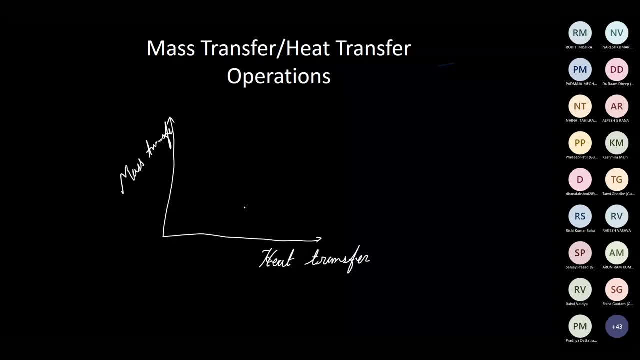 so, uh, like, if you are having some reactor, some reactor or agitator, huh, so that, like that reactor or educator, like, for example, if it is cstr, it will be associated with a lot of transfer, as well as mass transfer, but mainly governed by the chemical kinetics, and that's why the action is below. 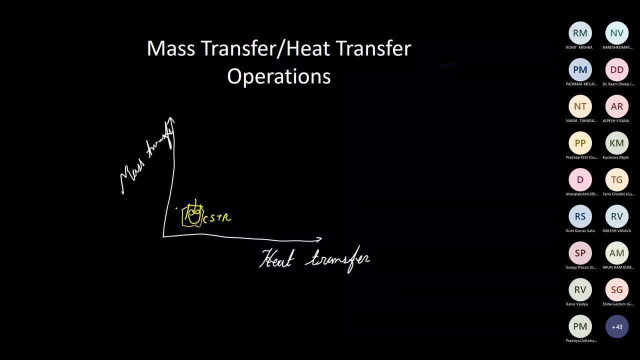 uh, and if you are having some like pulsed column, distillation column, then lots of things to do with the mass transfer rather than heat transfer for that column type of equipment we need to play over here and uh, if it is uh, having some rotating uh tag bait, uh, power over here and also it will have more mass transfer. 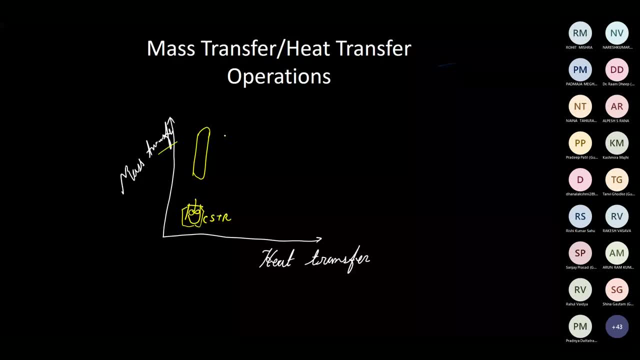 and less heat transfer. accordingly, if you are having some micro reactors uh like, uh, some micro channels uh, which will have high mass transfer as well as high heat transferring. and that's why, uh why, while citing this mass transfer, then put it at this place, because that kind of micro reactor 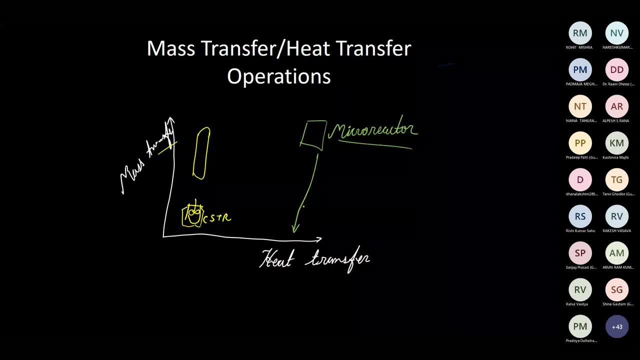 it facilitates high heat transfer as well as high mass transfer rate. if you take simple example of simple plate type heat exchanger or any other type of heat exchanger, then then you can locate it at this place because it will ultimately lead to a lot of heat transfer coefficient, lots of transport take. 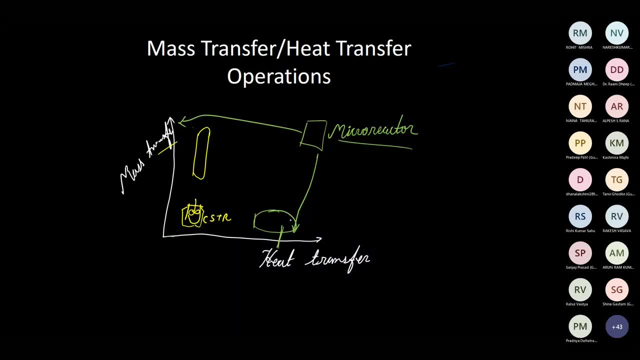 place but accordingly uh not any mass transfer take place in that uh state type heat exchanger or any other themes, facilitated heat exchanger or even extended surface heat exchangers. we are having some assembly like heat exchanger as well as separator reactor, so that kind of 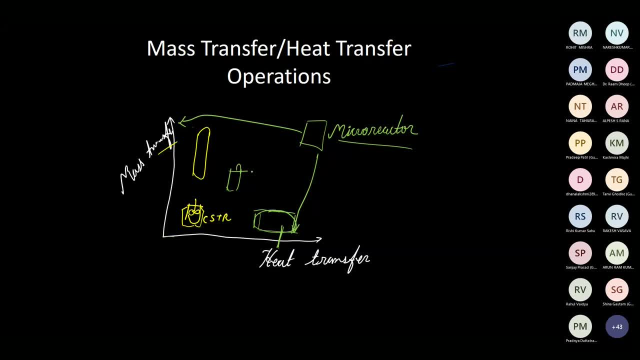 assembly associated with some heat transfer device. uh, if it's going to be heated again, to cycle back, and occasionally some product is taken out and one of the stream is continually created as a reactant. so in this case, uh, depending on the extent on this reflux or recycling, the 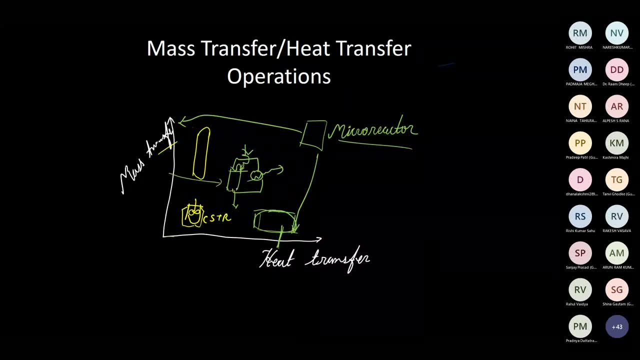 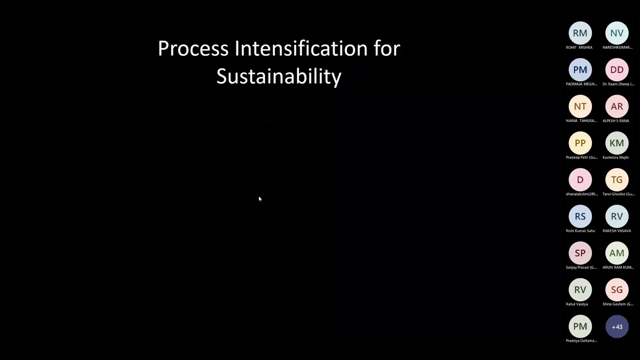 mass transfer will also can get increased and at the same time, the heat transfer rate will also, the transfer extent will also increase. so in order to intensify the process, we need to reduce, we need to decrease the size of equipment, pieces of equipment. we need to decrease the path, flow path, transferring path. we need to 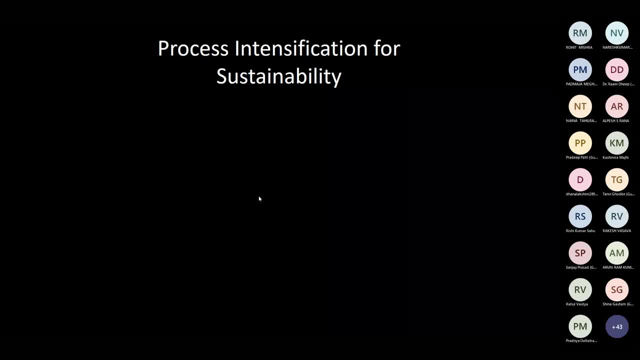 decrease that number of operations, number of equipment and ultimately, that space. so the process intensification when we need, when we are talking about this sustainability, so that sustainable processing requires, so the sustainable processing require obviously process intensification, because we are talking right now regarding the uh process intensification, so this can be achieved by process intensification. 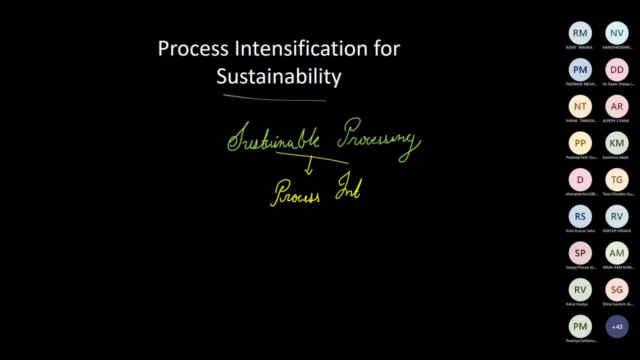 so the process, intensification, automatically. now she'll be Essex, you knowswary, so that activities are Music and global Всё, because intensification and how this intensification ultimately helps us in achieving the final product or that, the final service or the device. so in order to achieve that thing, we need to. 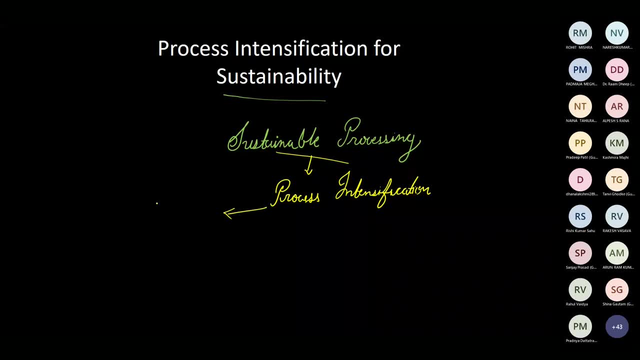 implement it and that implementation will ultimately презид targeted towards the formation of product storage design or process design. On the other hand, this intensification will lead to some new phenomena which is occurring at the molecular level and that will ultimately give us some molecular species or this kind. 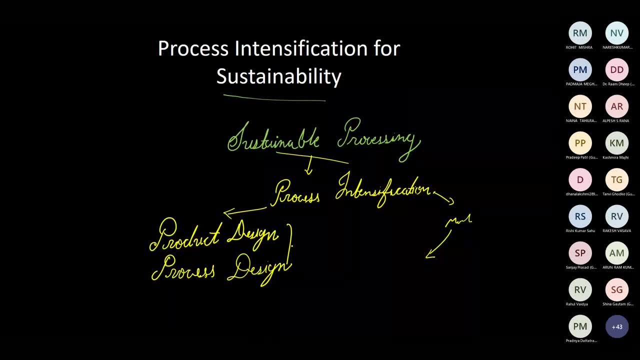 of design will ultimately give us some device and we can have final targeted product or the device available at the stand And this device is matching with that, our own requirement, what was produced or what was fabricated by the conventional techniques. So that is the main concept of the sustainability and intensification. 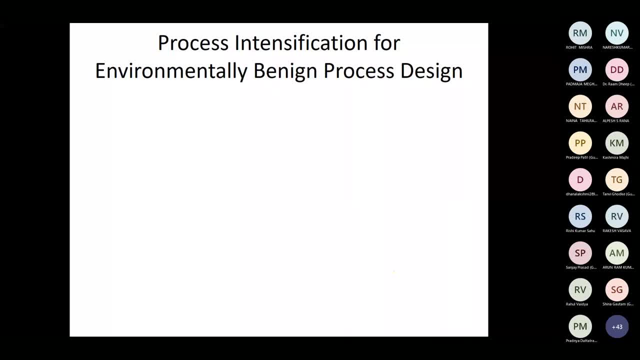 So. So, Rather than altering that unit operations or altering that certain piece of equipment or the flow sequences in the existing process, if we do this process intensification at the early stage, then it will be more appropriate. It will save money as well as time and effort in order to achieve that desired device. 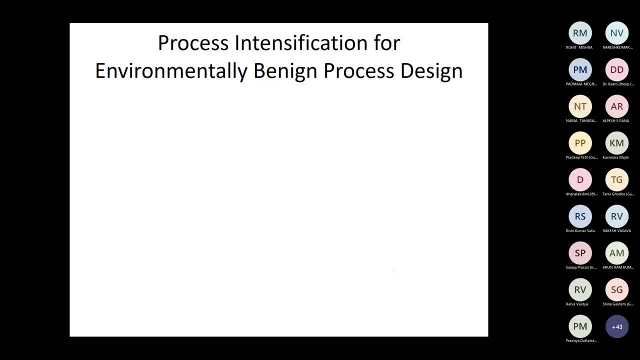 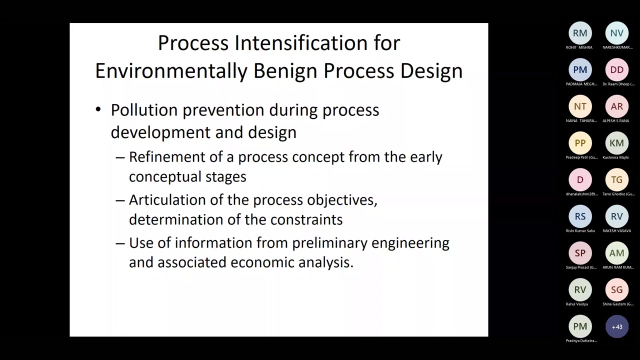 So that kind of process design requires some sort of logistics and needs to be done in the early stages of the design. So the pollution prevention during the process Development and design is the part most important for any design engineer in order to minimize that waste generation in terms of quantity as well as quality of the waste. 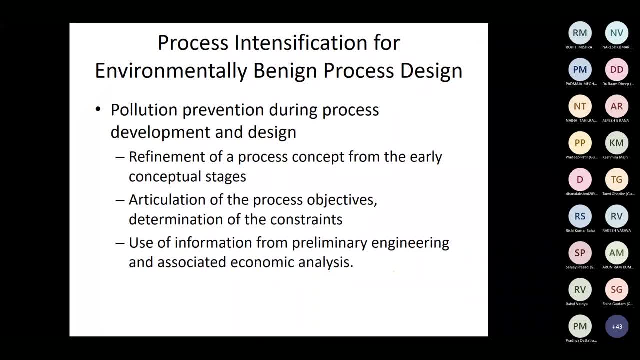 So these are the main points we need to consider while processing intensification of environmental design. So these are the main points we need to consider while processing intensification of environmental design. So these are the main points we need to consider while processing intensification of environmental design. 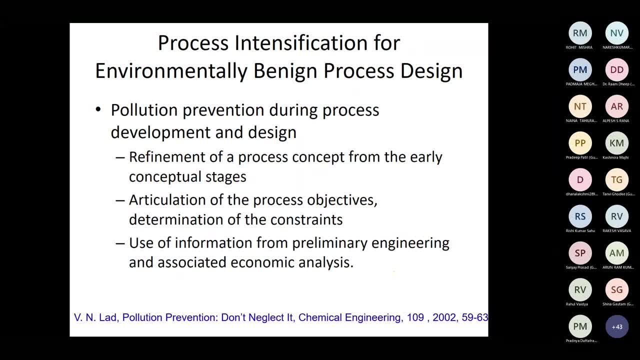 It is now time to talk, with an innovative process, of these systems and some offers are amounting to: And how can we implement these constraints? How can we implement our ideas, new ideas, considering the constraints on hand? Accordingly, we need to work out at the design stage. 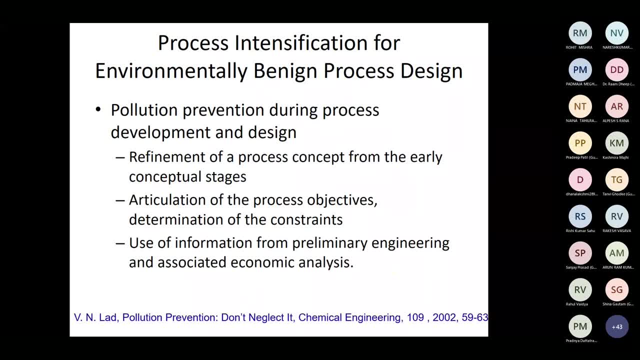 and that will facilitate that easy processing or easy job for process in general. So the use of all the information from preliminary engineering commissioning, scale-up plant, scale-up trial runs and all the associated current analysis we need to work about by 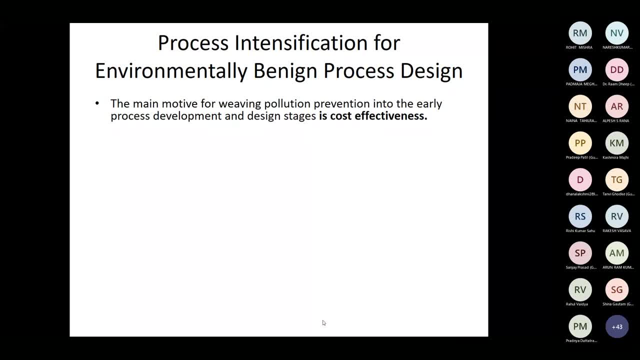 checking that cost-effectiveness of the final product, Because the main objective of all that- the pollution prevention into the early process development strategy- is the cost-effectiveness as well as the more safety. It's something like proactiveness of the design engineer which will ultimately result. 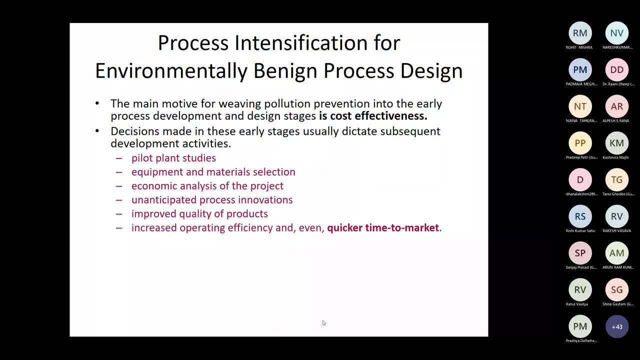 in more sophisticated plants, sophisticated instrumentations and, at the same time, the cost-effectiveness, safety of the working person, personnel, as well as that environmental sustainability- all the things are considered while that process fits Okay. So this is an image in the early stages. 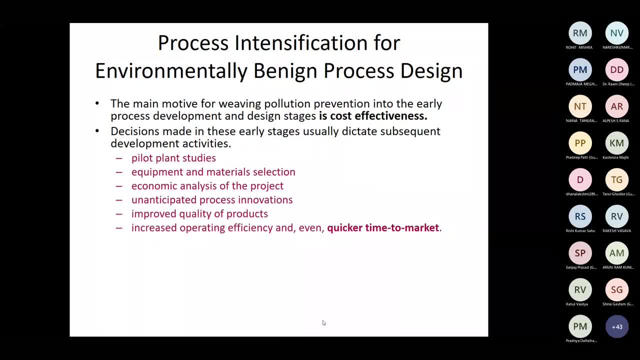 usually the case of development activities, which includes other plants like. what size of your carry fluctuates. what is the size of your neutralization tank? Do we need to provide alkaline breaks, acidic breaks for our neutralization tank? What are the types of? 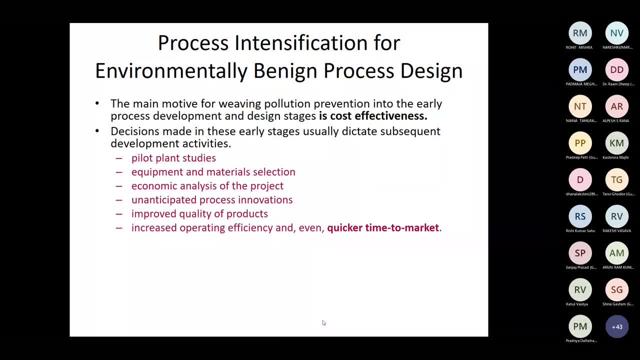 or what is the property or what are the parameters for the alkaline streams coming to your alkaline treatment plant from different plant locations. Accordingly, what are the characteristics? Do we need to mix them prior to entering the neutralization tank? or, if it is more acidic? 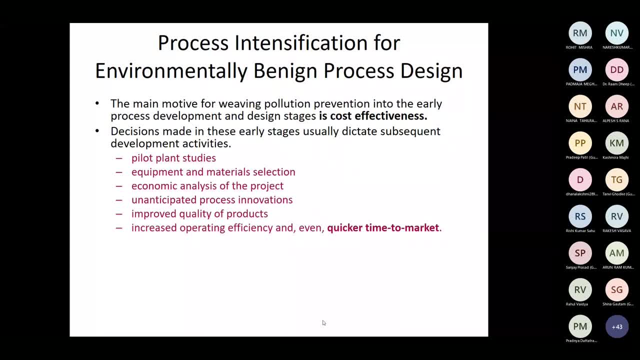 that is treated with that some alkaline substance, and then to go for further processing or further treatment. that needs to be considered at this stage, And what we do, what are time requirements for the processing of your affluencing- is also important to consider during the design stage only. 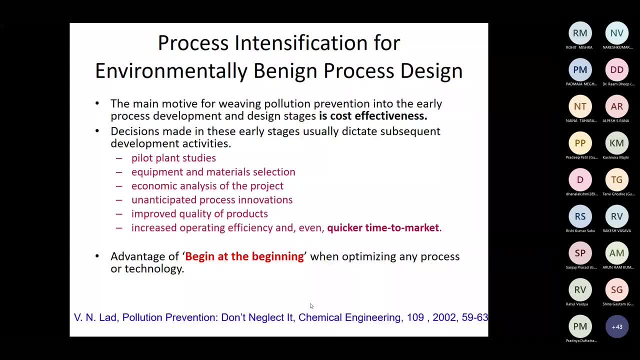 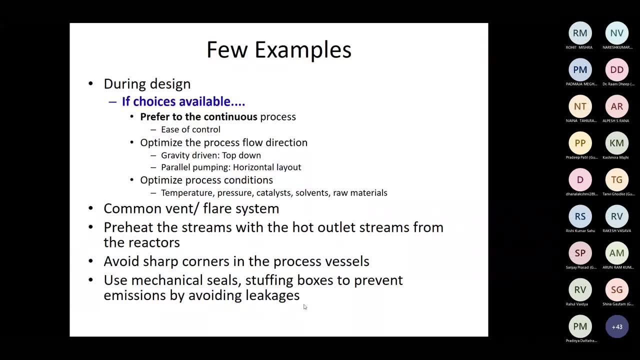 So what are the examples? So if we are having the available choice, then better to prefer to the continuous process because it's having lots of easy control, optimization of the process, flow diagrams like we can have that very hard. Suppose you are having different stages. 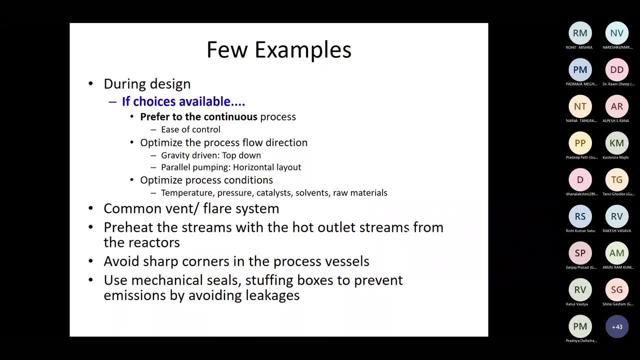 like from this, you have one heat storage tank coming into heat exchanger, your stream goes and then some form of separator, separator truck is coming, got a product. This thing is going to come through. So this is what we are doing. 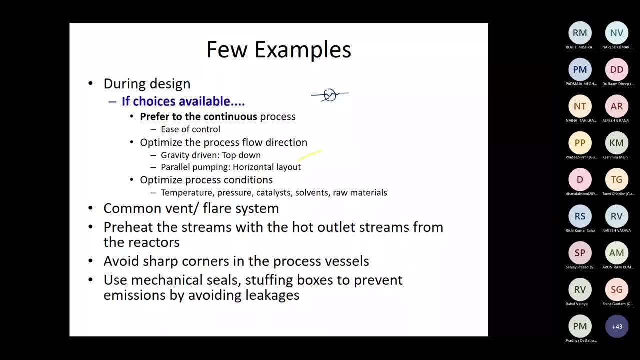 So this is how we are going to do it. So the other thing is that we are going to have to prepare for the storage tanks, the heat exchanger, the stream and then some form of separator. So we are going to have to prepare for the storage tanks. 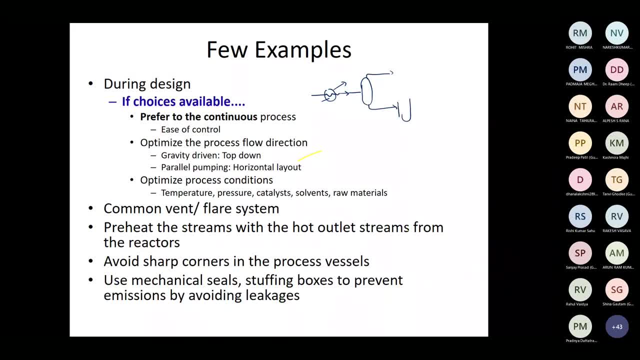 to some other reactor, again going to get heated or cooled and again mixed with something else in order to have that chemical reaction to occur. so if we are having this kind of series of equipment, how to locate this entire thing? what is advisable if we? what will be the overall cost? 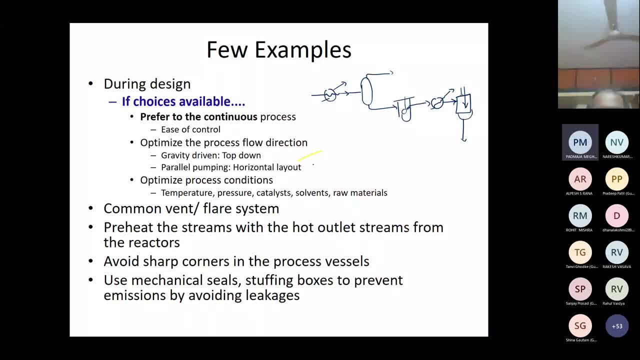 of lifting all this raw material at the topmost floor of your plant, of topmost floor of your plant, and then all this heat exchanger you can place at that topmost floor, then at the bottom, just below it, you can place this again. this reactor will at this floor and these two at the bottom. 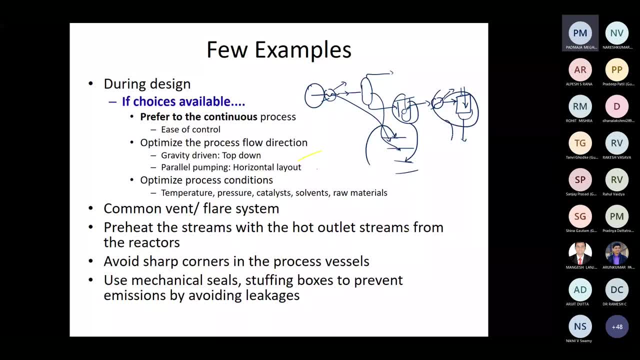 assembly will rest at the ground floor and we can have the final product available at the ground floor. so the only cost involved in this particular operation is to lift the material from this door. how to increase the potential energy. that cost is of importance over here and once it reaches. 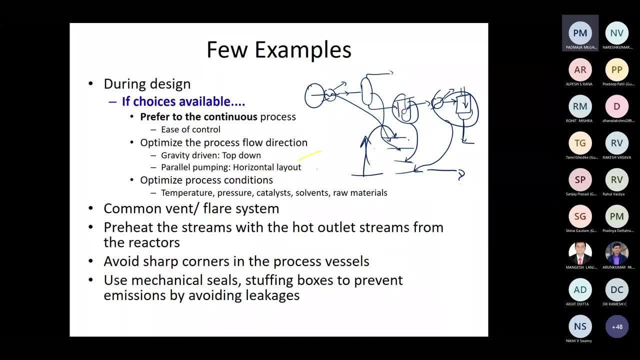 it will completely flow with only due to gravity only. but if we are having this kind of process sequence horizontally, in that case we need to provide the power, either here or intermediate position based, calculating this, uh, taser loss, what is occurring in all these kind of treatments? so, accordingly, the pumping cost. 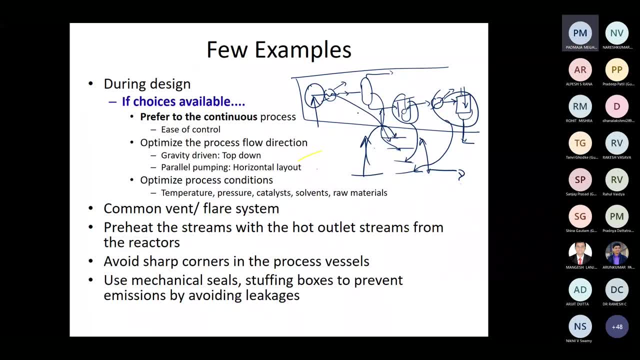 will be so, ultimately, we need to consider the pumping cost in this case, as well as for lifting this material through this elevation. so, uh, in case of uh, in that case, we need to consider the pumping cost in this kind of treatment. so, accordingly, the pumping cost will be so, ultimately, we need to consider the pumping cost in this case, as well as for lifting. 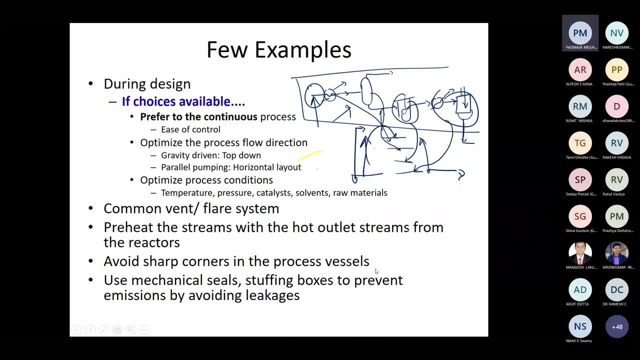 this material for a follow-up process. i forgot to mention that the outside of the unit is going to be at the bottom of the floor and the inside of the unit is going to be at the bottom of the apartment of the unit, so it's going to depend on the type of screw that you're using. 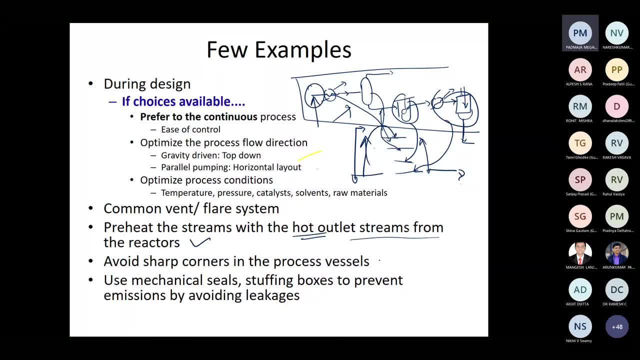 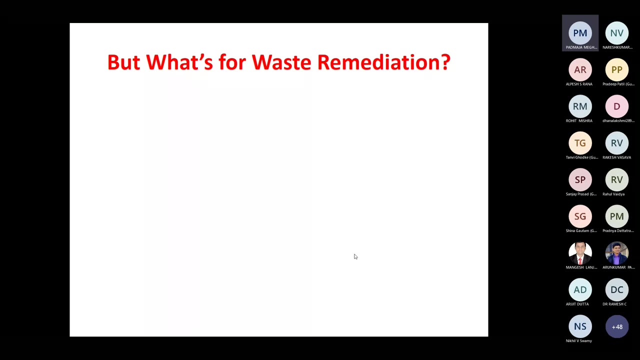 and then when you're coming out of the unit, you also want to Gary, and what you're trying, and the avoiding of this leakage is. so the question may be this: what to do with the base? okay, so again for this waste remediation, we need to think about what are the 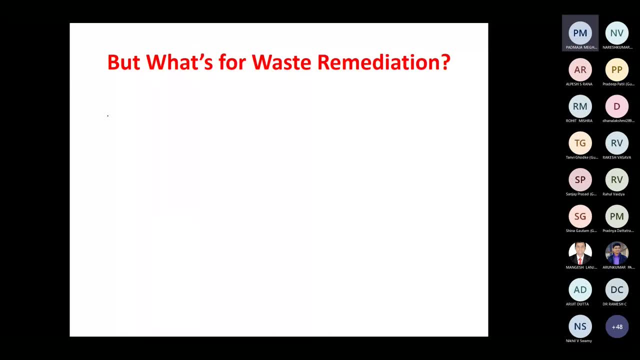 equipment going to be used and what are the methods in that service? so so, with mass and the mass associated with your ect in your ear, effluent treatment climate is some reactor you need to think about. what are the means for reaction, to carry out some chemical reaction or 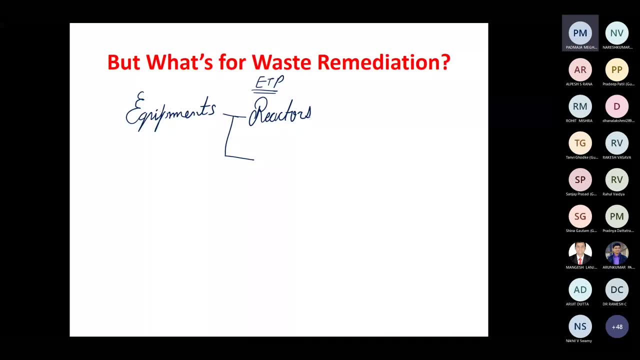 separation. so you need to think about what are the methods in that service also, let's see so the reaction and separations equipment means some separators, like, let's say, to be in a social environment related reactions like neutralizing fangs, incinerators, etc. 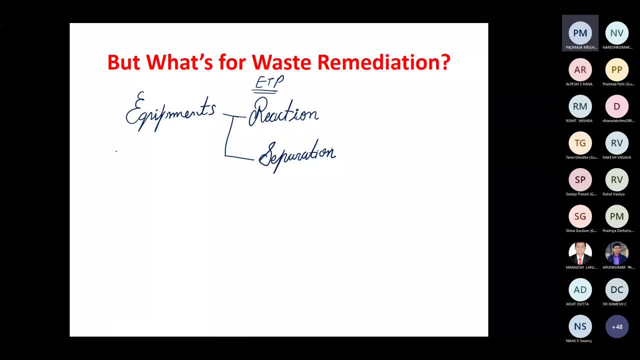 So incinerator neutralizing fangs, polycystic bond, some in double category of the, if you can see, are associated with some kinds of reactions, Whereas clad circulators, separators, filters, strainers are common in this category of this separation. 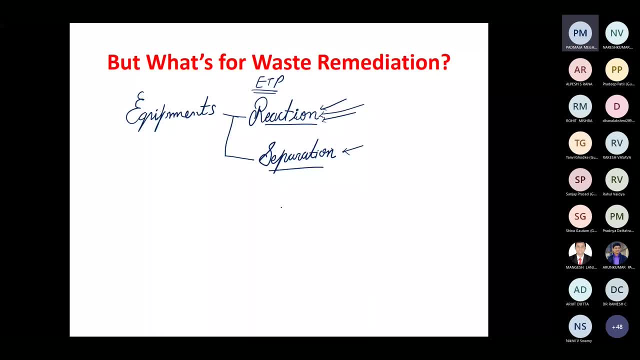 And when we talk about this intensification for this based radiation in case of the mapper, So for methodology, then we need to think about what are the other options available for that based remediation. Is there any other processing route which will ultimately lead to your main? 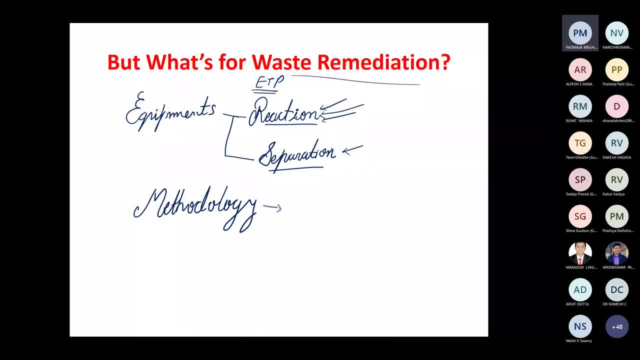 the same product but at the, which will minimize your flow rate of your stream or the quantity of your effluent stream. So that requires some use of multi-personnel reactors. Multi-personnel reactor is the first thing, And second think about some different energy sources. 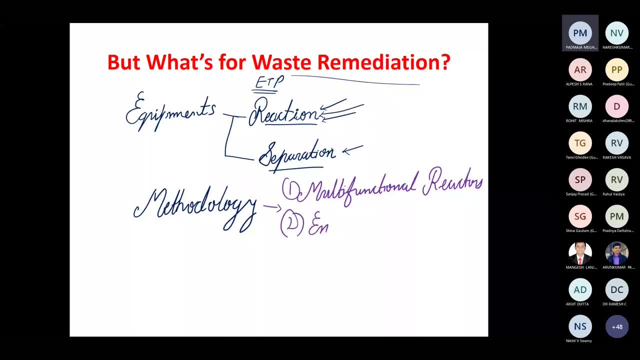 Like, if you are having that particular chemical reaction, how do you supply heat of reaction to it? so not even just a sound waves also create lots of energy, And the sound energy can be effectively implemented in order to reduce that barrier. for you know, 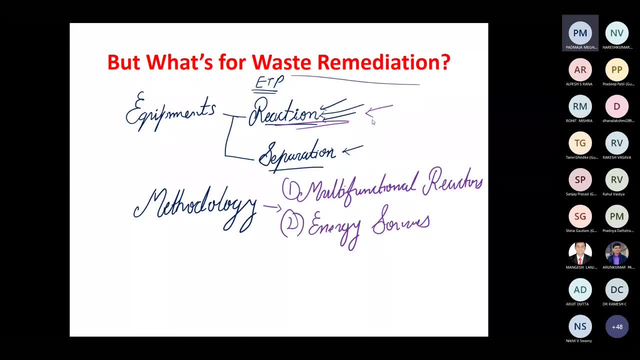 a reduction of energy. So we need to think about all these things. Yeah, reaction between your reactions in order to form desired product. so that concept is utilized in that sonochemical reactor. yeah, for example- just i'm giving you this example- sonochemical reactor, so that will take the energy from the sonication. 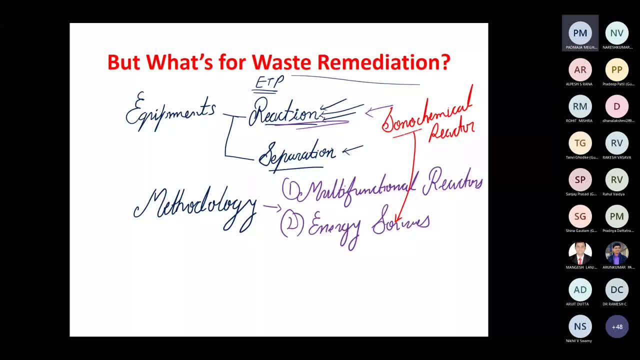 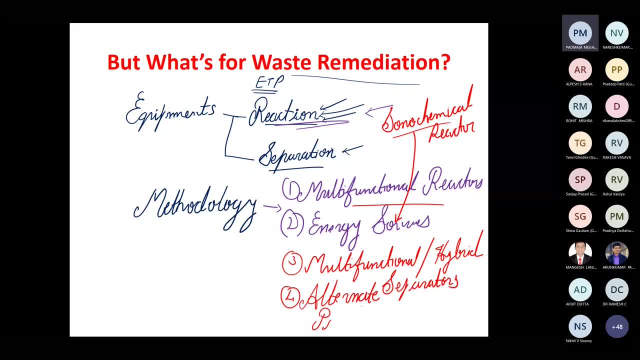 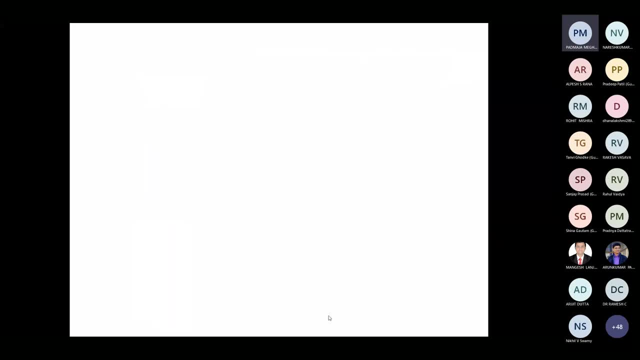 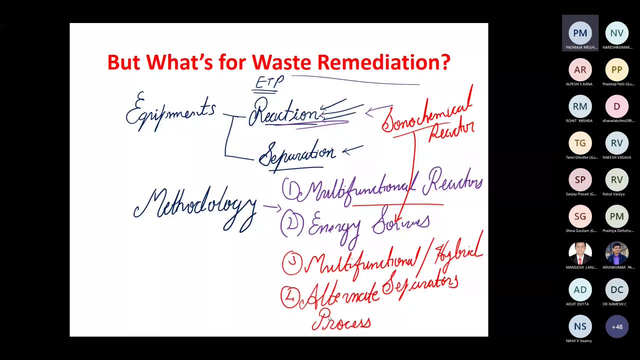 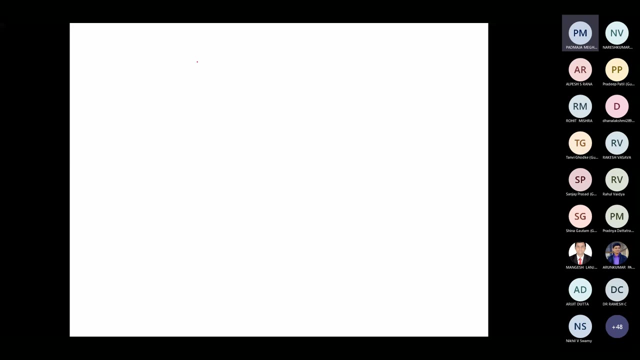 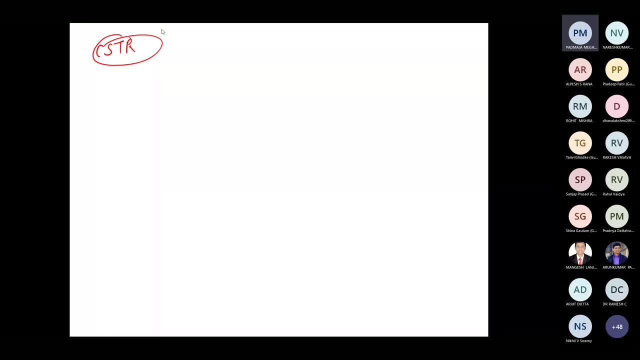 uh, then uh, can, or What needs to be done in order to get the string In conventional neutralizer. what happens? The mix, the strings get mixed in. some like just I'm going so all the strings get simply mixed and that's immediately then in intensified process. 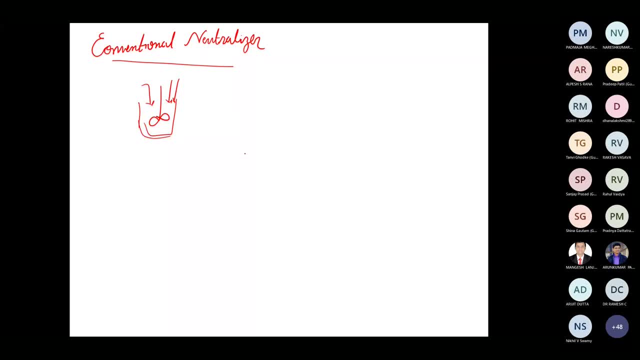 what makes it different from the rest of the thing is it is the type of the reaction. type of the reactor may be different. so, for example, that technology like eliminating the large size of reactor may also save lots of space, lots of capital investment, lots of. 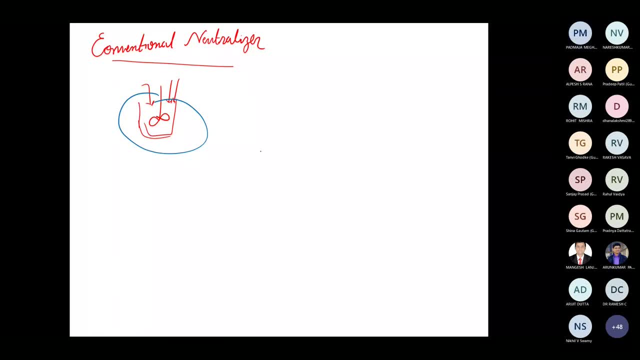 energy, and that's why micro technology, micro reactor technology- so the micro reactor as there are there, contains tiny size, accordingly, that micro channel which can be re-trafficated by some professional techniques as well as some conventional techniques, and so these will ultimately result in lots of benefits, and this benefits 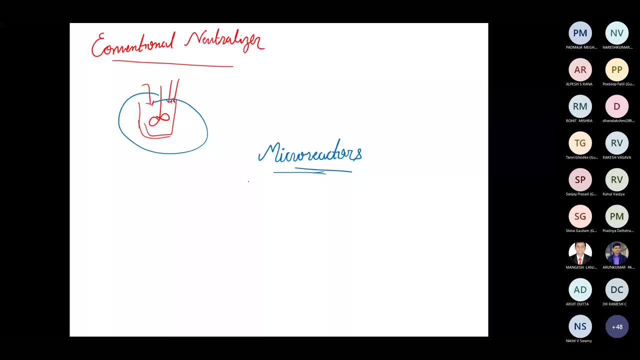 involves that overall volume of your reactions utilized means overall volume of additives or the intermediate used during the process is very late and the activity is the very important in your here: the activity and accordingly that yield of your final and further considering all these things. see if you are using the micro. 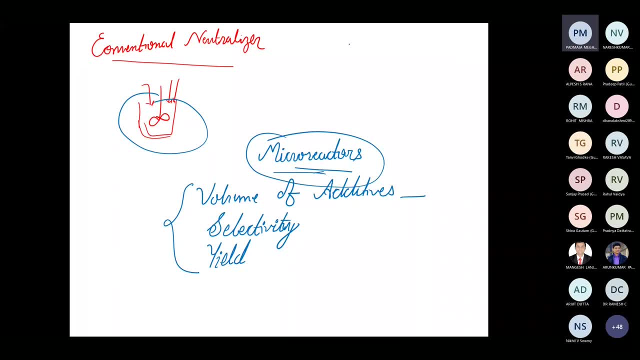 reactor in your ETP and your ETP flow rate is, let's say, for example, your flow. your liquid is generated, liquid effluent generated. suppose 5 meter cube per hour time. this is your flow rate. can it be cope up with? can your micro reactor cope up with this flow rate? 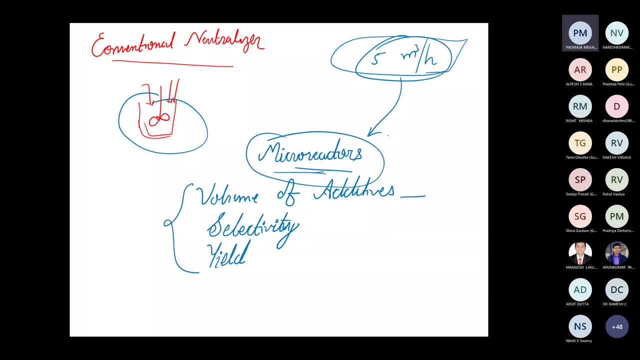 what would be the size of the micro reactor if it is containing some channels? micro channels size may be varying from few micrometers, so some hundreds of micrometer. and how can it facilitate this match? high throughput of the effluent strength in that case. so that's why 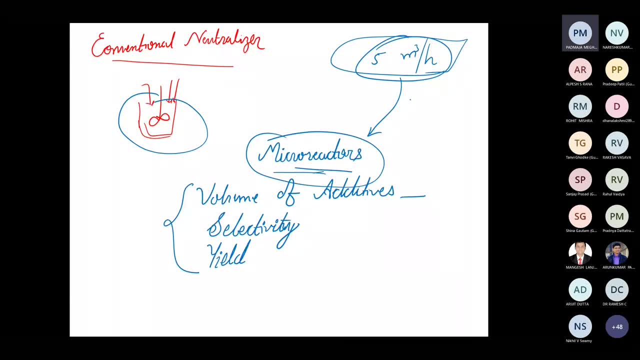 we must check for reliability, reliability of your final choosing micro reactor. how can it be integrated with similar kind of other micro reactors, and all can be processed parallel fashion, which can facilitate your handling of 5 meter cube per hour or any other higher flow rate. so that is. 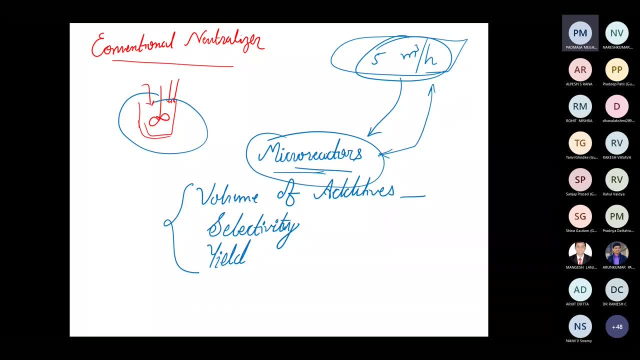 a big challenge in the, especially in the case of the micro reactor, so that decreased in this effluent density and decreased in the concentration accordingly, your chemical usage in treatment of that stream will be different and hence that micro reactor option, whether it is advisable to use or not, that can be. 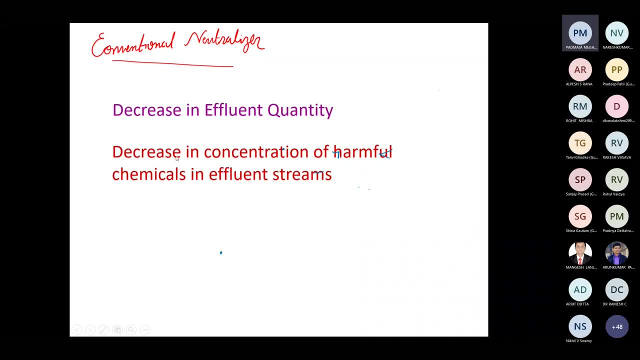 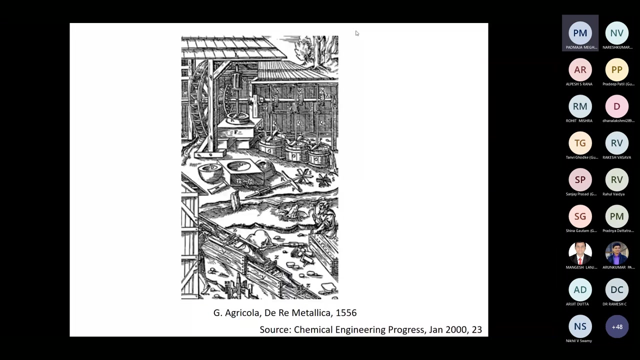 identified. so we have to consider the processes of micro reactor, especially the in the carbon footprint. so This is a very old technique for recovering gold from gold ore, where all these gears are made up of some wood materials and these are the shafts connected with this gear mechanism. 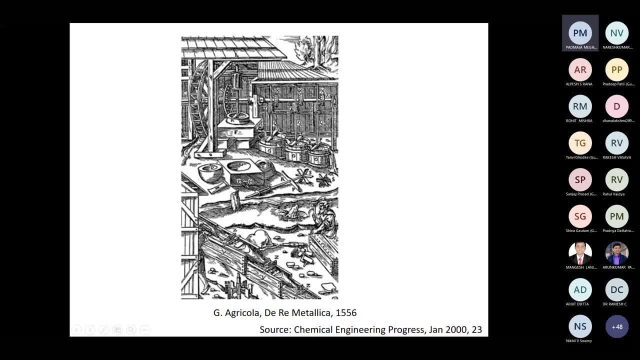 and on the far end it contains some educator blade. they are residing or simply supported by the periphery of this theater and hence these are series of cases: one, two and three, and uh afterwards on. all this is actually a torrent. ultimately, you can go to this finally. 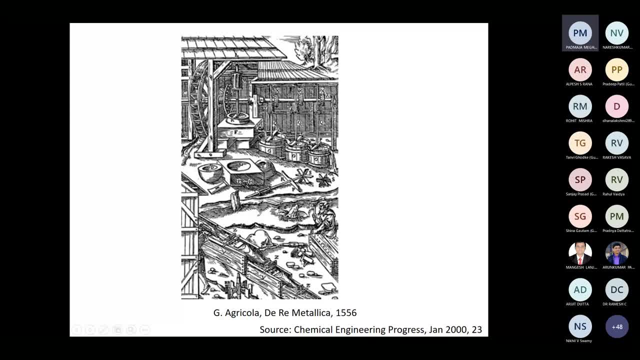 cardboard material and, let's say, protection. so this is the traditional process, uh, and lots of things need to be done still further, even though there are lots of advancement has been available in this technique, which will give us some idea regarding how can you implement your media, like what media appropriate thing in order to achieve that thing. 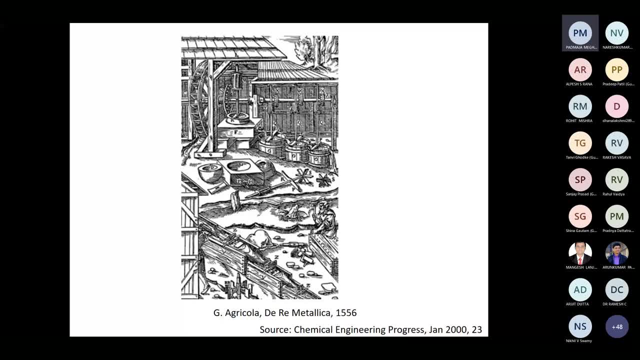 so, so what will be the investment over here in this case? uh, if you simply see, like, uh, uh, what can be done? so far, we have discussed a lot of things for general purpose: intensification. so, just before taking this example, how can you? what are things that can be reduced? 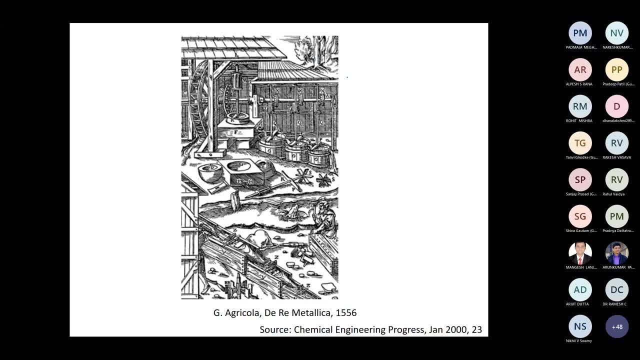 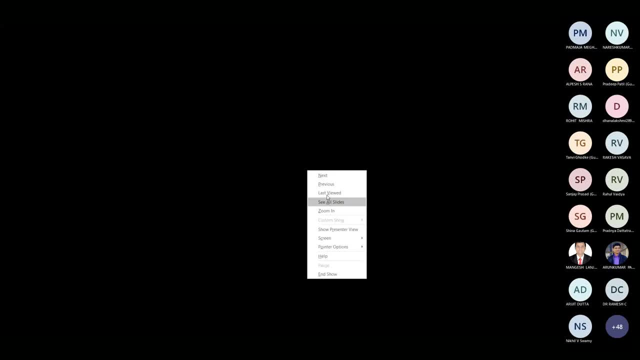 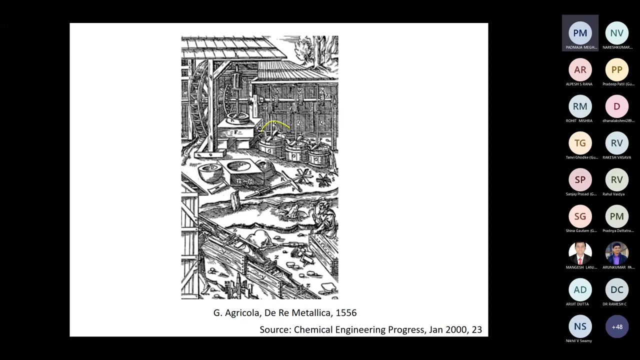 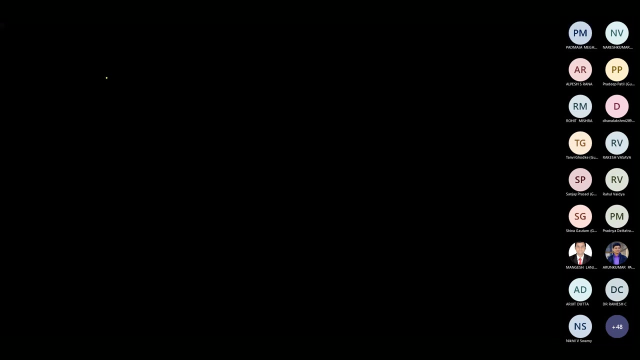 process, uh, you using concept, the process intensification, uh. so so see, uh, if you, if you here, it's what? what are the things that can be replaced or that is already replaced, already replaced by somebody else before us, educators, this peer mechanism. So in what area we can try over here so we can reduce, so that we ultimately result in? 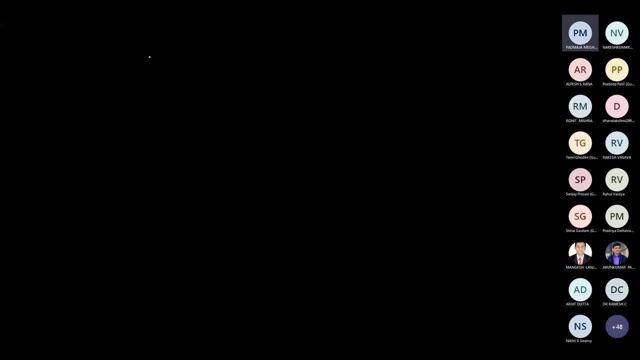 this decrease of overall investment is is and time. raw materials, energy means inventory, also Also energy. So we can reduce the cost of our investment. So we can reduce the cost of our investment. So we can reduce the cost of our investment. 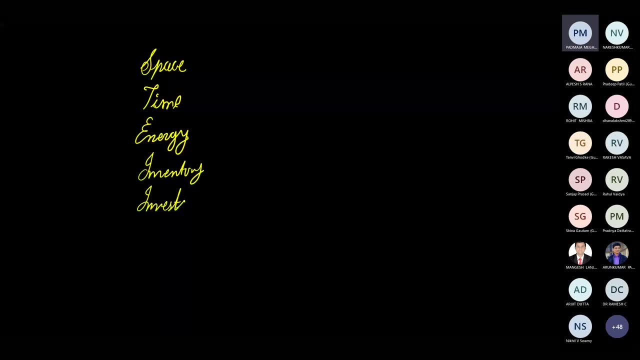 All these things get reduced if you provide, if you put some effort considering the concepts, what I, what we just now discussed, And, accordingly, accordingly, what will be the result? the ultimate result will be: What is the overall result? That overall production rate will be much more, and even the quality of your final product. 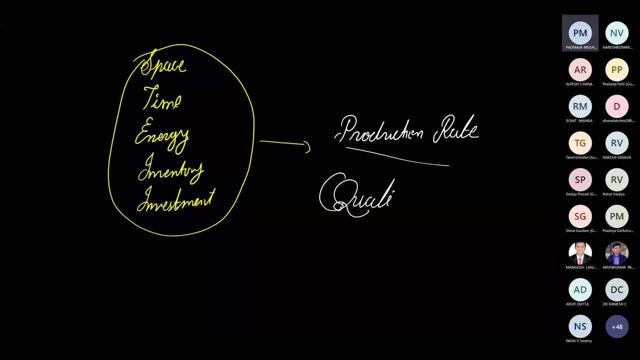 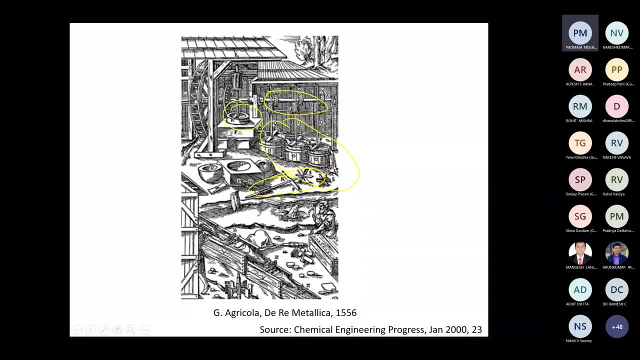 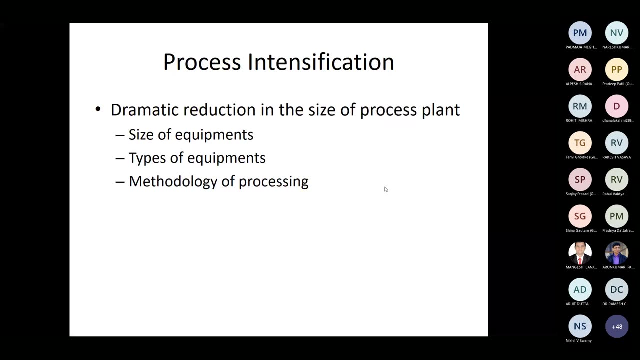 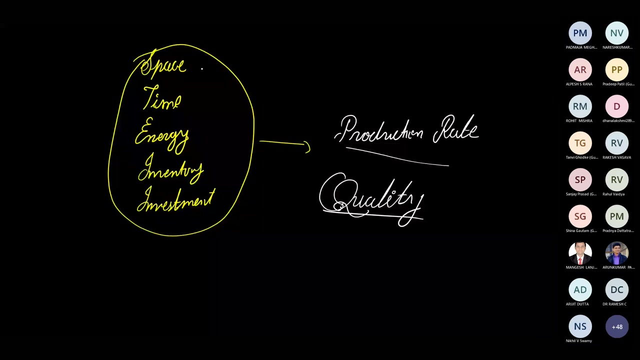 will be much more. In this particular example, the overall concentration of your final product will be much more And, at the same time, this energy will also increase. Okay, That's huge. So, ultimately, in order to achieve all these things, the reduction in all these parameters, 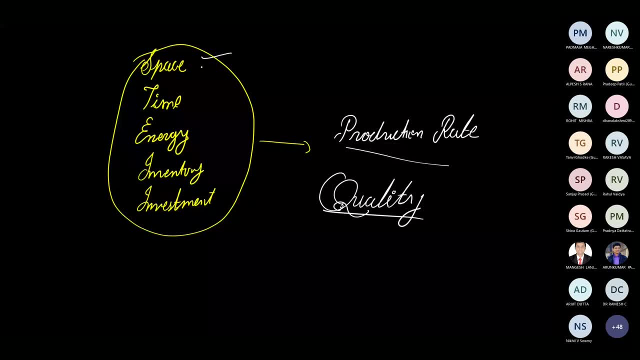 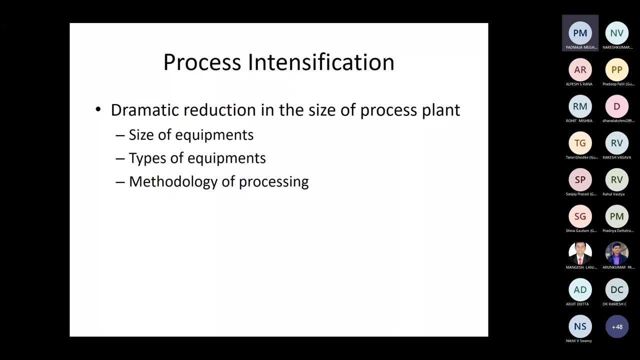 reduction in all this space, time, energy inventory, investment- what we need to do now. So we need to work out on the size of this equipment, type of defense industry heat considers and methodology of processing steps, And then we will reconfigure it in order to have 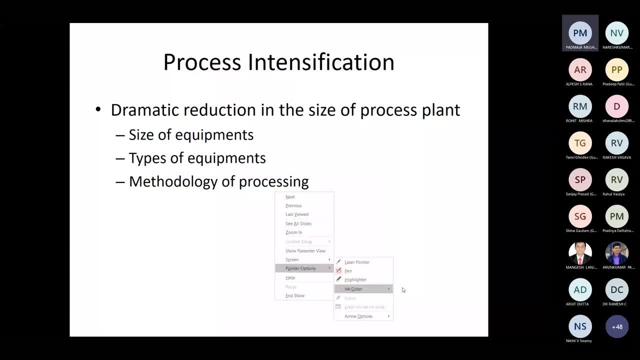 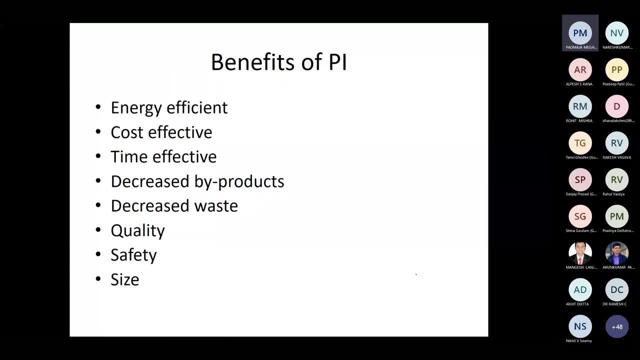 So, as we discussed this energy efficient operation, most part protective time, protective operation, And we will have to make these, these steps as value of your overall processing staff. processing units results in the decreased byproducts while performing to that sustainability. So is it a sustainable solution if the byproducts is reduced, byproducts quantity is decreased. 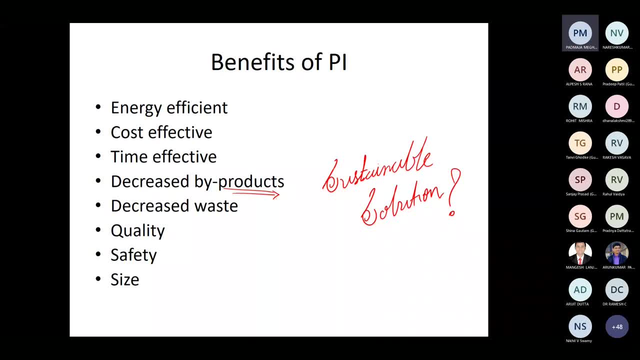 will it give a sustainable substitute? How do you rate this item? So, when we talk about the sustainable, at that time we need to bother about the overall environmental impact, as well as the market availability of your final product, its composition and, if the byproducts are formed, and what are the alternate routes in order to discard. 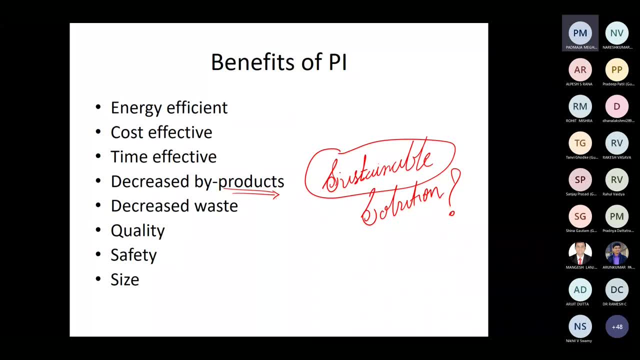 from the plant site or reuse in its own plant or somewhere, how to market that product, for example, or is there anything required in order to evaluate to that particular byproduct according to the distribution of waste? that will also ultimately result in that loss of production and you can have easy or more safer and the desired goal will be achieved. 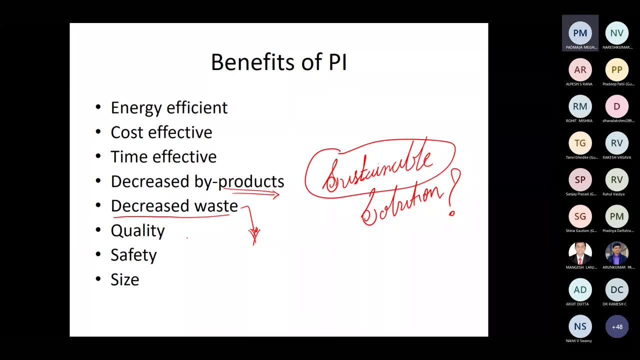 by this, Yes, Okay. So what is the quality of your treated water and the cost of extra effort used in the design stage? only So this extra effort during the design stage that will only result in the final quality of the treated waste. 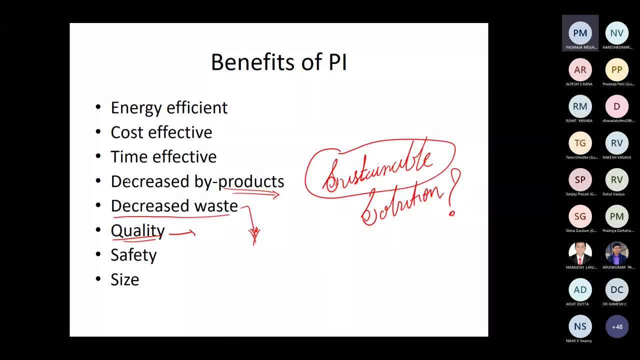 So the prior treatment is again, it's less. how much the matter is going to be So according to the overall size of your treated appliance. we also that and the sample is not down. Okay, So I need to filter it and then we can process. 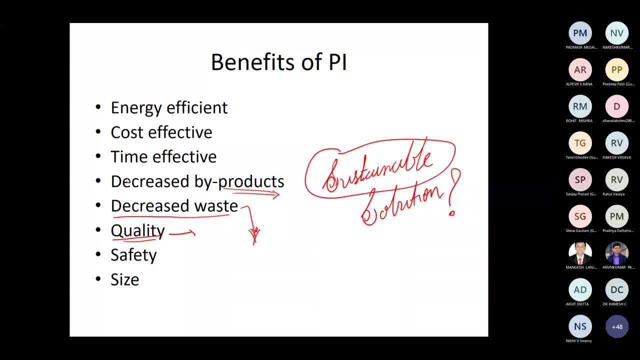 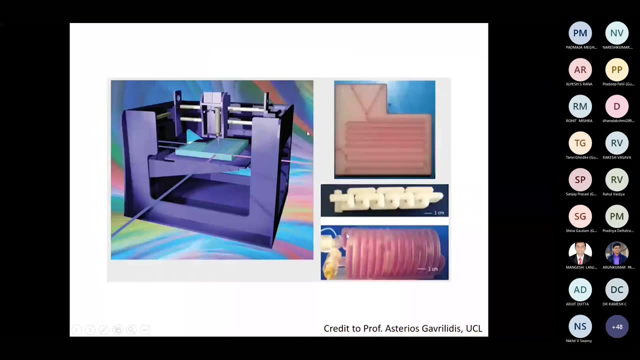 Okay, effluent will also drastically reduce and overall COD, COD- all these parameters can be eliminated as described by that local carbon property, and hence it's just, for example, like if you use this kind of things, like if you want to use some this kind of micro reactor. 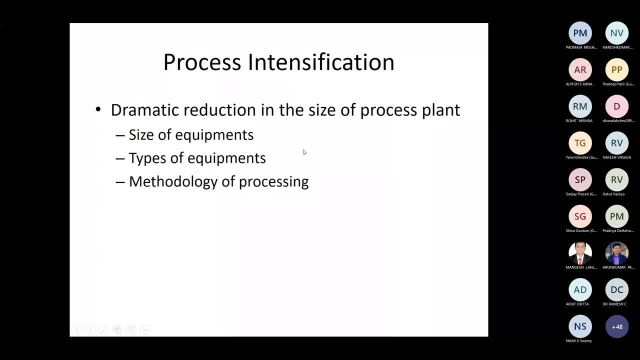 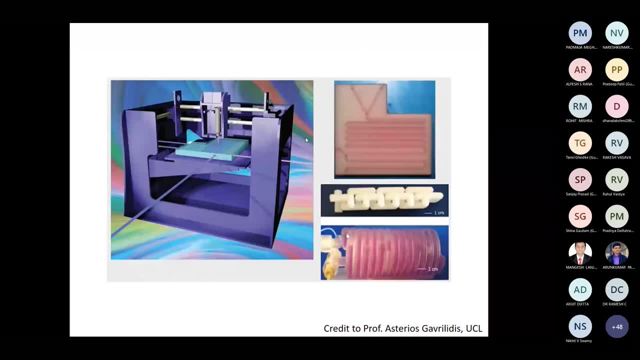 uh, this minor reactor ultimately incorporates some of micro groups for those tiny volumetric elements which have a reaction channel, and there are different techniques available through which we can navigate these micro channels, like here. it is like you can use it like 3d printing, which will result in simple, which takes on both simple steps. 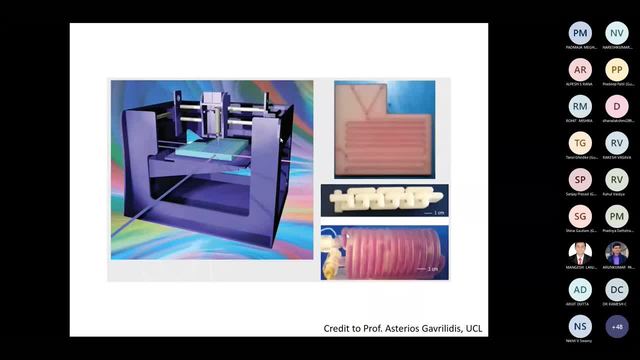 like trying all that right generation. you know some appropriate software and then your 3d printer will bring that object in the way based on the command you went to it, and you can have this uh tiny reactor or micro reactor available. so uh, materials as well as machines are available right now, which will help you. 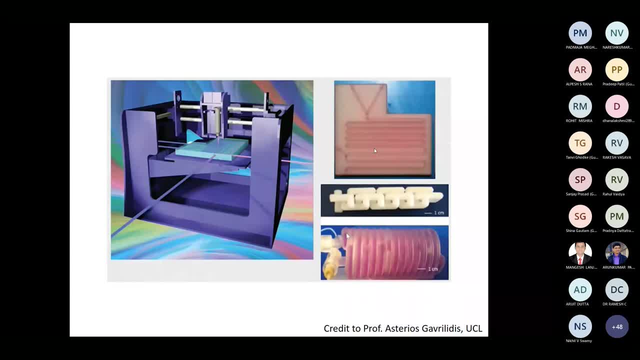 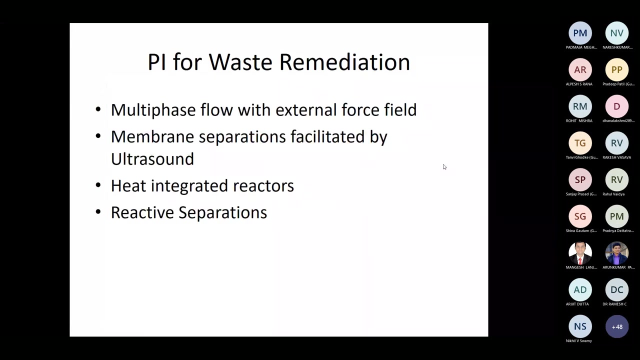 lots of flexibility for change over to the things and and also the penetration of some properties of the strings as well. so ultimately, the multiphase flow uh with the external force field. if your effluent treatment stream contains some metallic elements which can be applied, for example, cultural weights, also 잠깐만. 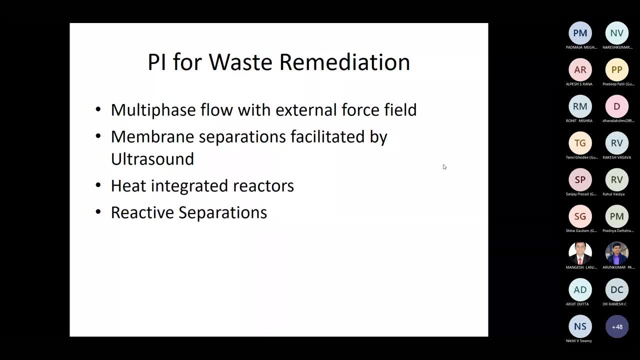 with the actual magnetic field, is that can be really removed or separated if the magnetic field is provided enough, just for example, and the membrane suppression operation, if they are assisted, assisted by ult абсолютère, if they are assisted by ultrasound, or if there are some reactors which can be heat-inflated. 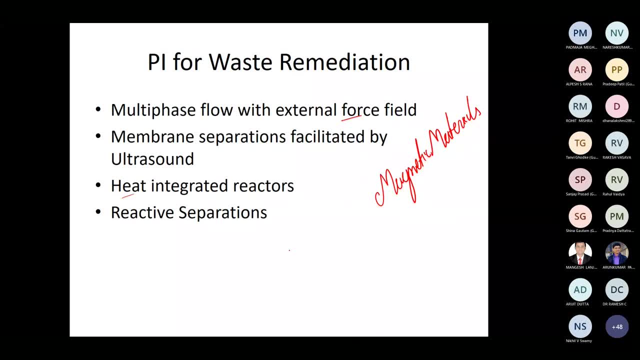 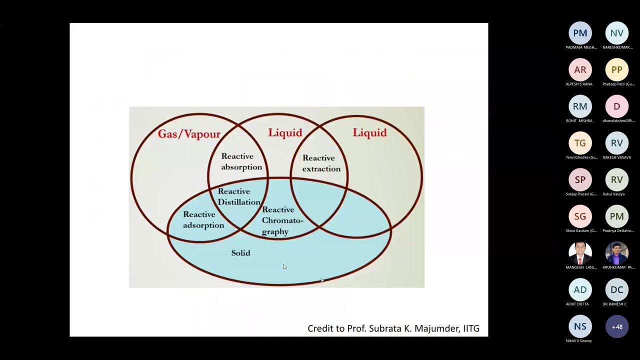 or some microwave reactors, can also facilitate that. This one equation, facilitated by this membrane separation operation, that is also a good option, one of the good options, and has reactive coefficients in which your reaction and separation occurs simultaneously. So these are the main things you can consider, especially for this remediation, and which 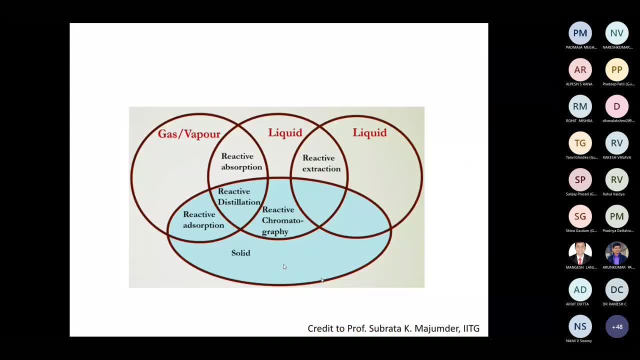 we will discuss later, Thank you. streams which are coming to the effluent treatment plant from the chemical process, which can be divided into pure liquids And again this liquid in turn can be classified as organic liquid, aqueous liquid stream. And this is your multiphase flow, where your 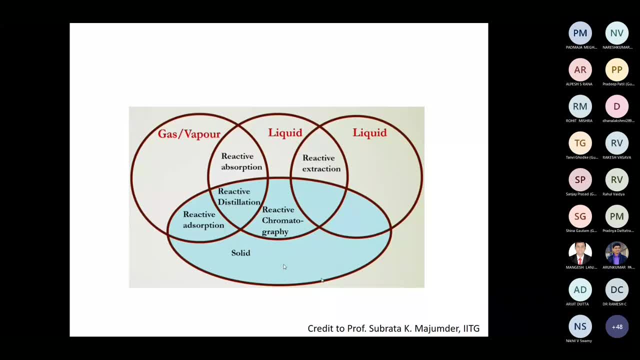 gas and vapor bubbles may be associated with your liquid stream. Sometimes even direct gas or vapor can be connected with the flat system through which it is on plant site. So absorption need to be reconsidered. what kind of proper contact mechanism? what is the driving? 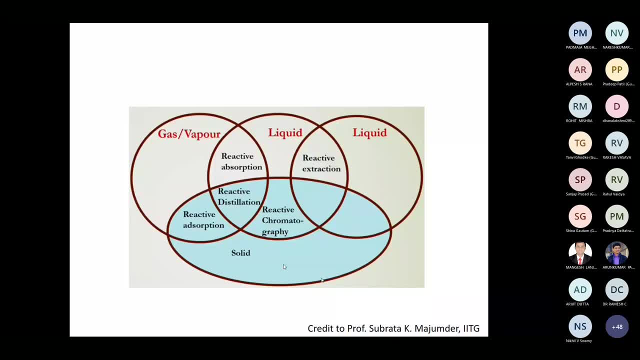 force in this gas-liquid operation? is it the chemical reaction? is it chemical absorption of gas by means of chemical action? is there any way in which we can use that reaction resistance or diffusion resistance accordingly? if it is a liquid-liquid extraction, then is 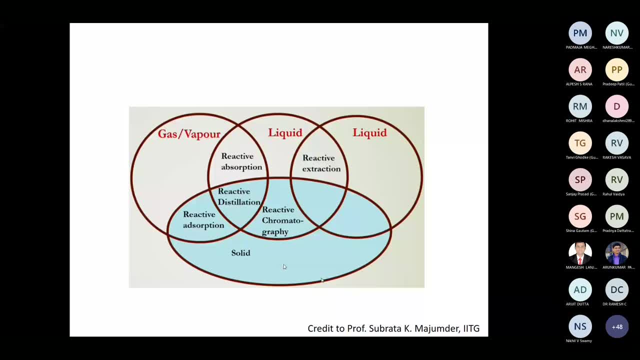 it associated with chemical reaction. do we have another solvents which can more preferably dissolve one of the constituents from the other liquid stream and accordingly reactive distillation. So we have the distillation as well as the reaction occur simultaneously and as soon. 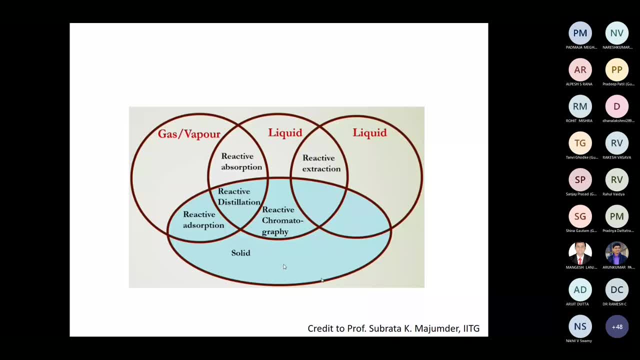 as the product forms the form product, so the byproduct can be simultaneously separated from that zone. so that is reactive distillation. similarly the reactive absorption. you need to come to the reaction, the absorption takes place simultaneously, and reactive chromatography. 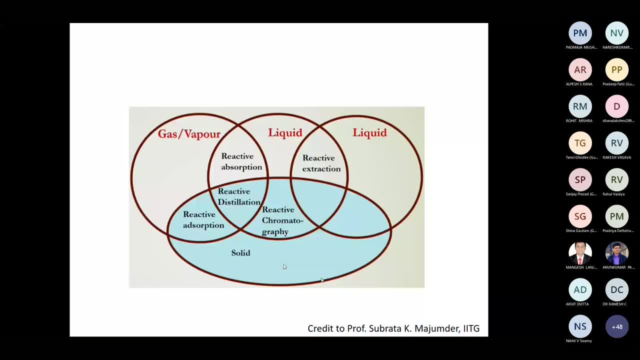 takes place simultaneously and the byproduct takes place simultaneously, So these are two ways as well. there is some sort of multi-phase phenomena are very often very common and we need to look at that thing in order to achieve these basic things which. 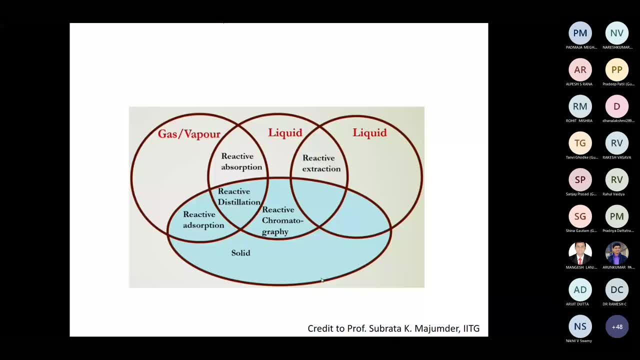 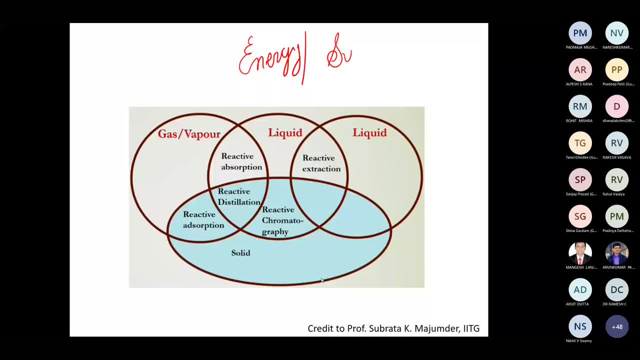 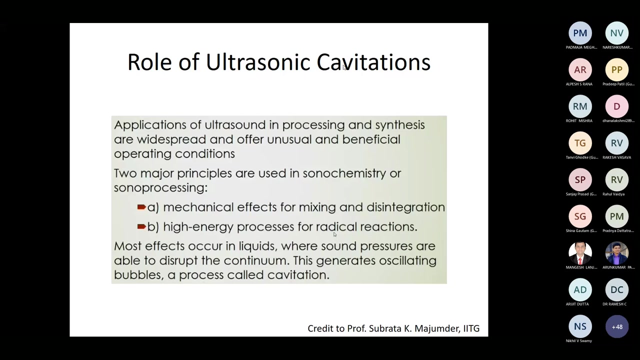 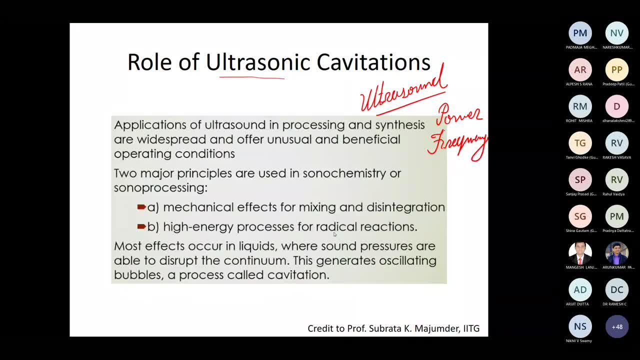 So we need to combine these different appropriate parameters for your ultrasound and also ultrasound may be at point source. you can provide this ultrasound by point source in which your ultrasonic probe. ultrasonic probe will provide will generate the ultrasonic waves at its tips. 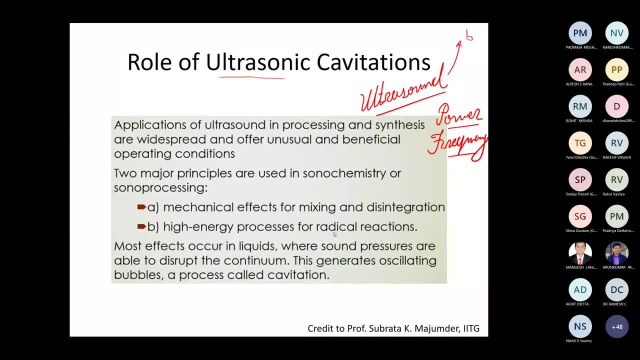 and that will give your ultrasound. So we need to think about all these points. So we need to think about all these points. So we need to think about all of these points as we are looking at this ultrasound. so email customer statement for each of these points. 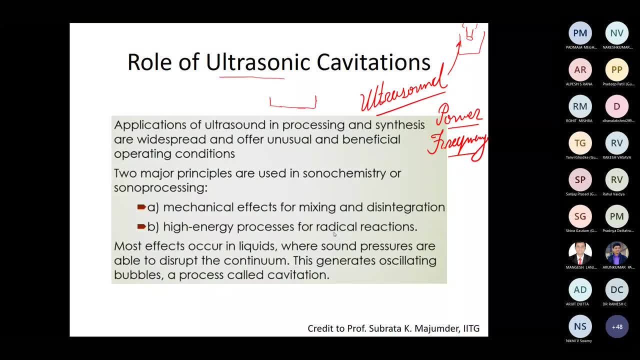 Also, if you got 얼마나 of data, Where do I get all these points? Okay, so I have 10? And that formula is pretending to know for you that I also get. I know, I know, I know that it's not so big a deal, but how they know how much time left? 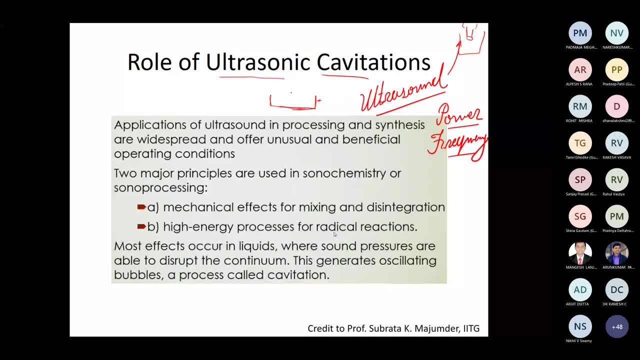 down with you, you might. Yes, that's right. So there are two things: bath and ultrasonic horn. ultrasonic horn or ultrasonic bath. These two things are available Currently. they are also utilized in chemical industries, as well as in pharmaceutical industries. 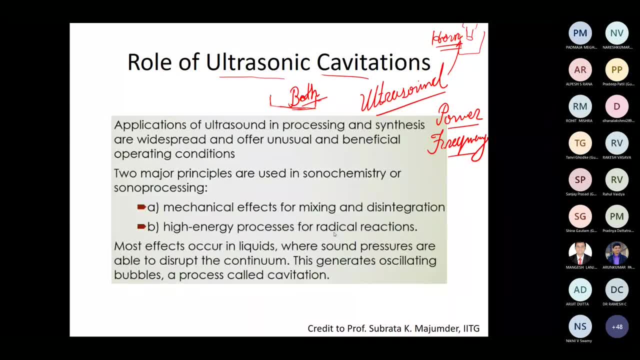 in order to provide that ultrasonic cavitation to that reactive media, in order to facilitate that chemical reaction using the sonar chemistry principles. So the mechanical effects of mixing and dissipation can be easily killed in that case and high energy processes for reactions as well. 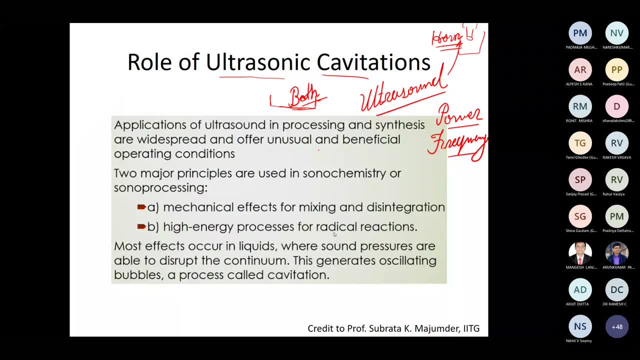 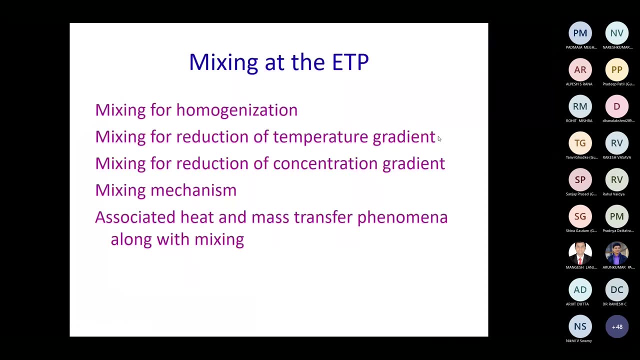 So easily facilitated by means of this kind of horn, where in the near vicinity of this zone? So there are lots of effects. So, and what is the need? Why do we need to look at certain factors in order to achieve or in order to view that? 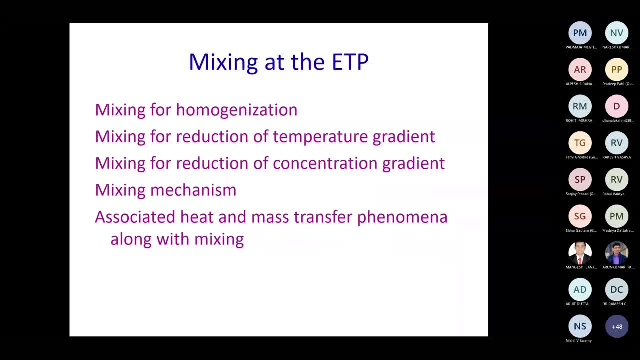 mixing tendency of the liquid. That is also important And these are the factors. So what you can see here, What you can see on your screen now, like how can we implement this entire mixing process or why do we bother about mixing for certain treatment purposes and steps? 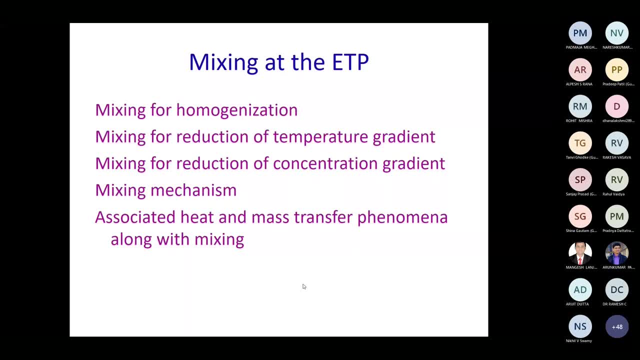 So most often we need to homogenize that entire effluent streams which are coming from deep streams, the parts of the earth or the plants, and if we are having a stream that is having throughout the same temperature concentration of the species, then the overall 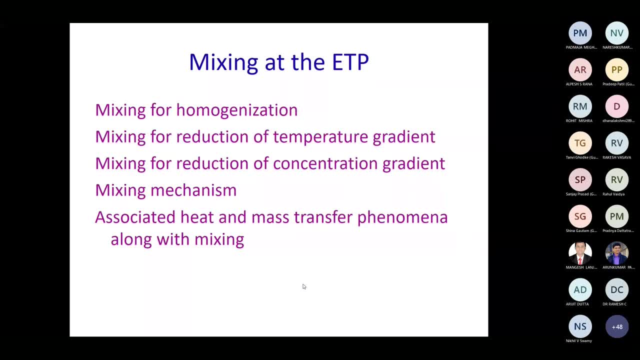 loading or the overall effort. The required at that effluent step can be easily designed or can. they can be easily looked at, can be easily addressed if something went wrong. if something goes wrong, especially in case of heat transfer and mass transfer controlled, 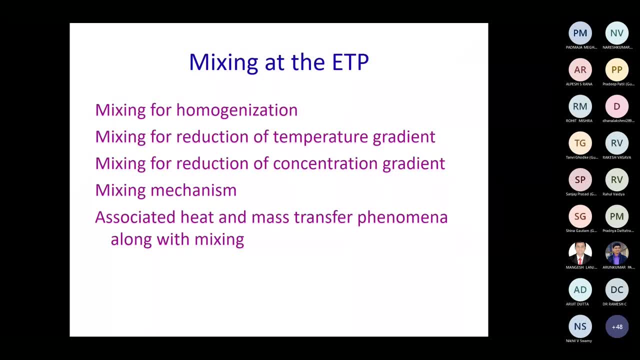 So okay. So here are the items that we can look at. So what I want to do here is to give you a quick overview of the methods that we are using in our application, So we can look at the first method. what we are using, what we are looking at, is the. 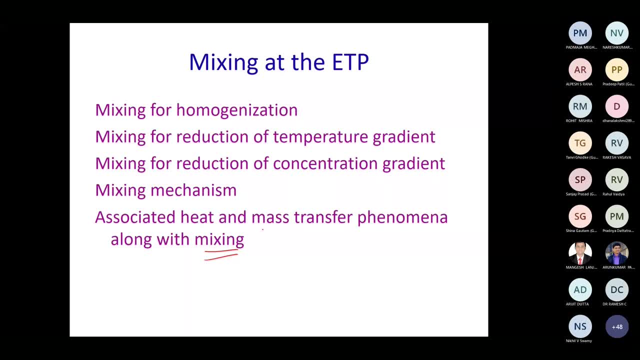 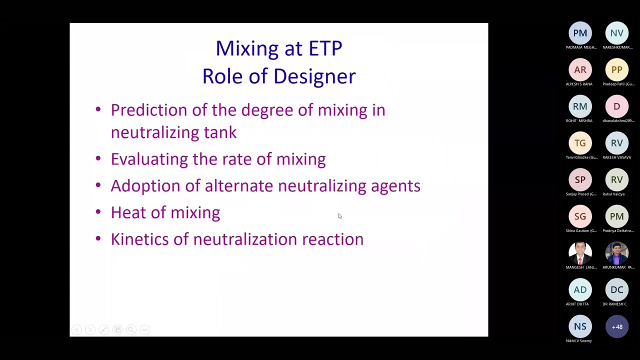 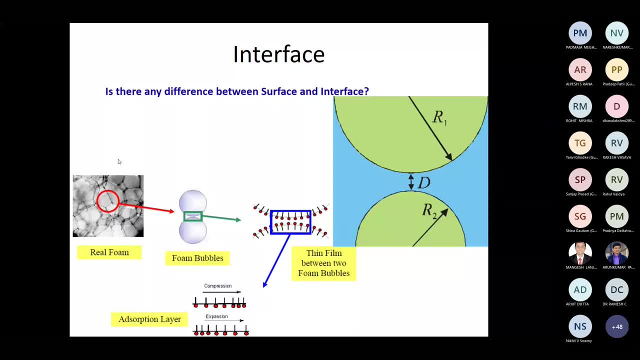 affluent treatment plant how to break the foam easily. so deforming agents need to be utilized, and that deforming agent means, if you know the intrinsic phenomena, how this liquid bridge is going to get destroyed by the action of the attractive force of these two droplets. if these two droplets competition is very high in comparison with the overall strength of this. 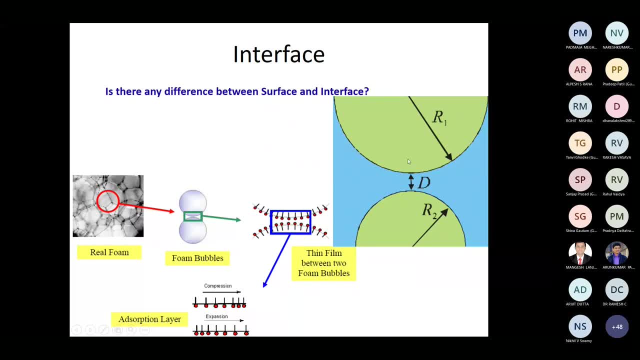 liquid bridge, it will get wet and both the liquid colors, which is other, and they will merge each other with each other and hence we can have that you because droplets- and ultimately we can have the phase separation, and this phenomena may ultimately lead to the separation of. 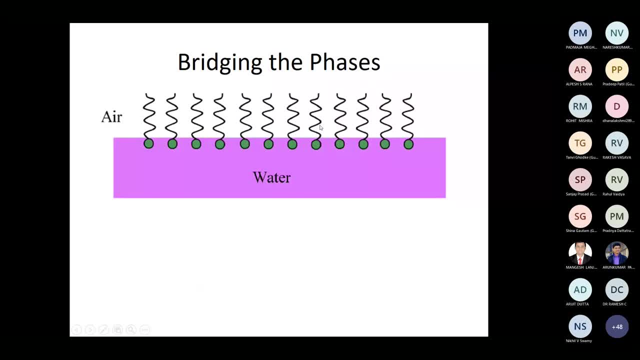 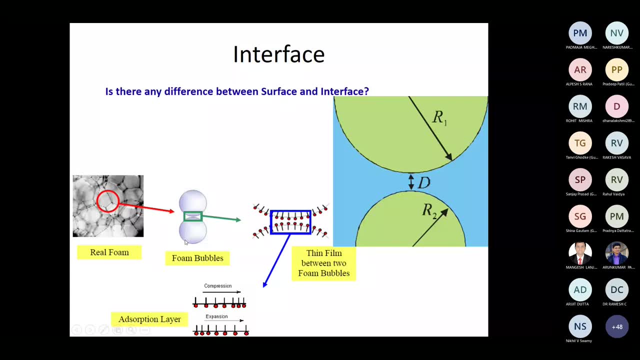 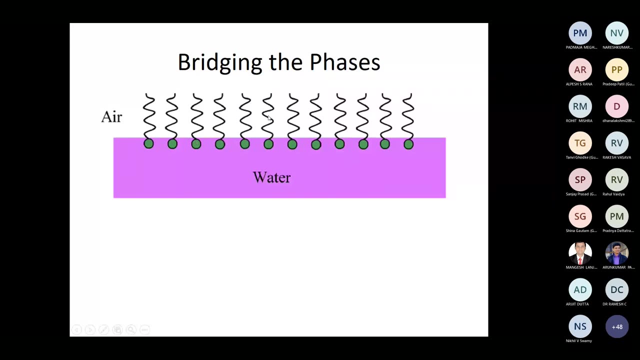 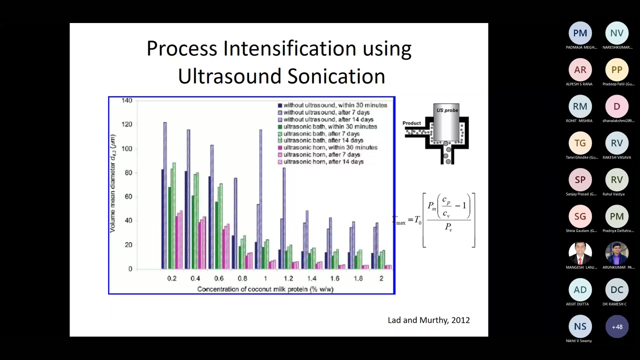 elimination or reduction degrees of this formation, of growth or the form. so some perfect active agents are useful for elimination, for altering the service, intrafacial transfer, and that's why you can achieve that transformation and ultimately we can have the phase separation and this phenomenon operation. so, uh, we, in our experiment, we used some uh ultrasound for our separation operation. 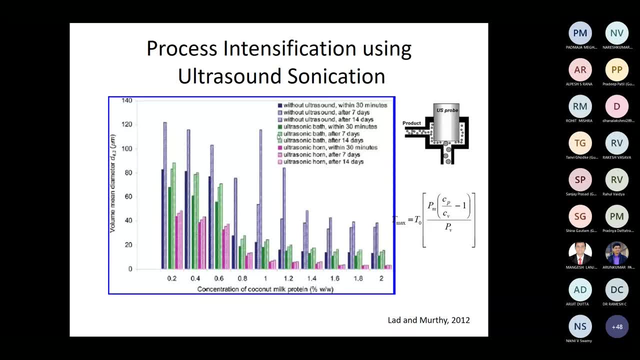 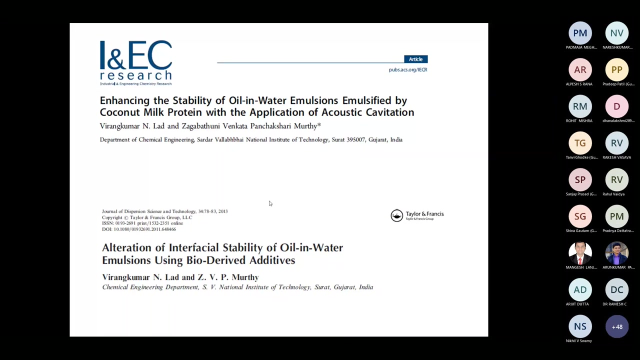 and we found that uh, what is the most appropriate uh processing parameter for ultrasound uh which will result in uh appropriate formation of that uniform size droplet in our sample to to produce at the time the 91, 9, and we found that it Uhm did not. 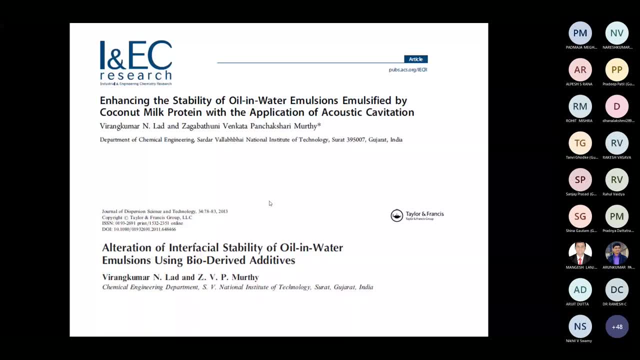 produce quite as good as the another uh sample for golden border transfer. but so, and especially at the time we worked with agriculture, we'll forget the idea about the points cars arehol sampling factor shop in the formula gold sample in a diagram. this is so kind of uh. it has this very sort of conventional nomenclature. there's important involved in our from pieces, but over all I first einmal use ultrasonic probe and then we use the ultra නrière and then we use the ultrasonic probe as well as a stress and also ultrasound vessel, ultrasonic back as well as ultrasonic probe. data quoting: that was Ε 400 feet. as helped that ultrasonic probe was very much effective, uh, even had to comparatively ininseed power. i was able to produce a, consulted by ben, convinced feel. 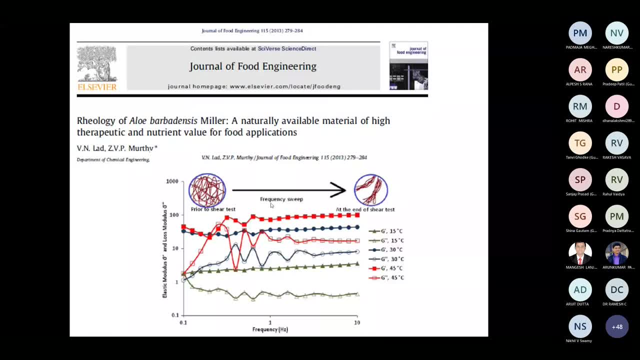 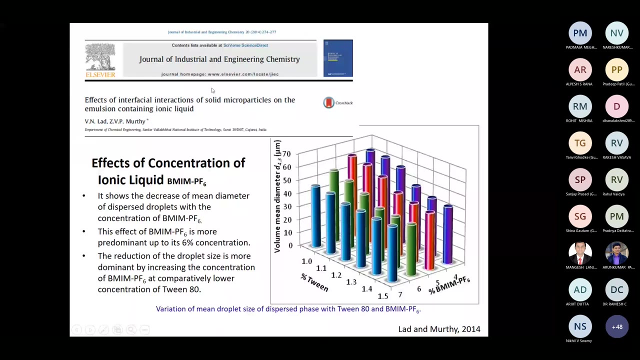 And here in this work we utilize some natural material in order to have that full evasions, where intensification has been done by means of some sort of rheological modification, And this is the case where we utilize some interfacial interaction in order to facilitate 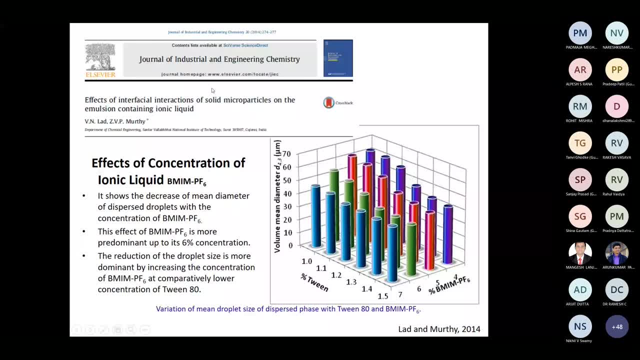 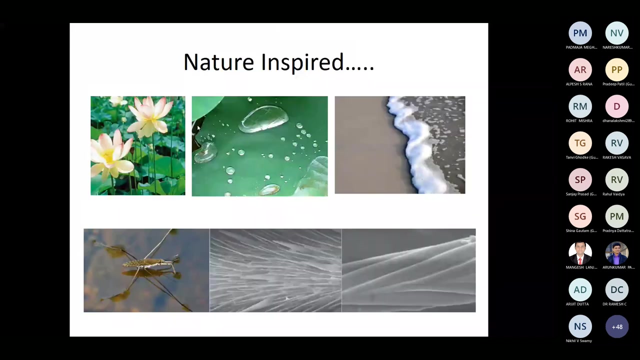 that intensified process for emulsification which can easily get stabilized at its own using some extra additives, And the extra additives used was that ionic liquid. So these kinds of additives can also ultimately result in some. So most of our research is nature-inspired, especially in the field of interfacial engineering. 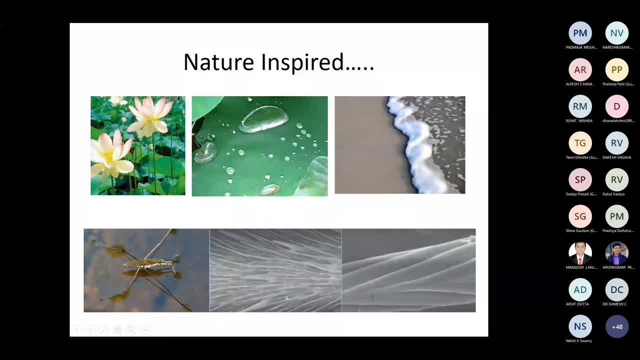 where there is a lot of super-hydrophobic surfaces, which are of relative importance. How to create the super-hydrophobic surfaces, how to eliminate this form, especially in these effluent treatment plants, or even in effluent treatment plants? 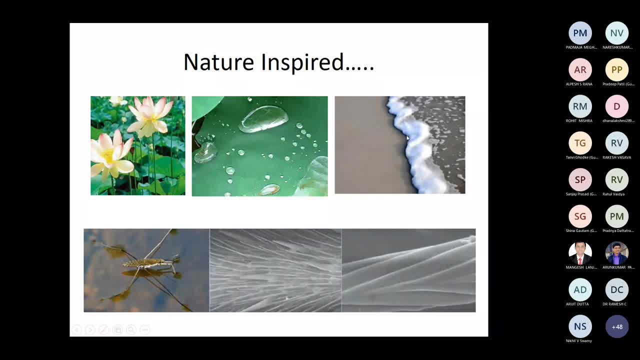 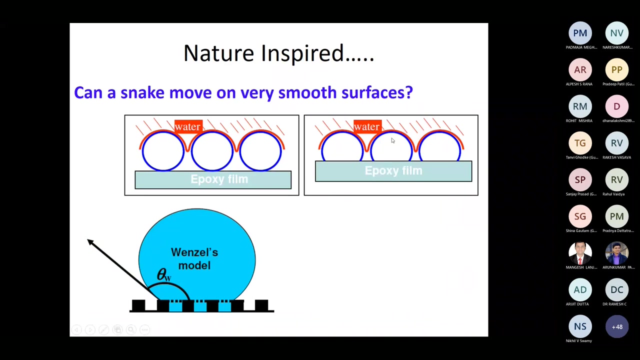 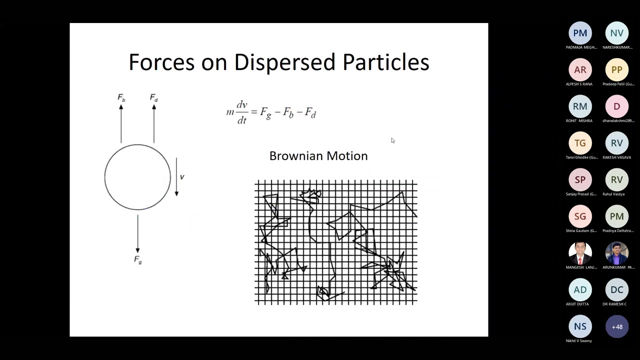 how to eliminate this form formation in some radios. So lots of interfacial phenomena is involved here. If we are able to identify that property, we can easily tune the surfaces and interfaces in order to achieve that required surface. So now, accordingly, this surface. 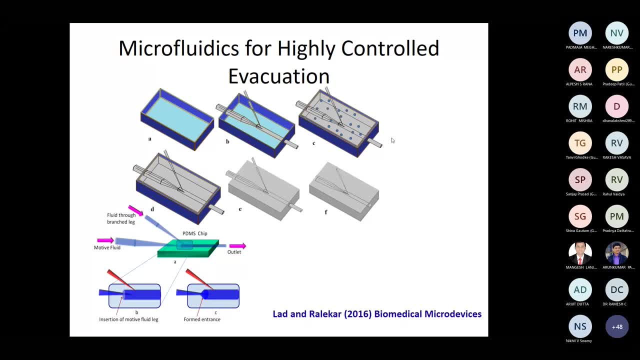 So, in order to achieve that micromixing in our device, we've replicated PDMS microchannels and this PDMS microchannel was a short-inert solvents- a short-inert one- And I've provided one deep-in solvents. this weld and mold was removed. 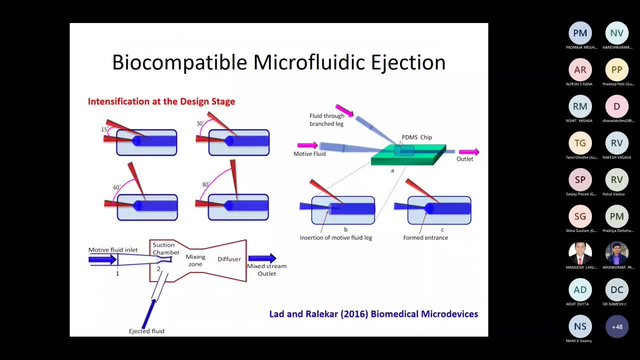 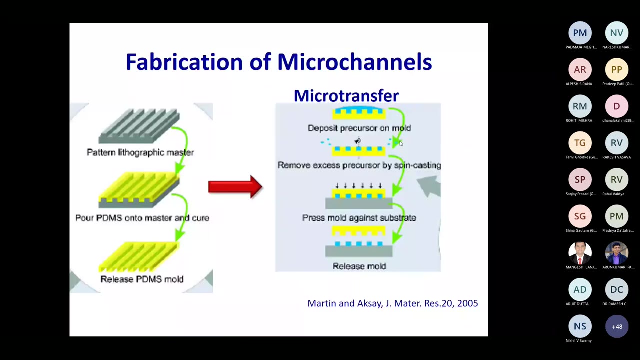 and this device was capable to produce a controlled vacuum. So if you want to evacuate certain space, it can be easily facilitated by using this kind of micro devices, which is just moving with the energy of the motif fluid only. No, any other extra energy is required, just the energy of the motif fluid. 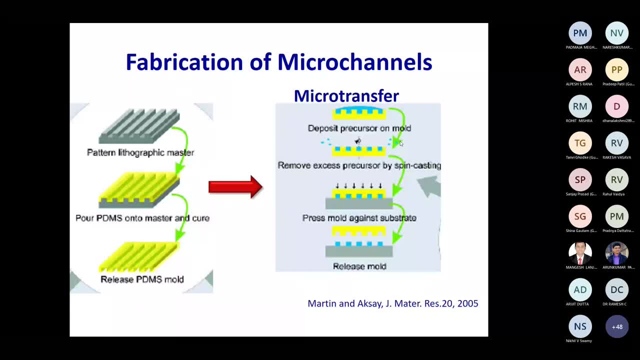 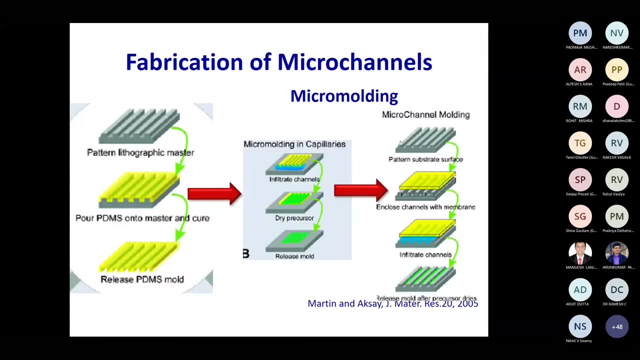 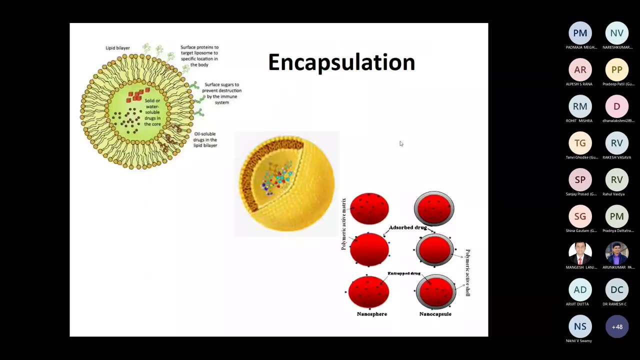 and the energy available in the motif fluid is utilized over here and the fabrication of microchannel is subsequent. Methodology is available. in writing. Currently you know this encapsulation of hazardous droplets by means of some biloves will also uncover. that also avoid that exposure to the environment. 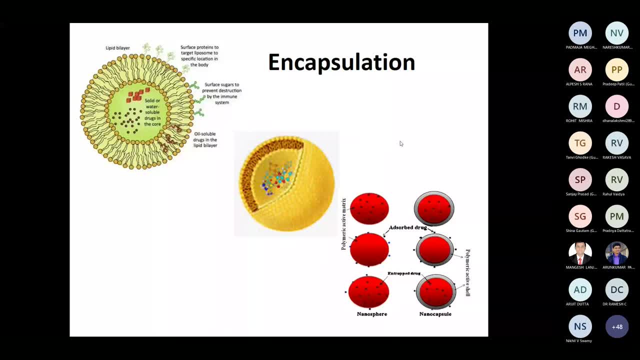 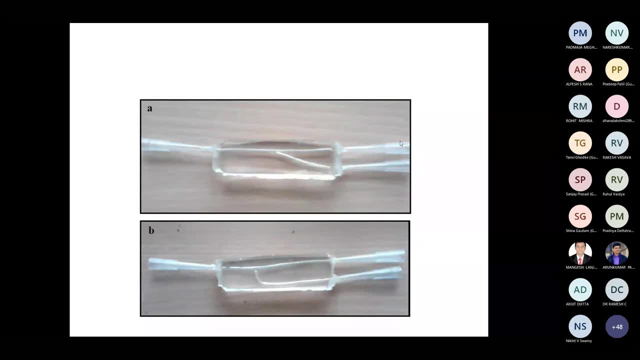 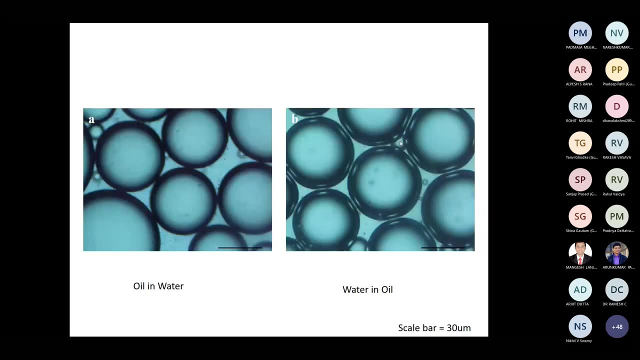 and that can be also utilized for appropriate drug delivery applications. And this is just a particular reference in the setup where we can now implement using some oil and water emulsions and droplets that are also generated using these oil and water emulsions. 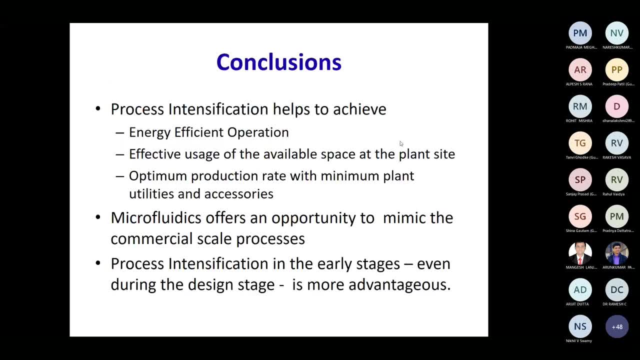 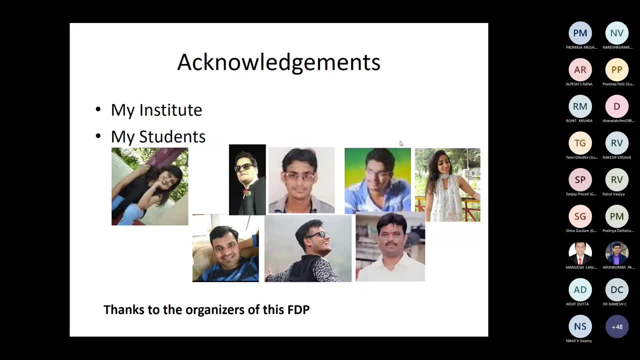 and this is my research group. Some of them have been just passed out. Clear has decreased And this biloves is one of them. So you know the THC is coming and it is indexing also. What is this degree is also the. 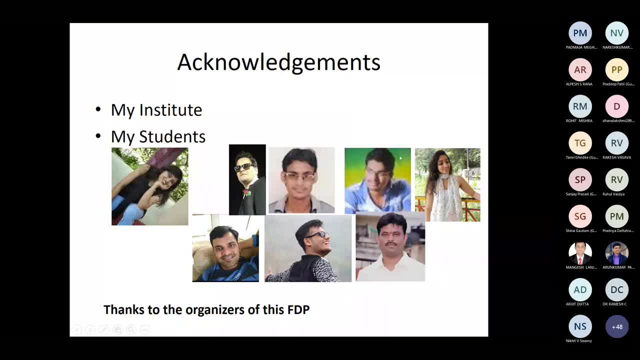 what is the THC degree that is used here? So, once again, thank you very much for listening to me. So I would like to thank my institute for providing the facility for research work, as well as my students, And once again, 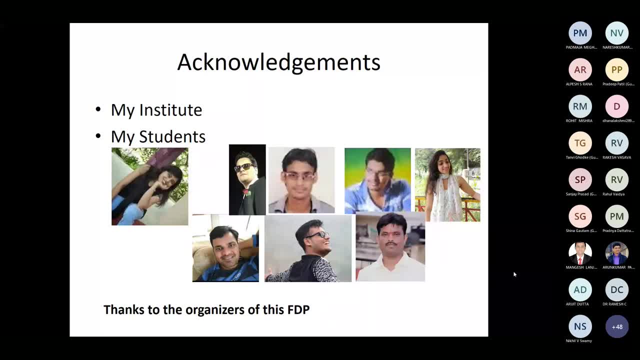 I thank you very much for the organizers for giving me this opportunity to express my views on this particular topic, So if you have any query or any questions, please feel free to contact me. Thank you, If you have any query or any questions,